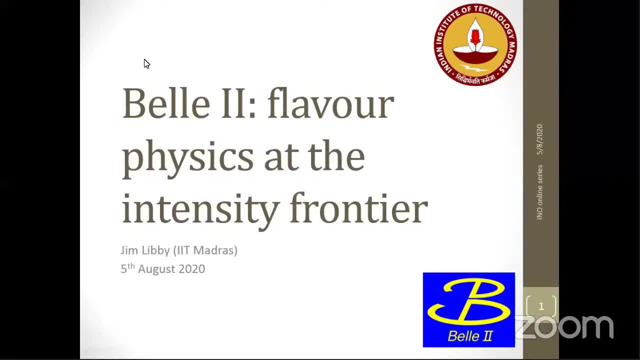 Thank you. Okay, So welcome to the series of online interactive lectures which have been organized in this by the I&O project, And today we are in the 15th week of these lectures, and today's talk is going to be delivered. 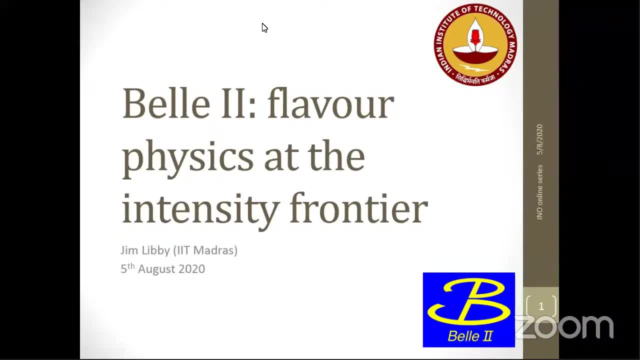 by Professor Jim Lippe. James Lippe, that is from IIT Madras and he is going to talk on the Bellet 2, Flavor Physics and more at the intensity frontier, Just couple of minutes on today's speaker. He is an experimental particle physicist. 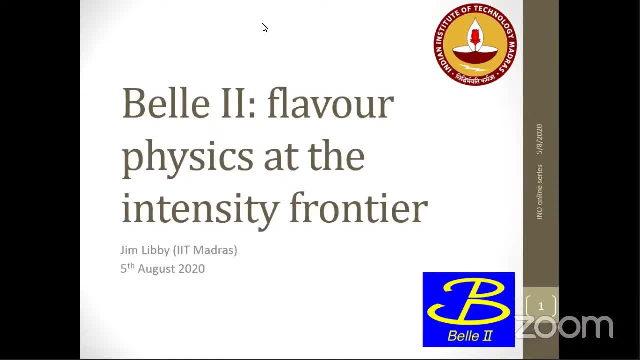 He is working at IIT Madras, as I said, since 2009,. Professor Lippe received his undergraduate and postgraduate degrees from the University of Oxford. His PhD work was largely based on the European Center for Particle Physics, that is, at CERN. 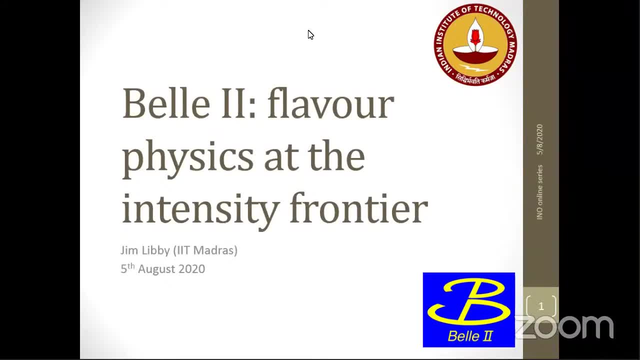 Geneva for working on electroweak measurements at LEP2.. Since completing his PhD in 1999, he has worked principally on Flavor Physics with accelerator experiments at CERN, Stanford, Cornell, KK, that is, Japan, and also high up in China. 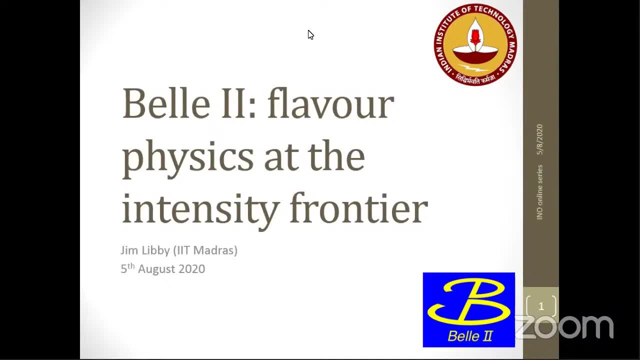 So that is his vast experience in Flavor Physics, and today we can look forward to a very exciting lecture from him on this topic pertaining to Bellet 2.. Yeah, So, Jim, over to you. Okay, Thank you, Satya, for both the introduction and also the invitation. 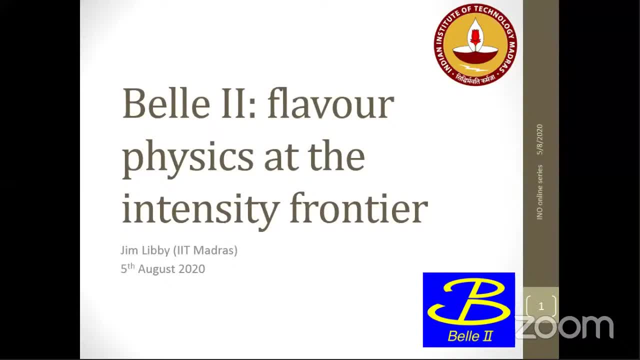 So I will be discussing the Bellet 2 project and Flavor Physics, and I should be clear from the beginning here I am talking quark flavor, not lepton flavor. So that means I'm going to do some sort of pedagogical introduction as well about why 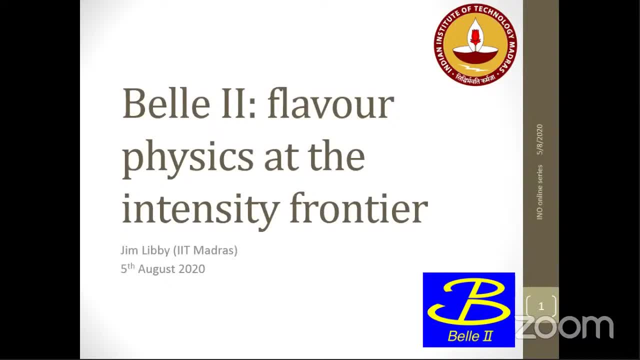 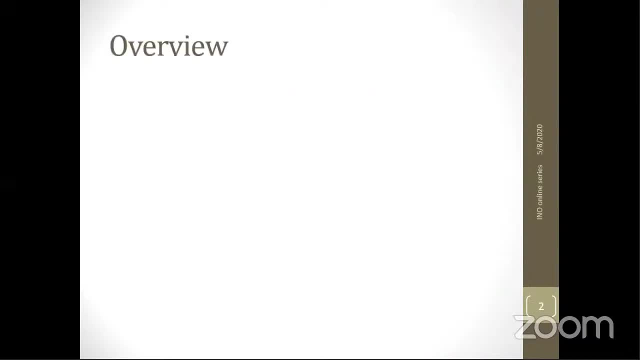 the quark sector is an interesting place in terms of particle physics and that's where the intensity frontier comes in. So for the overview of this talk, I will just introduce this idea of the intensity frontier first and what we're trying to address by such experiments as Bellet 2 that operate. 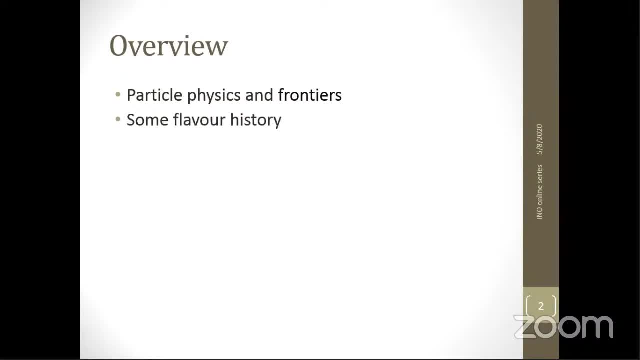 at the intensity frontier, And then I'll describe some history, which is quite appropriate for what we're trying to do. So give some examples- actually textbook examples- of things that we've learned from flavor measurements in the past, And then I'll talk about why we think this is a suitable place to look for new physics. 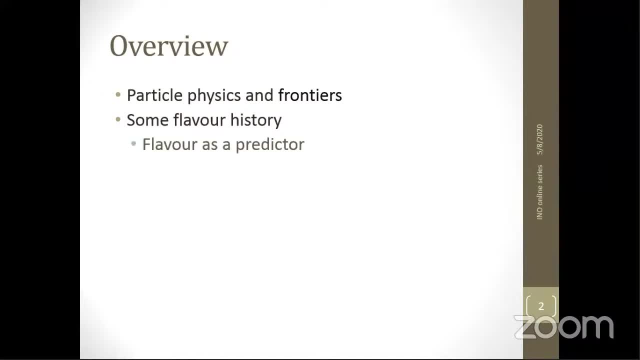 today. So essentially it is flavor as a predictor of higher mass scales than that of the beauty and charm quarks that we're looking at. So that naturally then leads me to the precursor, to Bellet 2.. So to understand Bellet 2, you must understand Bell initially and its legacy. 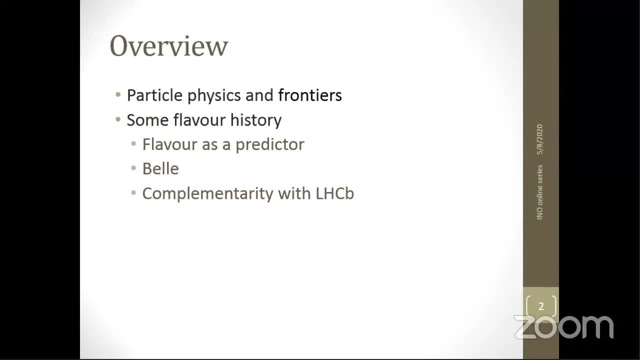 And also many of you will be familiar with Bellet 2.. You'll be aware that there is another flavor experiment which is rather different in its strategy. that operates in proton-proton collisions at the LHC, And I'll try and describe to you in a single slide why two different experiments are a 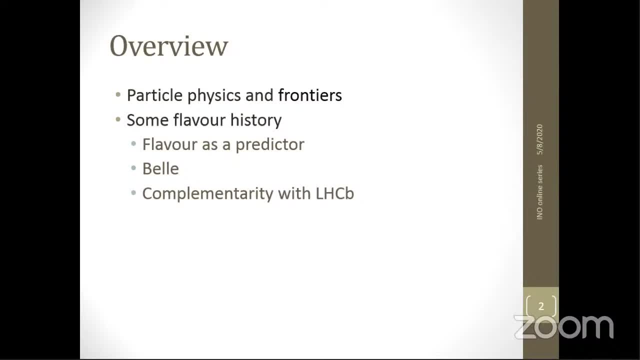 very good idea for flavor physics in different environments, And I'll talk in more detail about Bell 2.. I'll discuss some highlights of the instrumentation, Particularly actually, I should say So. I'll start with the Super Keck B, the accelerator here as well. 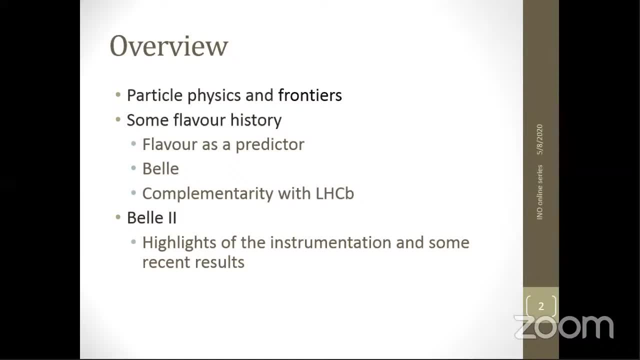 And show some recent results- actually so recent that they're taken from the iCHEP talks that are going on today- And then I'll give just one physics prospect to give you an idea of what might be achieved in the next few years, before I conclude. 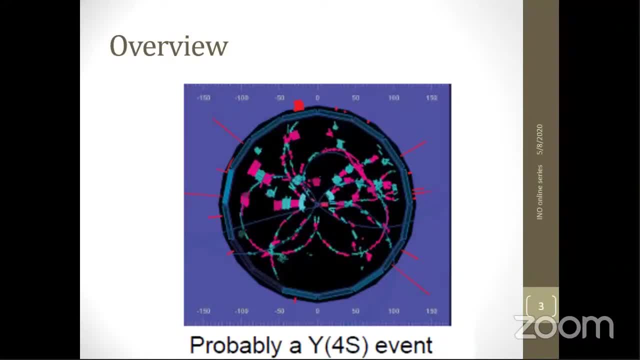 So any so? so Bell 2 is a running experiment and this is what our events look like. Okay, an E plus, E minus collision producing an epsilon 4s event. So there are a couple of things which I'll come back to in the talk. is that it's not like the event pictures that you see at the LHC. 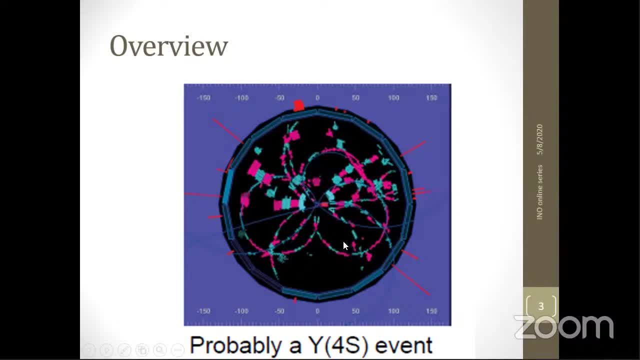 There are relatively few tracks involved and many of them are low momentum, hence they're curling around, But it's very much an active experiment now. This is probably the first B event that we saw back in 2018.. And also, we're at a stage where we want to exploit And, for those of you who are 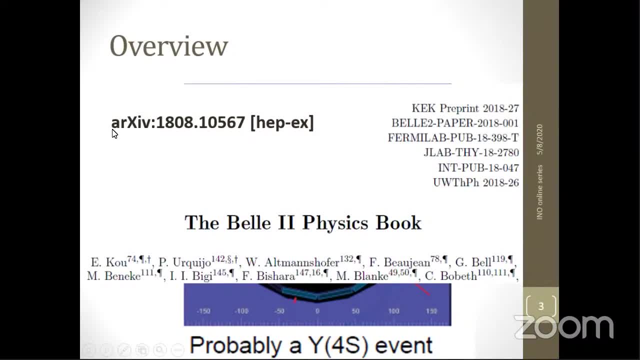 interested in the physics that I talk about. the best place to look is this rather intimidating document that we published last year, that was put on the archive in 2018, which is a physics book which describes the whole physics program, And there's no way I can do justice to everything. 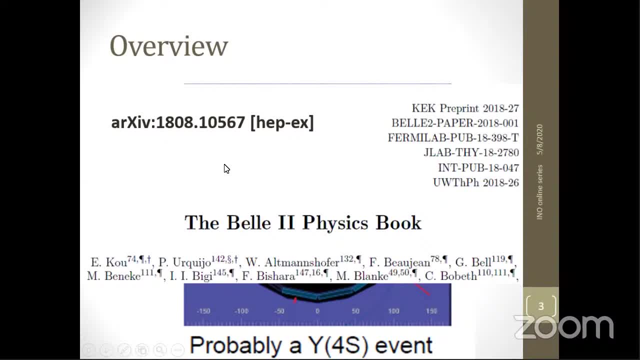 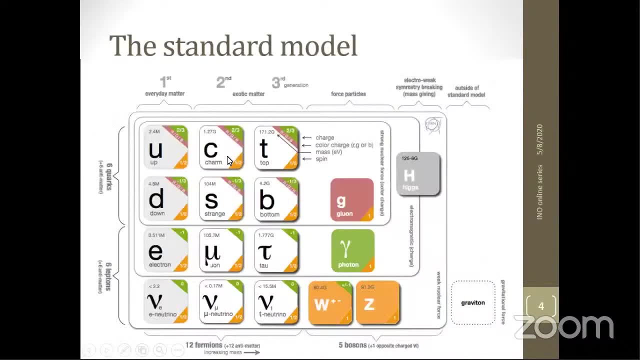 because there's so much else going on And I'll come back to this at the end. So this is just something. So the standard model- you should know this picture well- whereby we have our classification of particles into those of matter, the quarks and leptons, and then the force carriers. 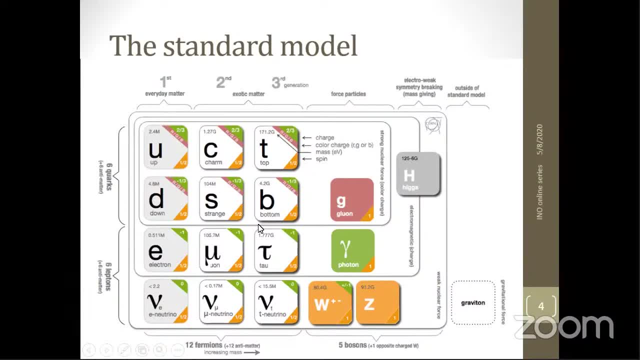 as well as the Higgs boson, And this picture has been tremendously successful since it was first put forward, And it's quite hard to actually understand how the physics program works- And I'll come back to this at the end. So this is just something. 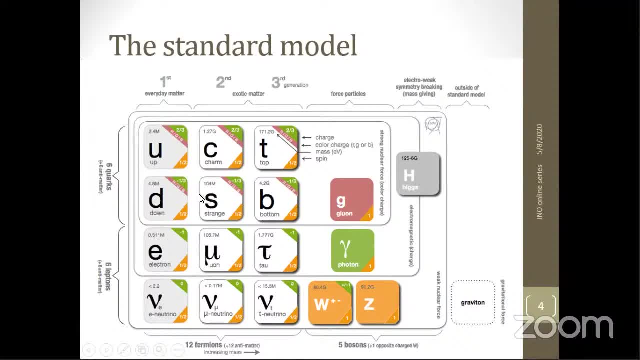 to look at And it's quite hard to understand how successful this has been. It's really confronted pretty much every single experimental challenge that's been put up to it And, as a result, as it was built up, it's been highly rewarded in terms of Nobel Prizes, Much when I give this talk. 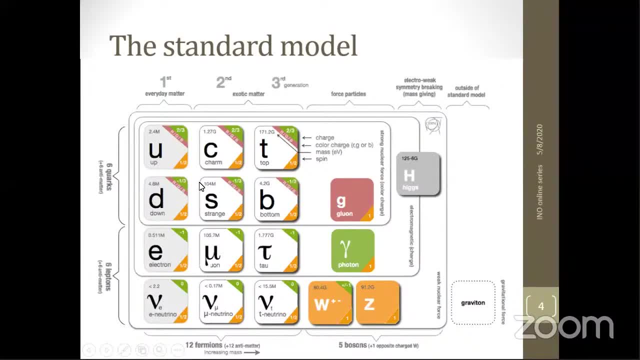 to non-particle physics people. this is somewhat frustrating to them. So just to just quickly go through how successful this has been, There have been Nobel Prizes, first starting with Gell-Mann for understanding quarks, And then Ting and Richter. 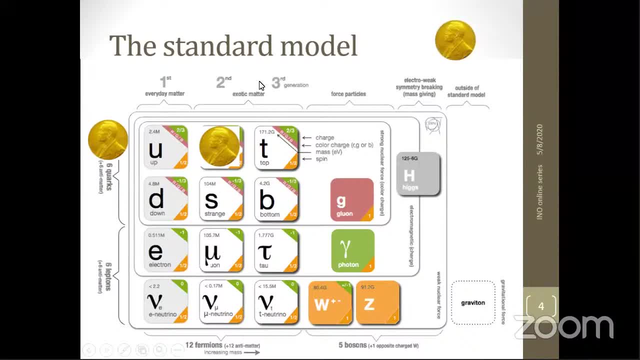 one for discovery of the charm quark, Then the overall standard model structure- Weinberg, Glasgow and Salam was given the Nobel Prize. This was followed by CP violation in strange quarks for Cronin and Fitch, Then Rubia Demir, one for the W and Z boson discovery. 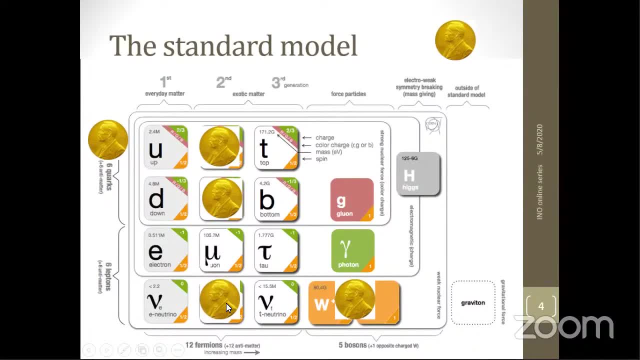 Then Steinberger et al for the muon neutrino, showing there's more than one type of neutrino. Then the discovery of partons, with Taylor Friedman and Kendall at SLAC. Then Rhinus one for discovery of the electron neutrino, Then Martin Pearl the same year, for discovery of 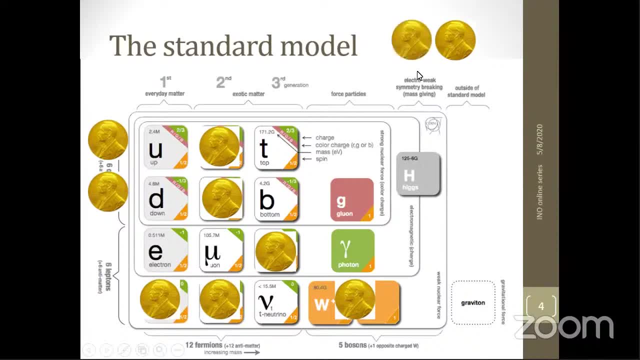 the third generation, the tau lepton, Then Tuhuf and Feldman, for showing that a locally gauge, invariant quantum field theory, relativistic field theory, is renormalizable and hence is a suitable way to describe the interactions. Then you have Gross et al for understanding the strong interaction. 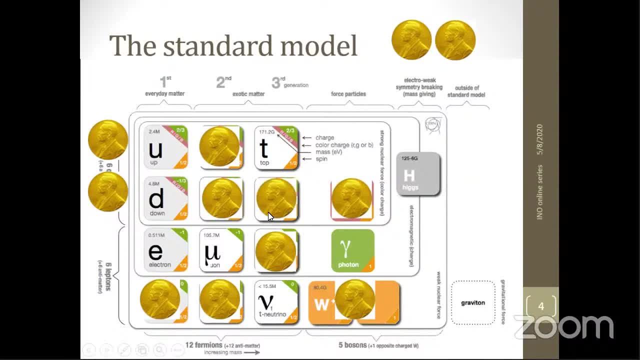 Kobayashi and Maskawa, who you'll hear more about later, for predicting a third generation to describe CP violation, Then Nambu in the same year, for spontaneous symmetry breaking, And then finally Higgs and Englert. So this is, I think, 14 Nobel Prizes for this one model of particle. 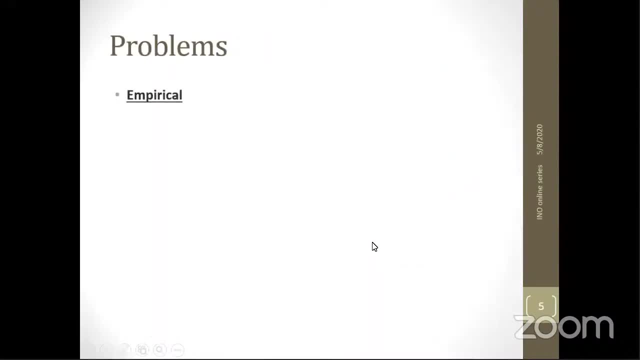 physics, But we know it's wrong. There are many problems with this, some of which are empirical. Most noticeably is that neutrinos are massive, which I'm not going to talk about in this, to this audience, but that also is the only thing of particle physics that's beyond the standard. 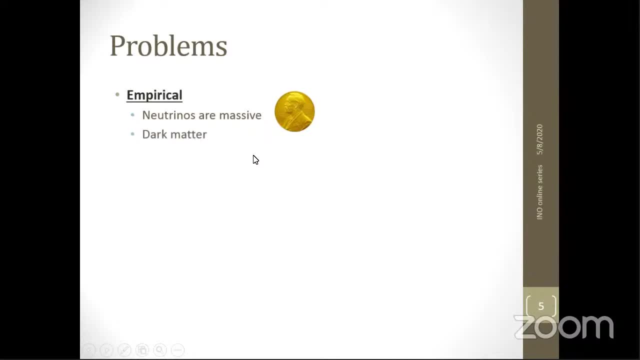 model that's won the Nobel Prize, Dark matter. we don't understand whether it has a particle nature. and what is that particle Dark energy? I don't think we really. we know it's there or appears to be there from cosmological observation, but is there some link to particle physics? 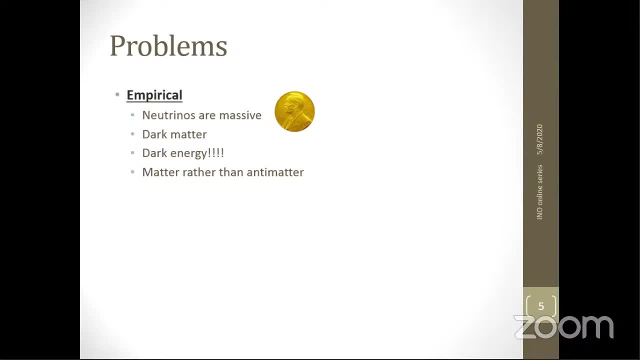 We certainly live in a matter rather than the antimatter universe. How did that arise? That's not explained by the standard model and of course, gravity is missing. Then there are aesthetic issues with the standard model as well. Why three generations A priority? that's not required and 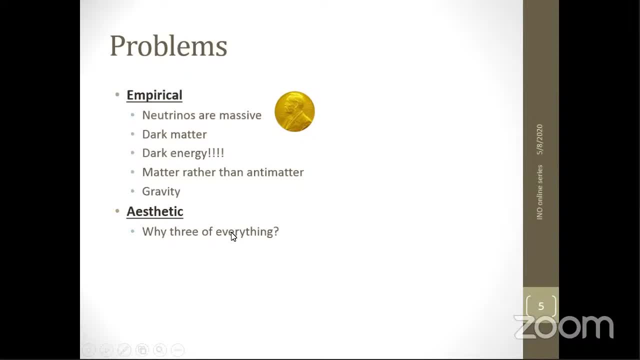 and why not four? Why not five? Why only three? Why this structure? And also why so many parameters are required to describe this. I've excluded neutrinos. I've said neutrinos are massless within the standard model. I've taken the masses to be. 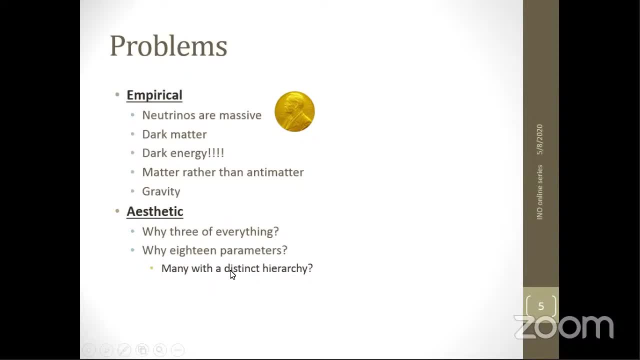 beyond that, with 18 parameters, And then also why they have a distinct hierarchy- Again something I'll come back to- And of course there's fine tuning problems: the hierarchy problem, the 18 decimal places by which you need to know these parameters, And overall you'd like to unify all. 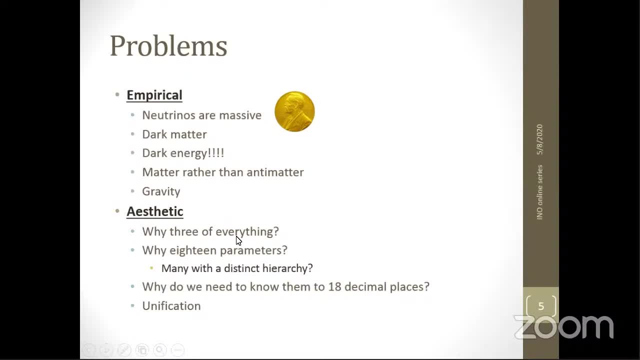 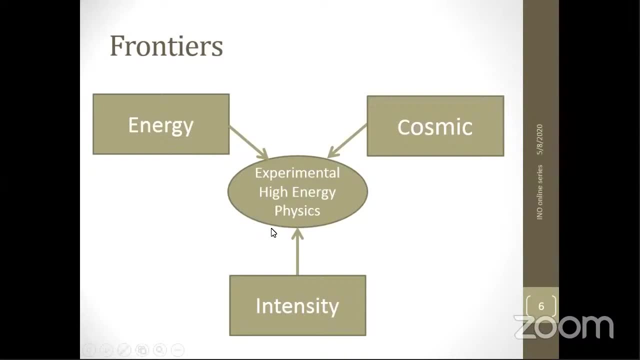 of these into one single theory, including gravity. So we approach this in three different ways. in particle physics experiments, These are the so-called frontiers. One has the energy, the cosmic and the intensity frontier, And this pretty much makes up all of experimental. 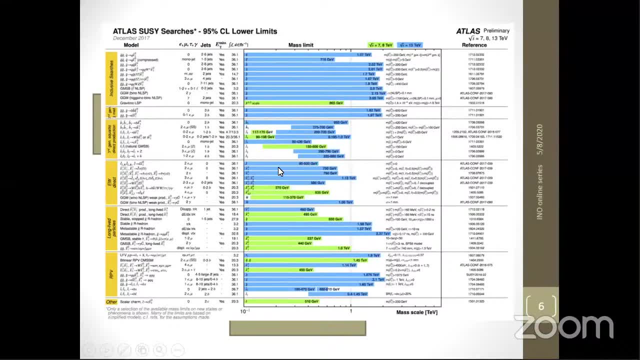 particle physics. So for the intensity frontier, that's the LHC, This is a plot from ATLAS showing the limits that they set on beyond the standard model supersymmetry. So this is trying to produce massive new particles at the TEV scale directly and then observe their 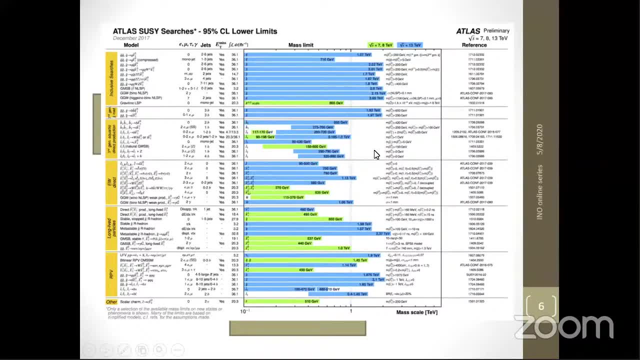 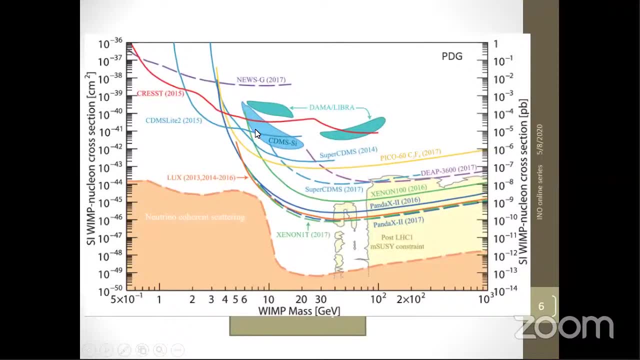 decays inside the general purpose detectors. So this is one route to discovering new physics. Then you may well have seen plots like this. This is not quite up to date. This is from the PDG, where you're looking at the detection of a WIMP-like candidate for dark matter. 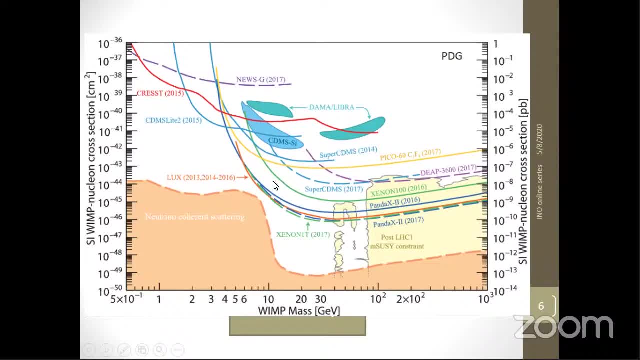 a weakly interacting massive particle. And this is a plot from the PDG, where you're looking at, where you have these very sophisticated experiments, often working in cryogenic environments, trying to detect the small amounts of energy deposited when dark matter scatters off. 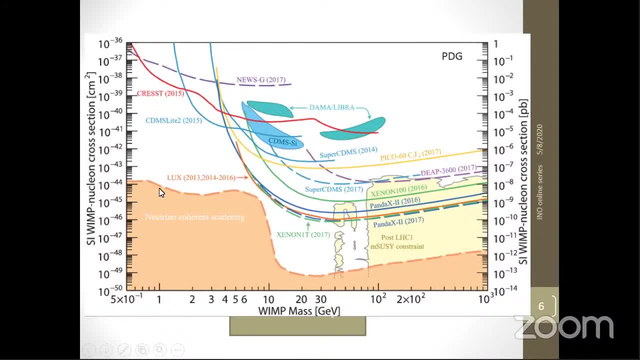 a nucleus, And these limits are pushing down now to very low cross-sections and to what might be the limit when you actually start having background coming from neutrinos in these experiments. So I apologize, you're going to hear a cat occasionally in the background. I can't do. 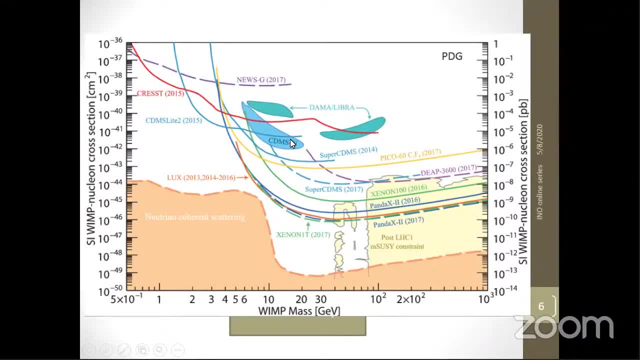 anything about that. So this is a plot from the PDG, where you have these very sophisticated experiments, often working in the dark matter, And she will choose the most inopportune times to start shouting. So that's the cosmic frontier, but what we're interested in in this talk is the intensity. 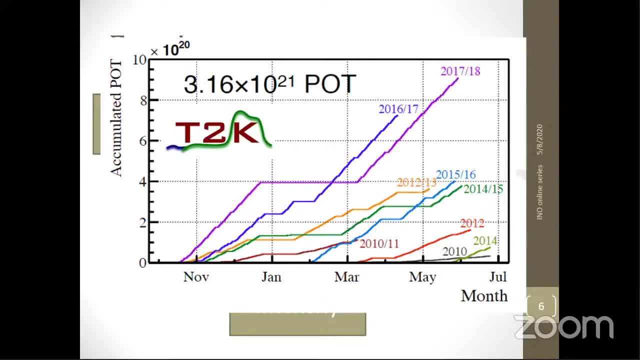 frontier. So from neutrino physics, if you take an intense beam here, generated by Jay Park, and fire towards the super camion candy detector, you have the T2K experiment and they measure the number of protons on them, the number of particles It's impossible to differentiate. 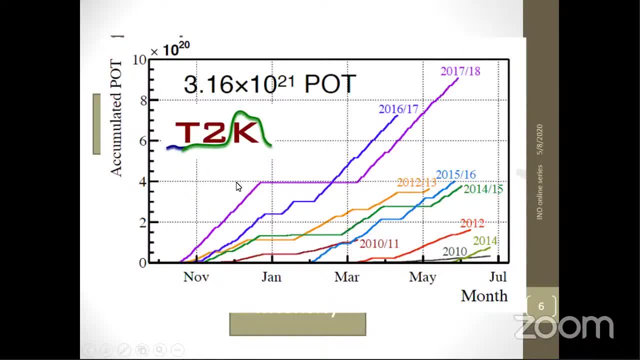 The solution to these two problems is actually to take the very high intensity of the super camion candy detector and start very close to the super camion candy detector target that they have um as their sort of measure of um, the number of neutrinos they produce, and you 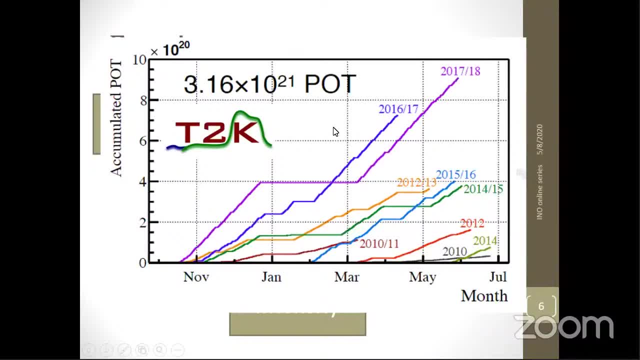 see, this is just a program of trying to get as many events as possible to measure parameters precisely, and that's exactly what we're going to be doing in the bell 2 experiment as well. we're going to work at this so-called intensity frontier, which is all about getting as many events as 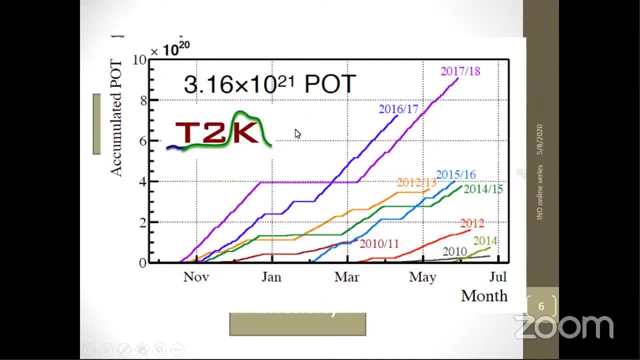 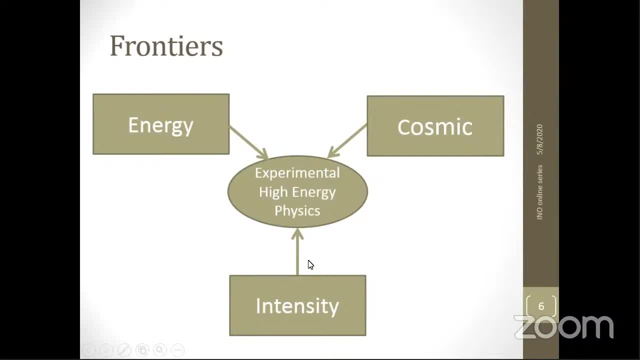 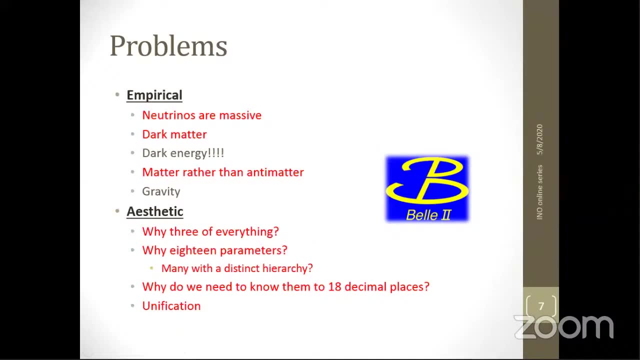 possible and doing precision measurements and searching for very, very rare decays. so that's oriented ourselves as to where the intensity frontier fits in in terms of bell 2, and bell 2 in principle can tackle virtually all of these problems. so the flavor puzzle in terms of why we have three generations in the hierarchy, is very much at the forefront of that. 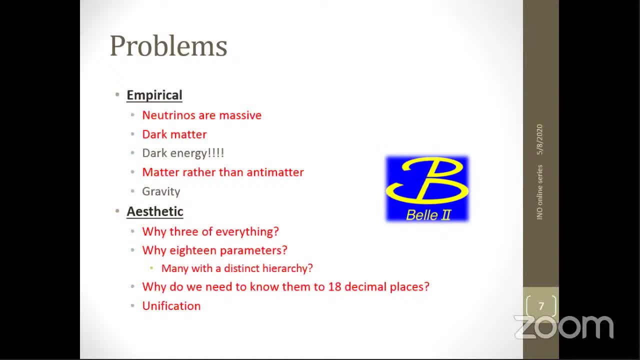 but we're also indirectly sensitive to many other things as well, and whatever standard model beyond the standard model physics there is should affect some of the measurements that we have. And if we don't see anything, these null tests that we have will also suggest that the mass scale of 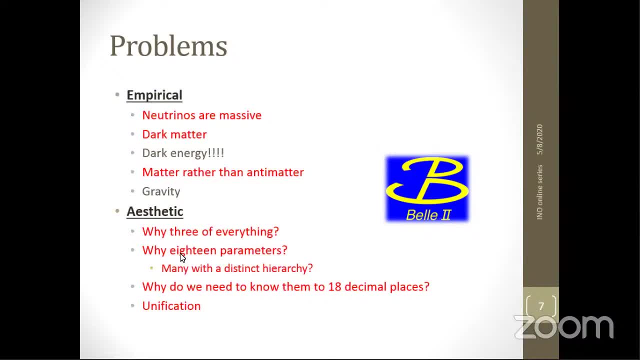 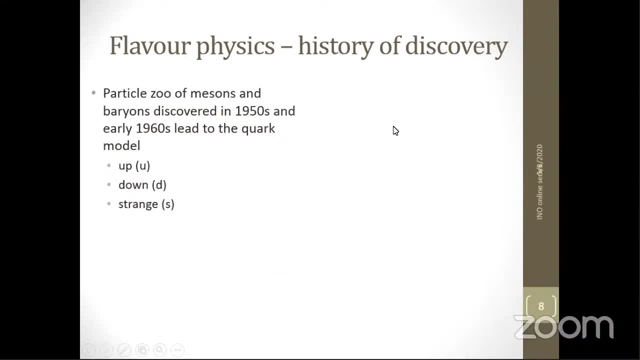 any new physics is extremely high. So those in reds are things I think Bell 2 can in some way address. So flavor physics. now the history of this. So, as I alluded to with my slide on the standard model in the early 50s and 60s there were many, many particles and not much sense could. 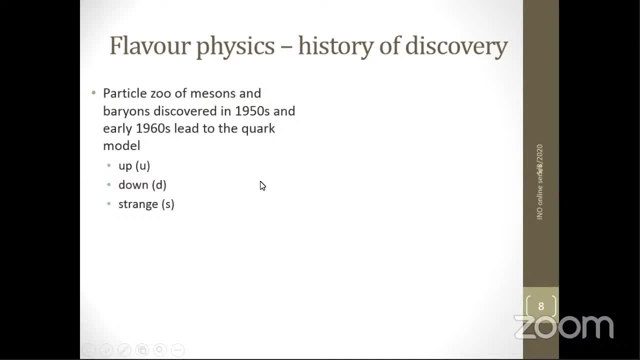 be made of them. Some were considered strange because of the way that they decayed, But Gell-Mann and Zweig put order upon this by suggesting the quark model And by understanding that these particles that have been observed have been made up of these three quarks. you could very much 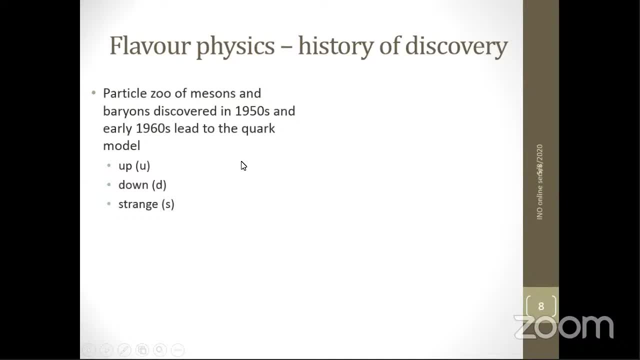 explain the lowest lying non-ets. So you can see that there are a number of different types of mesons and the octet and decouplet of baryons, as well as some other particles that were observed. So with these kind of discoveries, you 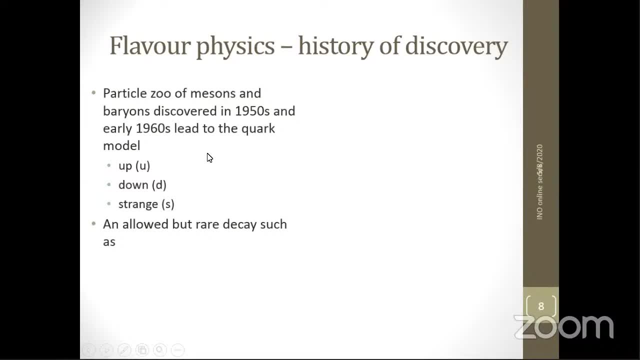 can actually study these particles more and more, And an example of a rare decay very much in the flavor sector is where you have this rare decay of a long-lived neutral kaon going to two muons. So this is a less helicity suppressed than the electron version of the decay. 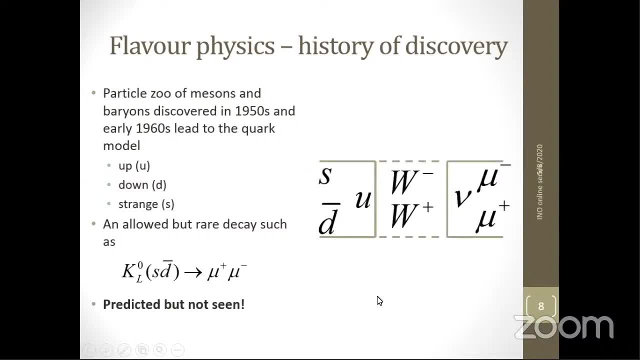 And so how this proceeds in the standard model was that you would have this second-order weak diagram where you have this box where you have the flavor transitions of the quarks mediated by the W, on one side to annihilate your neutral kaon, And then, on the right-hand side, the final. 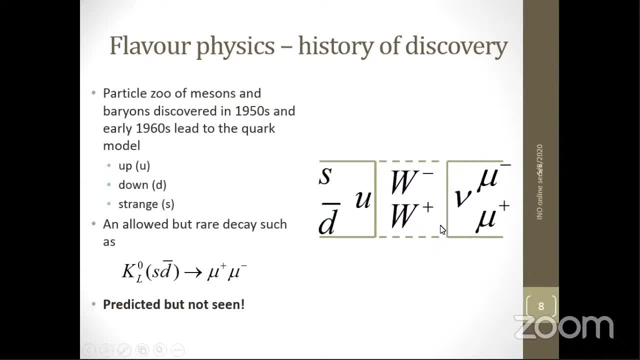 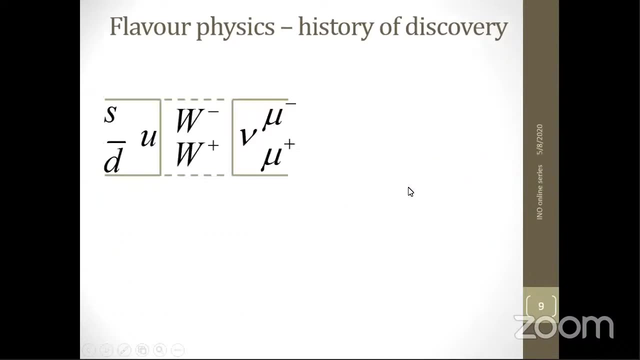 you'd have leptons linked together by the W's And this could be written down and thought about in terms of second order weak interactions. But the problem was that this decay was not seen at all. So how this was resolved was by these three gentlemen: Glashow, Iliopias and Maiani. 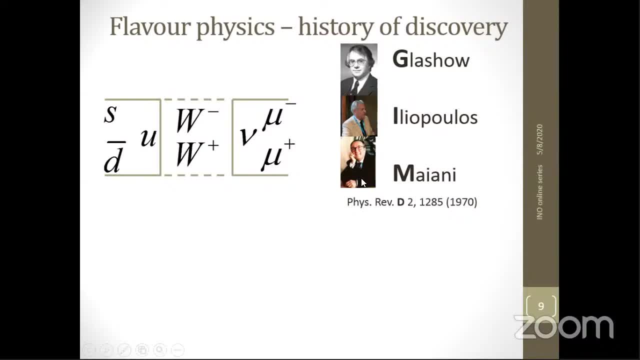 so-called gym mechanism suggested that a way to get around this was to have a fourth quark. So at this time there's no experimental evidence for this fourth quark. They suggested this to fix a problem in terms of a flavor observable, And here. 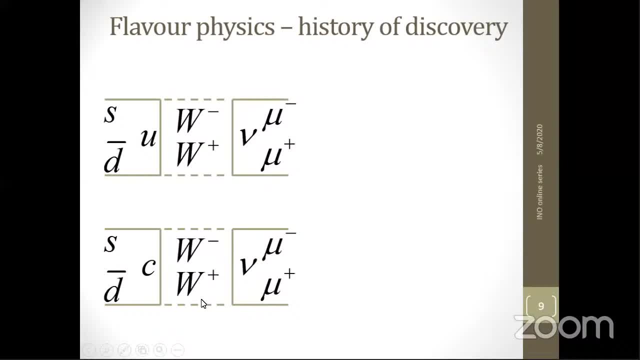 once you introduce the charm quark you get a second diagram where instead of the virtual U quark being exchanged between the strange and the anti-down quark, you have a virtual charm quark. And once you add in the various Kibibo factors to this, you see that there's a sign difference. 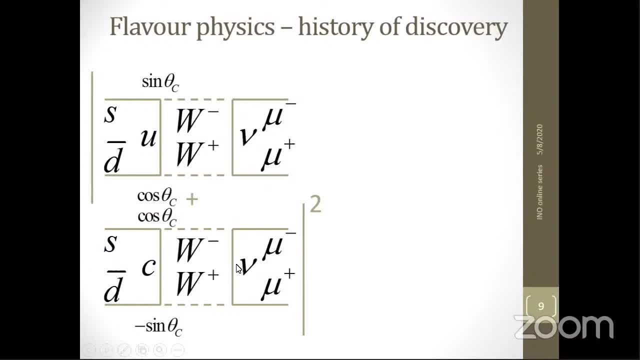 between these two different decay diagrams two amplitudes. So once you sum those coherently and square them up to effects related to the difference in the up and the charm quark masses, these two diagrams cancel each other out, giving you a rate approximately equal to zero. 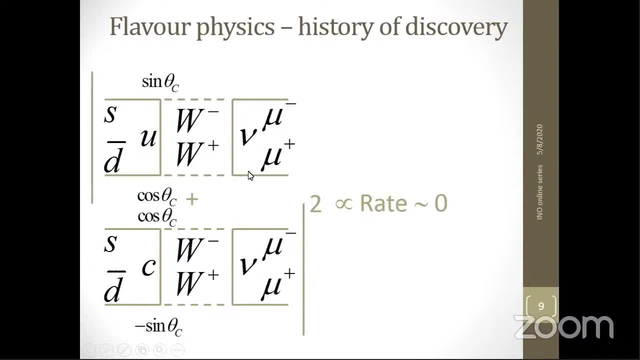 hence explaining the difference between the two, the rate of suppression of this decay. But because the up and the charm quark are not quite degenerate in mass, the decay does actually happen, and at a rate which you can then postulate what the mass of the charm quark was, which people did. But this is an example of a 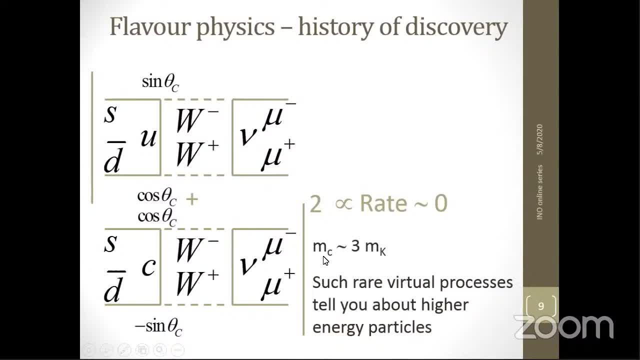 virtual process. You're not directly observing this charm quark, which has roughly three times the mass of the kaon, by looking at this process, which is actually at a lower mass scale, And that's the whole idea behind this. So this is an example of a virtual process which is actually 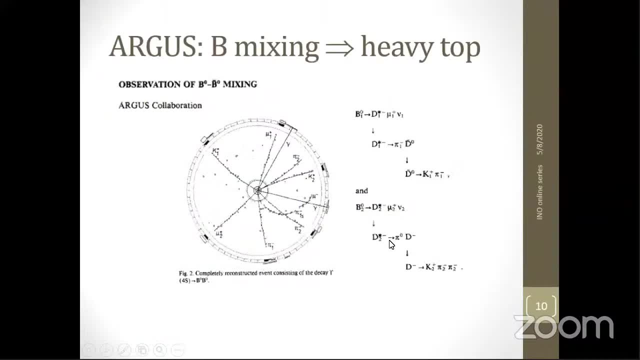 at a lower mass scale, And that's the whole idea behind making precision measurements in the flavor sector. So another example quickly, is that when bee mixing was observed- I'll talk more about bee mixing shortly- This was seen by having two bees decaying, where they both decayed to the same. 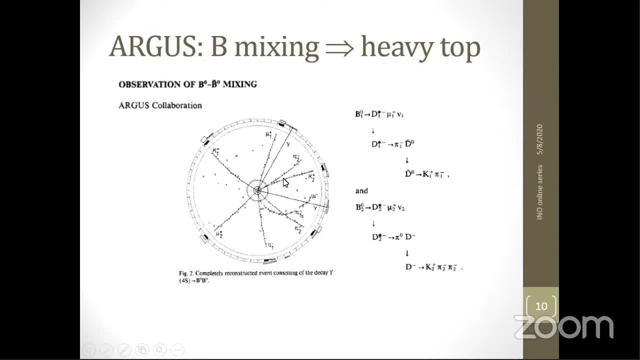 charge of lepton suggesting the bee mesons had one bee meson at least had oscillated And the rate at which one saw. so yeah, I've drawn the diagrams. it's very similar to the Kaon diagram, But now with the, with quarks on either side, and again you have this box. 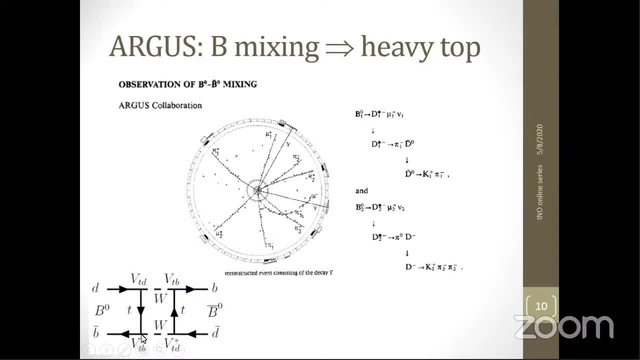 but in the box, because you have beauty in the top quark. there's a strong coupling between these two, So it's dominated by the top quark. So the rate at which this happened told you that the top quark was very, very heavy compared, say, with the scale of the bee meson and much beyond. 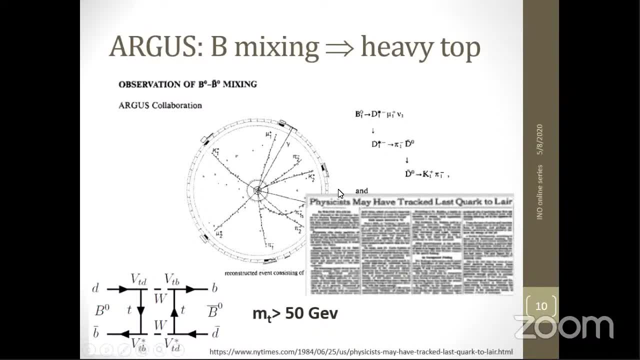 the scale at which people were trying to observe it, even though UA1 had optimistically claimed its level of gravity at the SPS back in 1984, but the mass was far too light for this to possibly have been discovered there, And you had to wait till the Tevatron before it was seen directly at 175 GeV. 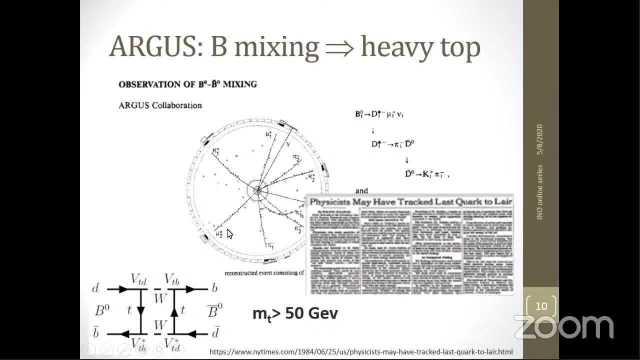 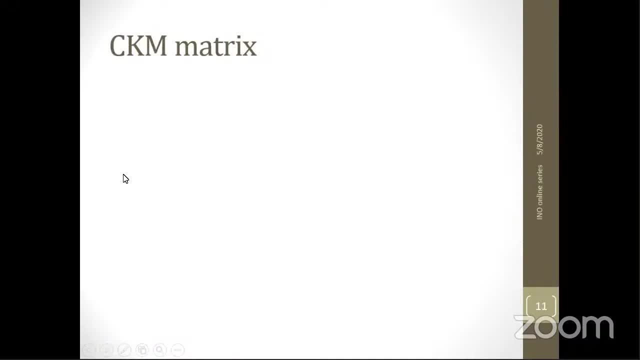 So these are examples of where flavor measurements have been able to predict physics at higher mass scales. So to understand a lot of what we do in terms of the measurements at Bell and Bell2, we look at the CKM matrix. So I've already mentioned the Kibibo couplings in the first two generations. 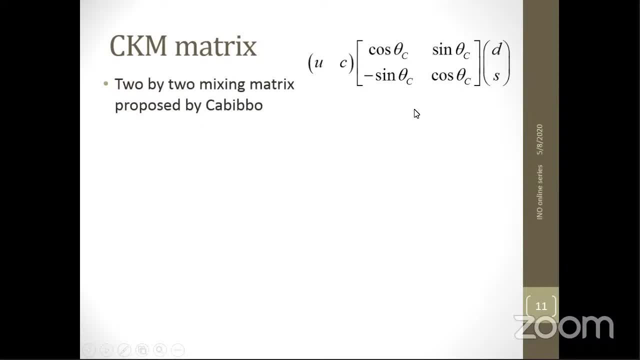 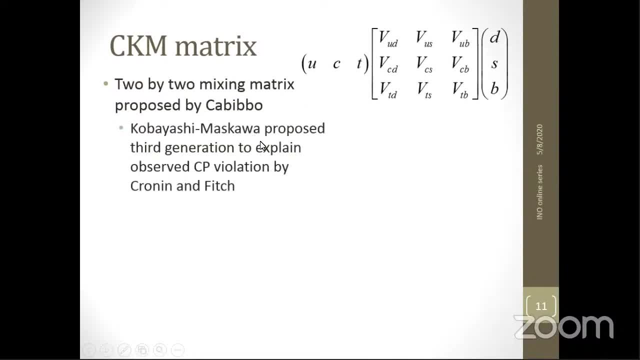 Now Kobayashi-Maskawa, who I've mentioned. they made the bold prediction, before even actually the charm quark had been observed, that to have CP violation, as seen in neutral kaon decay, you needed a third generation of quarks. And they had this, three by three. 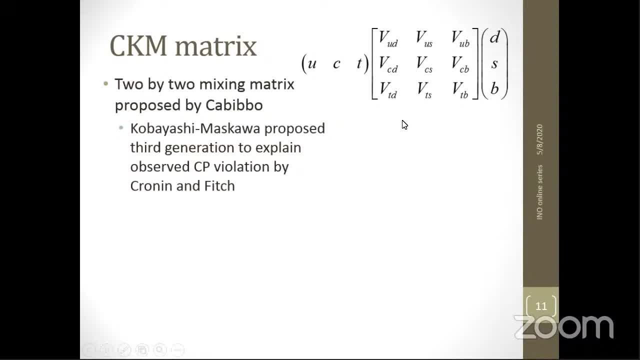 matrix, which is just the extension of the Kibibo model for quark mixing, And why they said you, you needed three generations, was because to describe this three by three, unitary matrix, as well as being using the ability to take phases that are unobservable into the quark fields. five: 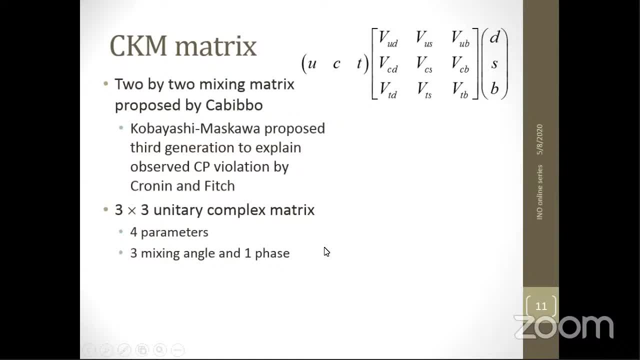 of those, you can show that you need four parameters to describe this matrix. Three of them are like Euler- angles, rotations in this three-dimensional space- and one is an irreducible phase, and it's this phase that allows CP violation to occur. So this also shows up something about the CKM matrix. 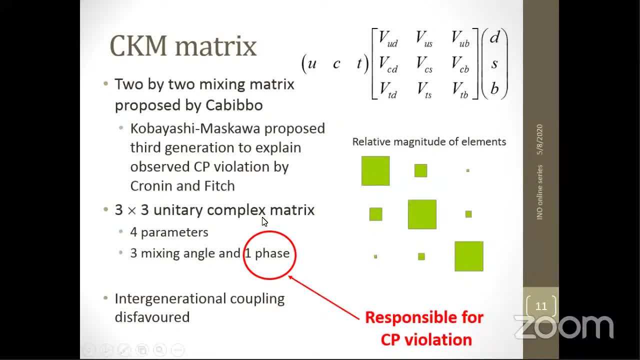 and particle physics in general. So these parameters, four parameters you put in by hand, but there's a strong hierarchy to them, that the diagonal elements, where you're coupling together quarks within the same generation, are large. If you couple between adjacent generations they're substantially smaller. 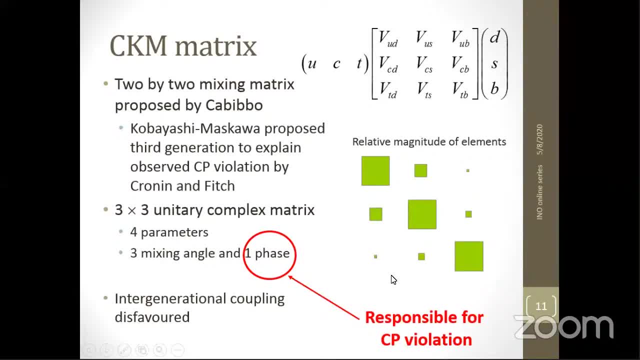 But they're smaller still if you go between the first and the third. so these very small dots here- they're trying to describe the size of the magnitude of these elements- are for VUB and VTD, which are rather small. So this structure is very important to why we are doing B physics and trying 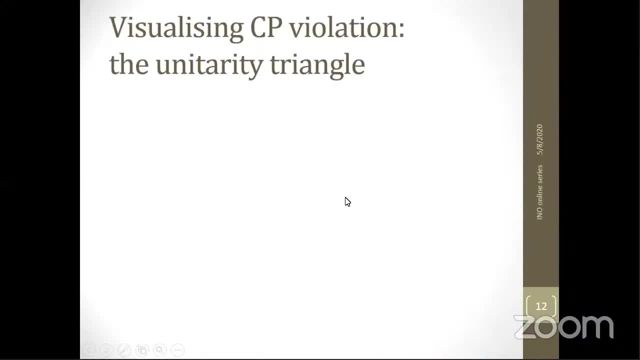 to study CP violation there, as I'll explain. when we look at how we visualize it in the standard model through something called the unitarity triangle, So we use what's known as the Wolfenstein parameter. So this is an unilateral parameterization where there is this parameter lambda, which is just sign. 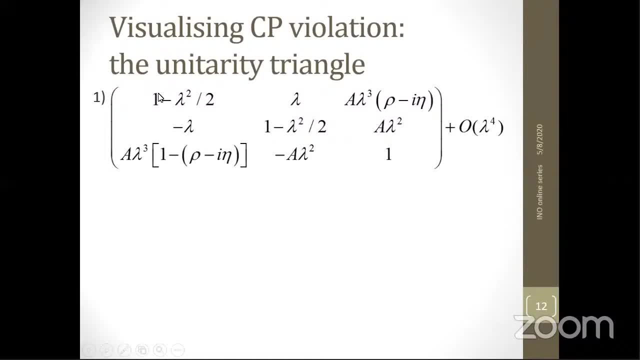 of the kubibo angle. So you write this, the first two generation mixing in terms of sign of the kubibo angle, and then you introduce these other parameters, a, rho and eta, to describe these off diagonal elements, and these parameters are all of order one and the expansion parameter lambda is. 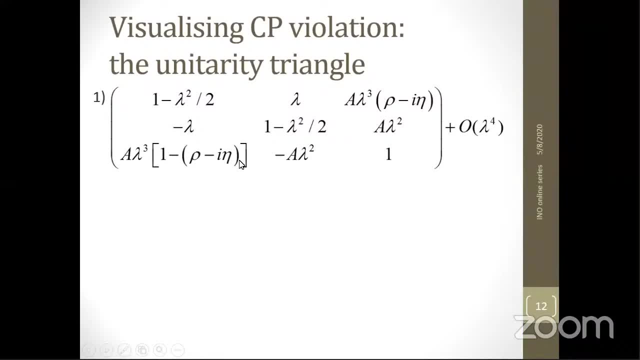 making the off diagonal element smaller. so lambda is 0.22 in the standard model. So you have then higher order terms. but you essentially look at these, this, this, this to this triangle, to order of these, the CKM matrix, to order lambda, cubed, and then you exploit the fact that it must. 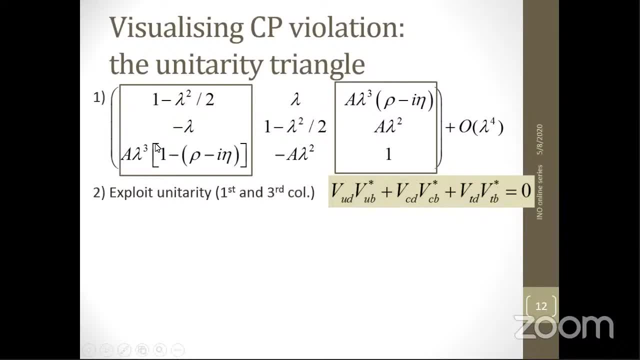 be unitary, unitary matrix. and if you look at the first and third columns, you can construct this relationship between the various elements of the CKM matrix which have to add up to zero. and because you have these complex elements due to the CP violating phase, you can also visualize this in the Argand plane and each of these terms in this expression. 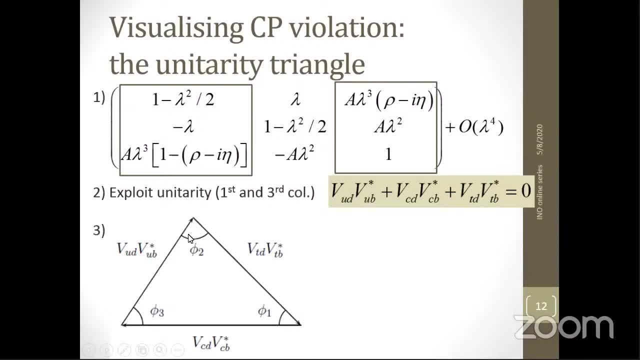 can be seen viewed as sides of the triangle. that has to close if you're satisfying this unitarity constraint. And what you should notice about this triangle is that each side depends on a coupling with the b quark as VUB, VTB and BCB. hence we're very interested in looking at studying CP. 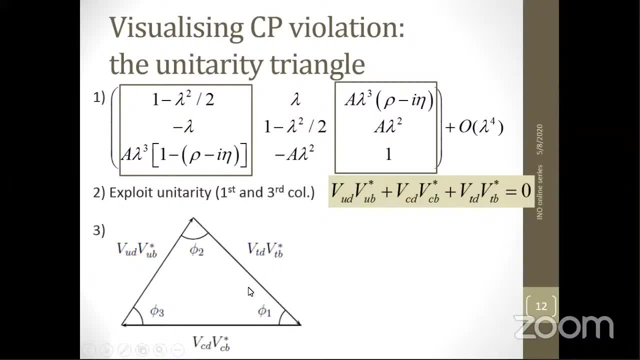 violation in beauty quarks. and this is the only triangle where you get the sides all to be roughly the same length, because each side is of order lambda, cubed, whereas if you look at other triangles, you'll have one side that's very small and the other side of order lambda or something so this. 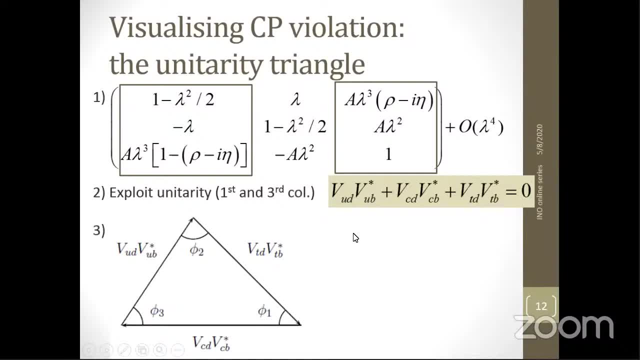 isn't the only triangle in which this happens. so you can see that the two sides are the same length, and so you get non-trivial values of the angles which Bell calls phi one, phi two, phi three, and the rest of the world calls alpha, beta and gamma. so these are just the internal angles of this. 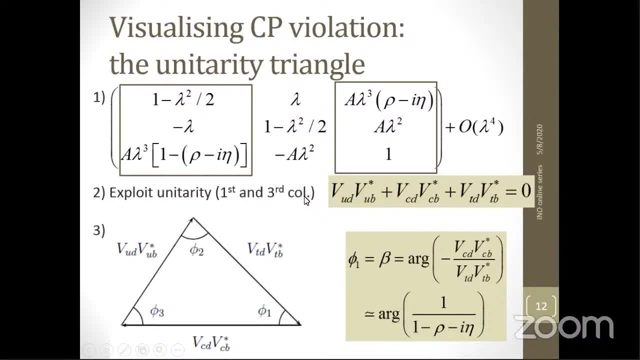 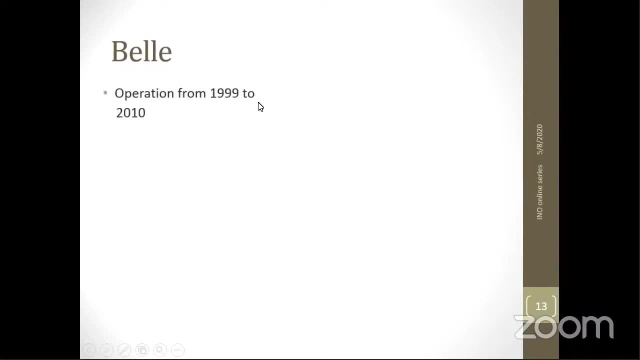 unitarity triangle, and I'll talk more about phi one or beta, in the later part of this talk. so, yeah, this is the other convention that you may be familiar with. so, Bell, this was an experiment that ran between 1999 and 2010.. It was an asymmetric E plus E minus collider at the Upsilon 4s. 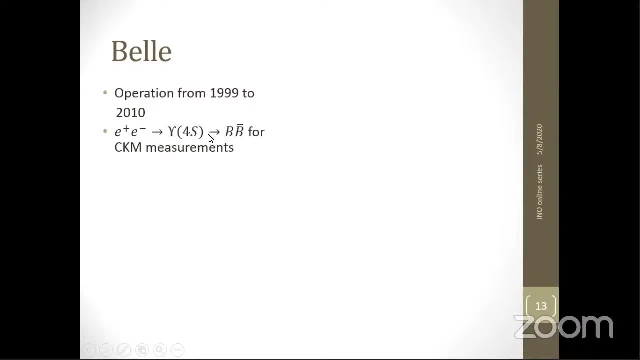 which is just above threshold for open beauty production. so the Upsilon 4s can only decay to a B meson and anti-B meson with no other particles produced, and it was designed to make measurements of this unitarity triangle, and the asymmetric energy, which I'll explain in a moment, was to allow. 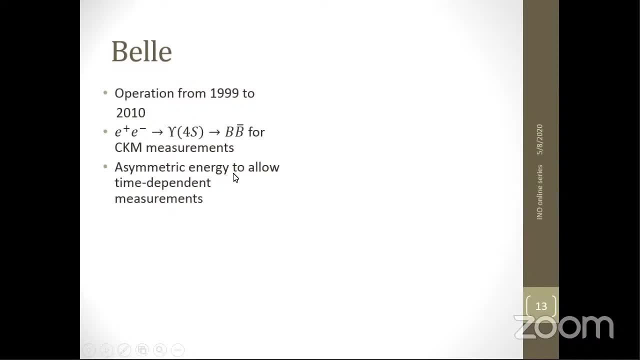 time-dependent measurements of Cp violation. so the other advantage one has of producing B mesons through this E plus, E minus collision with no other particles is that there's coherent production of the neutral pair, which means they're in a quantum correlated state so they evolve coherently. so you always have a B zero and a B zero bar until one of them decays. 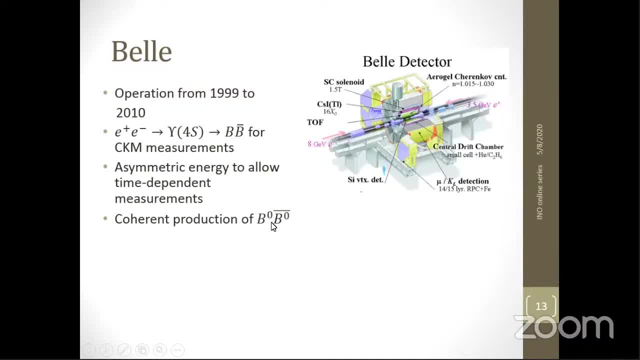 so this is very helpful for the time-dependent measurements. so it's quite a complicated idea. so the Bell detector was very much like any four pi spectrometer that you're used to, with the small difference that there's a asymmetry in the beam. so the electron beam had HgeV. 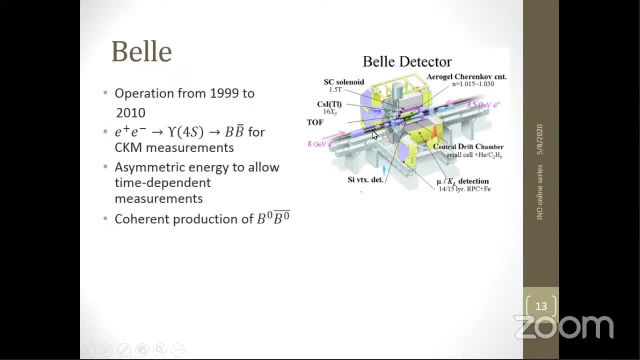 and the positron beam had 3.5 GeV, so the center of mass frame was moving in the in the laboratory frame of reference. so again, operating at this um Upsilon 4s, with just the two B mesons produced, there's very few differences between the two beams and the two beam mesons. so 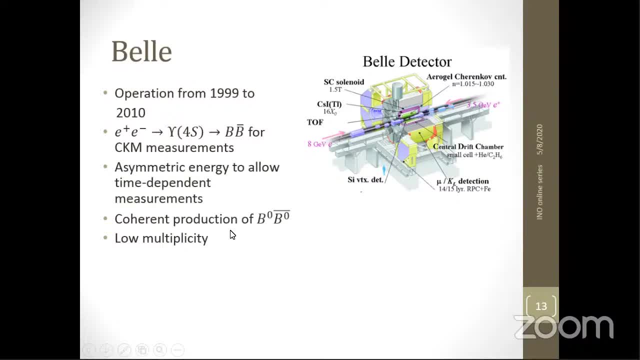 There's very few particles in the final state on average. You have less than 10 as particle multiplicity on average at this center of mass energy. And then you identify all those tracks using good tracking: electromagnetic calorimetry, hadron identification using Cherenkov, radiation and time of flight. 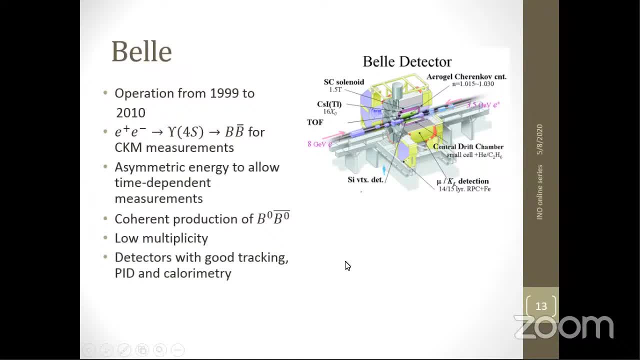 And you also had a muon filter to detecting muons And you could actually fully reconstruct events, where you reconstruct all the particles- And again I'll talk about that later on. But once you've reconstructed everything and you know your initial conditions, you can also reconstruct the missing momentum. 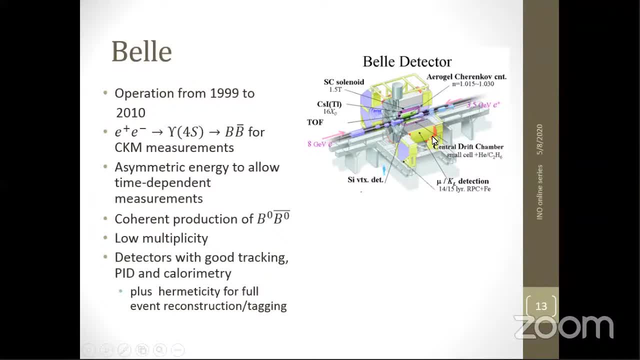 So you can essentially reconstruct neutrinos or weakly interacting particles- exotic particles as well- by looking in this kind of environment, because you have good control over your initial state kinematics, unlike proton-proton collisions. So there was a partner experiment at Stanford called BABA, which did not accumulate as much data but was highly successful in the early days. 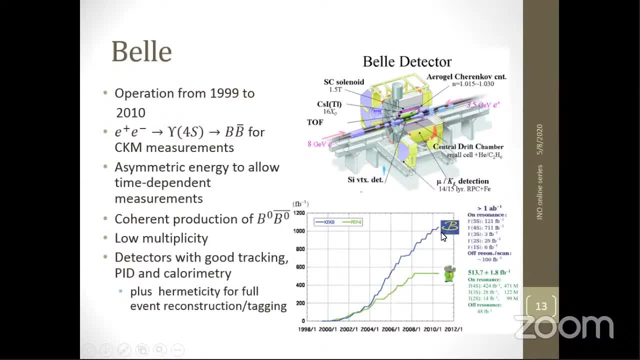 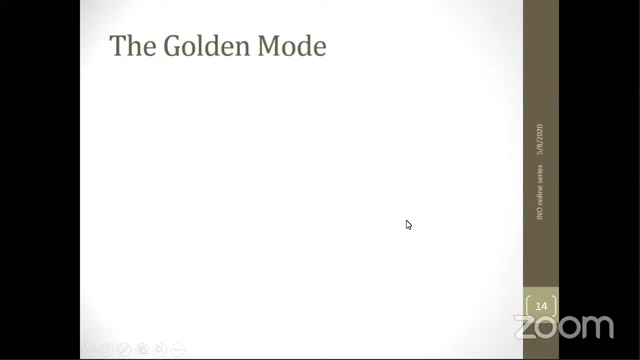 But Bell went on to collect one inverse atoban of data, which is a large amount. So, as I'll talk about this, But later in the talk I should just discuss the reason why we had this asymmetric collider, And this was because they wanted to measure CP violation in the B sector. 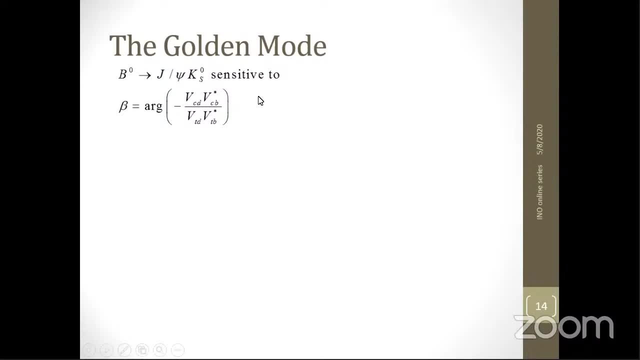 And this comes from this J psi k, short decay of the neutral beam is on- And this is our angle of the unitarity triangle And with a B0, you have this mixing process going on Which depends on this VTD CKM matrix element, which is one of the two complex ones in our Wolfenstein parametrization. 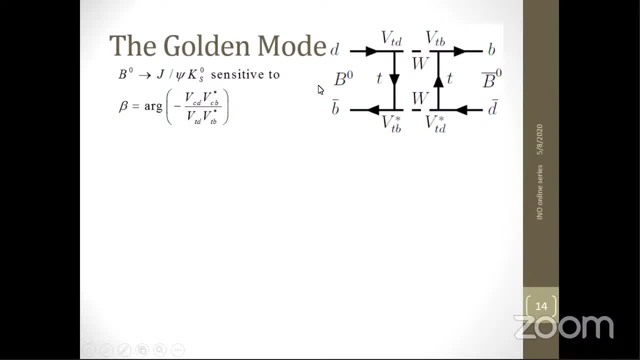 So that gives you some sensitivity to the CP violating parameters. But you can't measure a phase from a single diagram. You need to get interference. So you have an interference term to get hold of the phase information And how you get that interference in J psi k. short is that you have a diagram for the B0.. 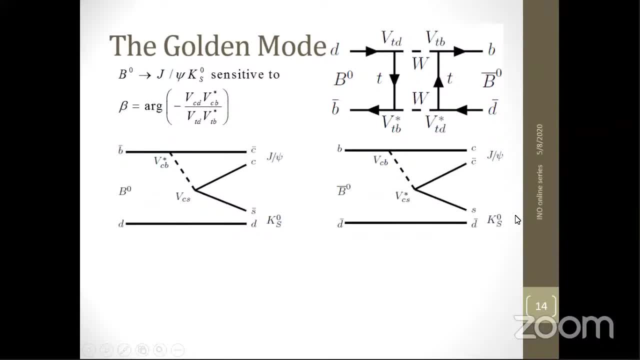 And the B0. You have a B0 bar that can decay to this same final state And these two interfere, with or without B0 mixing, And you can actually plot whether, as a function of how long the bees lived, The B0 bar has a probability of decaying to this final state or not. 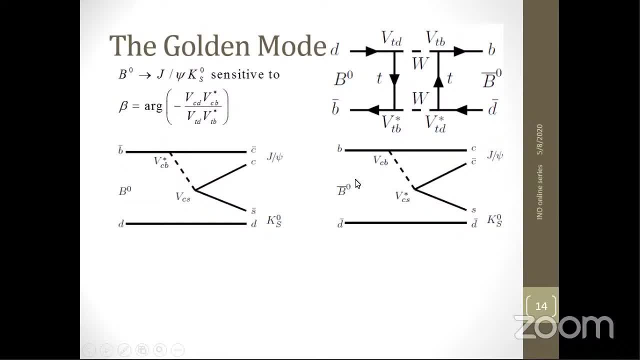 And you actually build up an asymmetry that depends on these parameters inside the mixing diagram, the weak parameters. So this relation: through the interference of mixing and decay you can have direct CP violation as well, Or you can just have CP violation in mixing, as long as you have the interference. 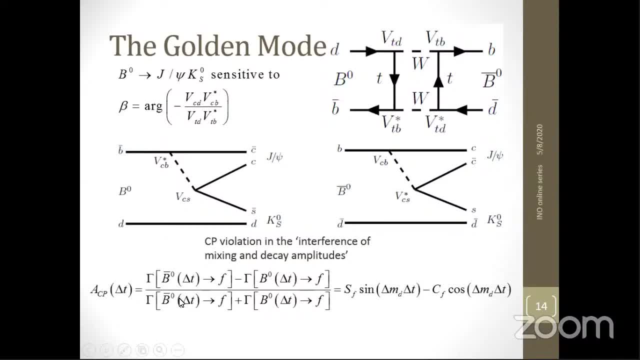 But you end up with this time-dependent difference between B0 bar and B0 going to this final state- F, J, psi, k, short- And then you normalize it to the sum of the two And you build up this time-dependent asymmetry. It depends on the mixing rate, which depends on the mass difference, this delta md. 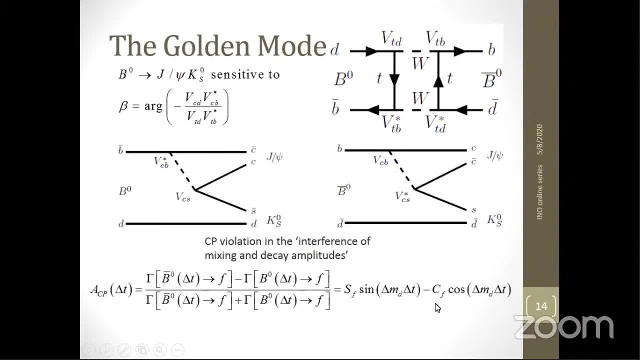 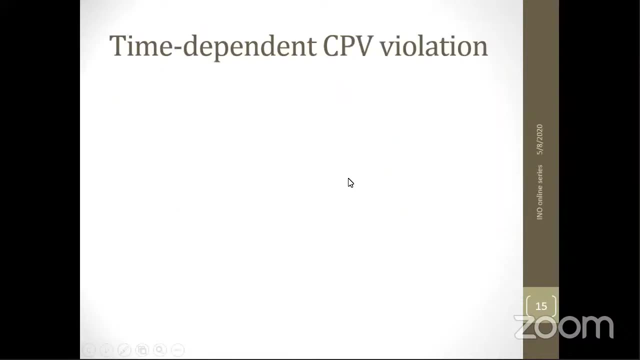 And then these parameters or coefficients, And in the standard model, you expect this cosine term to be zero And this Sf is just related to sine 2 beta. So this is how these time-dependent measurements, But why we had the boost was you need to measure this as a function of time. 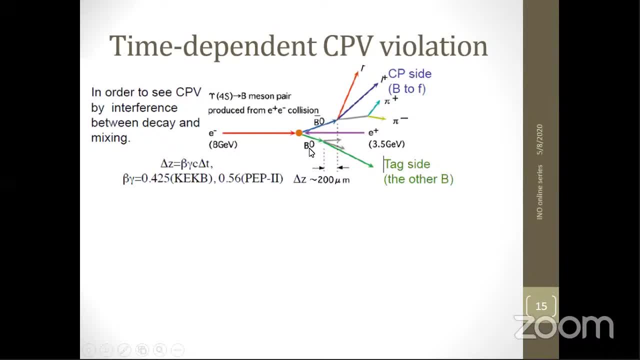 Technically because of this correlation, it's between the B0 and the B0 bar in bell and bell 2.. So with this boosted frame of reference, the two decay vertices for your B0 and your B0 bar for some distance apart. 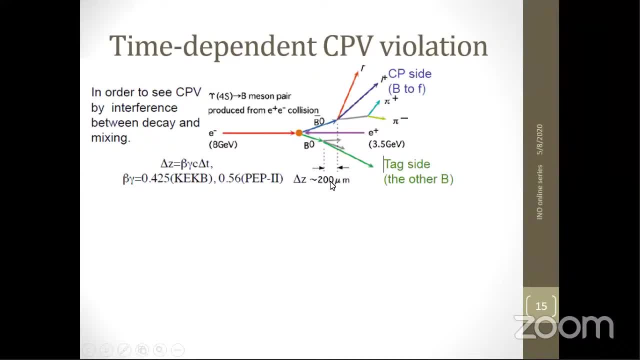 delta Z on average around a fifth of a millimeter, 200 microns, And one side you had your signal decay And on the other side you had a generic decay from which you could tell the flavor of that B. At the time of decay you had a generic decay from which you could tell the flavor of that B. 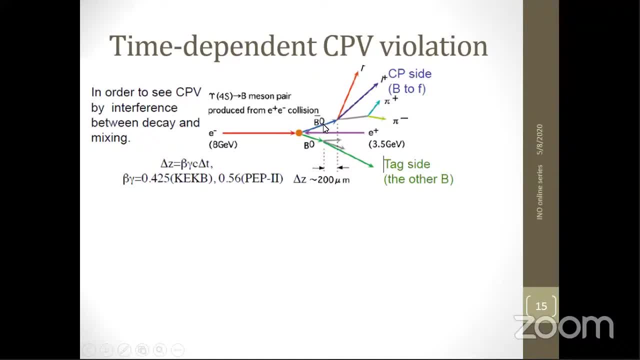 At the time at which it decayed, And that tells you that it's the other sign over here. So you just worked out, given the time difference and the number of Bs that you had at production and at decay, how you could build up this asymmetry over time. 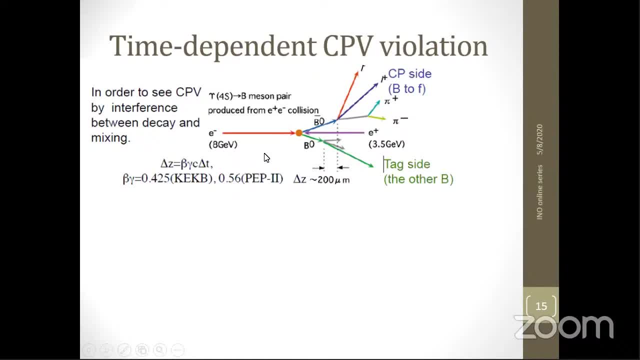 And you did it in terms of this difference because of the quantum correlation between the B0 and the B0 bar, And you have to get the flavor of the B right To make this measurement and you can do that with around a 30 percent efficiency. 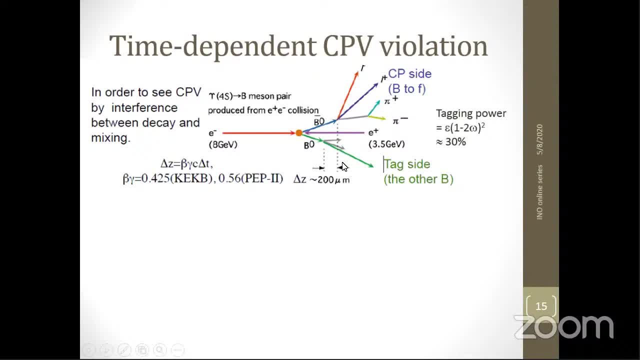 So this omega is the mistag rate and the efficiency is the chances of having some signature by which you can tell what the other B flavor was, usually the charge of a lepton or charge of a kale. So these measurements were made and you see the sinusoidal variation. 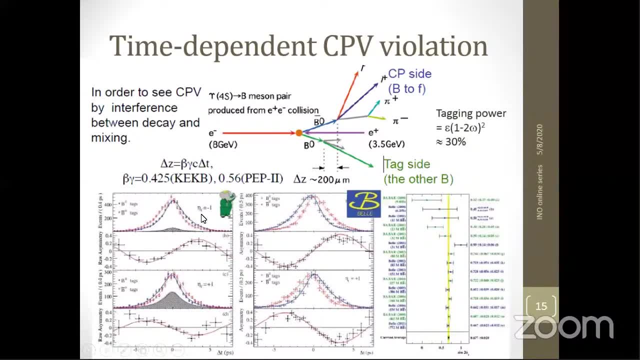 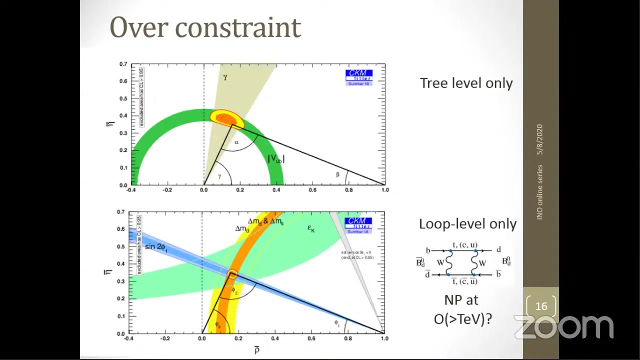 If you look at the difference between B0 and B0 bar for both the Babar experiment and for Bell- And they had agreeing results for this sine 2 beta- And you can see that the B-sector was a bit more. So the goal with all of this is to measure the unitarity triangle as precisely as possible using different measurements. 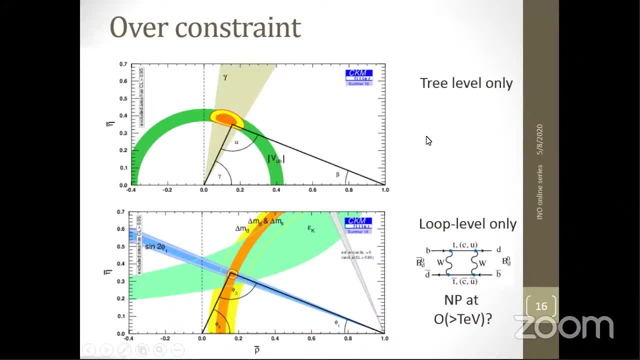 And, in particular, you can separate this into measurements that are only going to be used for the B-sector, And you can see that the B-sector is the most common one. And you can see that the B-sector is the most common one. And you can see that the B-sector is the most common one. 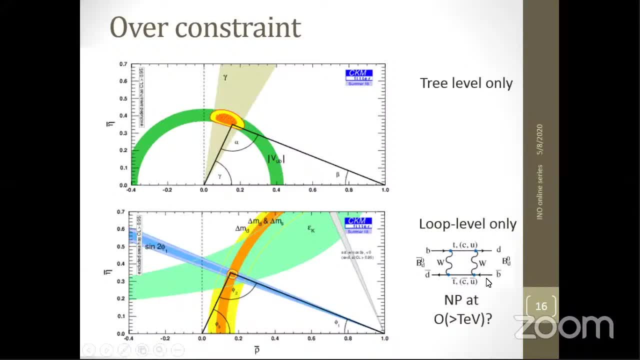 It's going to be a tree level where you have no loops at all, and that that can be done through semileptonic decays and also by direct CP violation in gamma. And you have this sine 2 beta measurement and the rate of mixing which fixes the length of this side, and 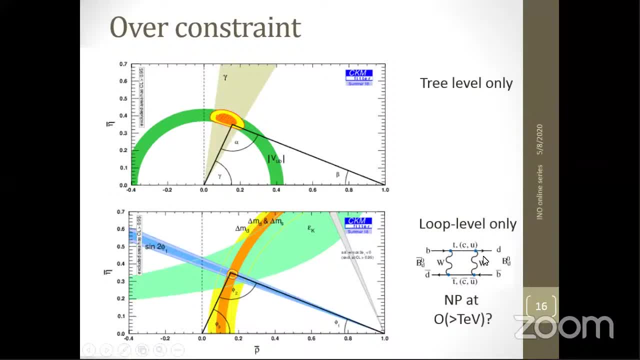 also some measurements in the Kaon system which are related to loops and box diagrams, Heidelberg line periods And on video. on the right, if you're pressing down to a very important tributary value and from της and new physics at scales very much greater than TeV could influence these different measurements. 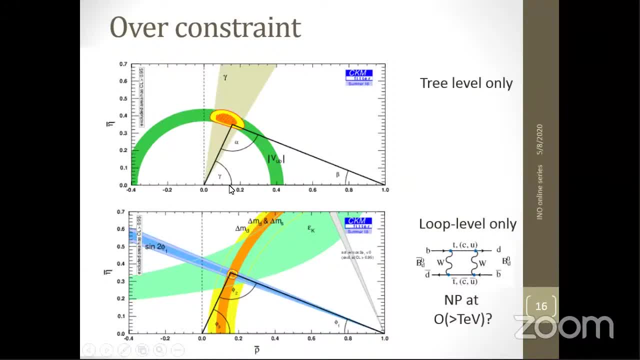 But what you notice, this yellow-red region here, is how well you measure the apex of the triangle with these different measurements, And at present the tree level one is not very well known compared with the loop level one. So if these two disagreed with one another, you would know that there's new physics within this loop. 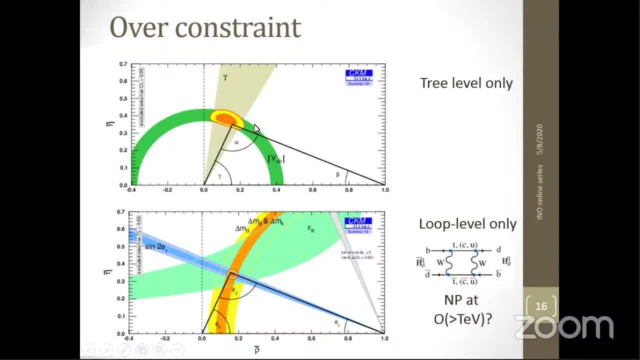 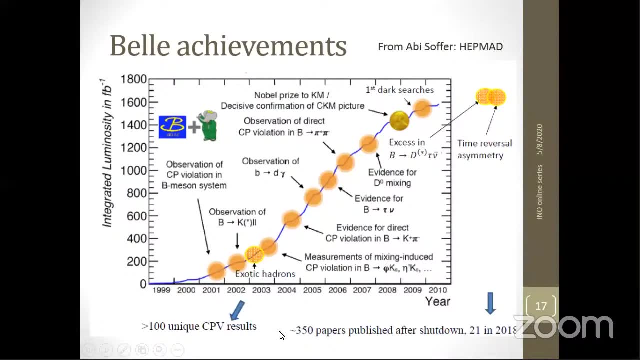 So with the unitarity triangle now we want to try and constrain this as well as possible. So Bell had many achievements. aside from this CP violation measurement, There are various rare decays observed- lateral weak penguins- which I won't talk about. 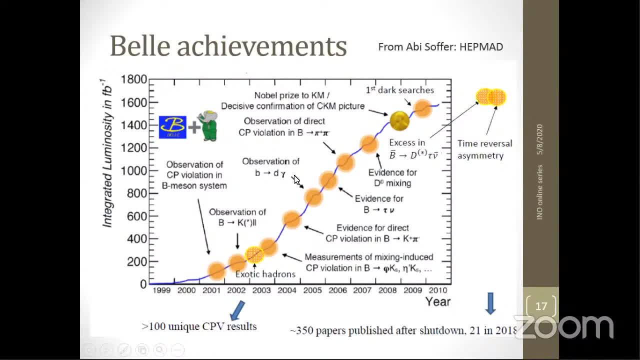 That'd be a nice talk for someone else to give in this series. Then there were things to do with charm, physics, demixing and also discoveries of many exotic hadrons, the so-called XYZ states, that don't fall into the normal pattern of mesons that had previously been seen. 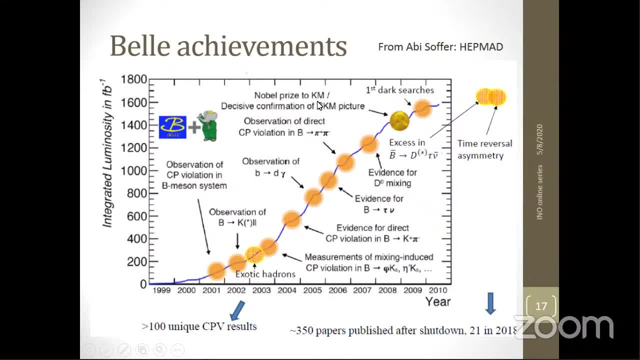 And because of the confirmation of the CKM picture of CP violation in the standard model. Kobayashi and Muskawa got the Nobel Prize here in 2008.. So it has been very successful. Hence the whole idea of Bell 2 is to basically do more. 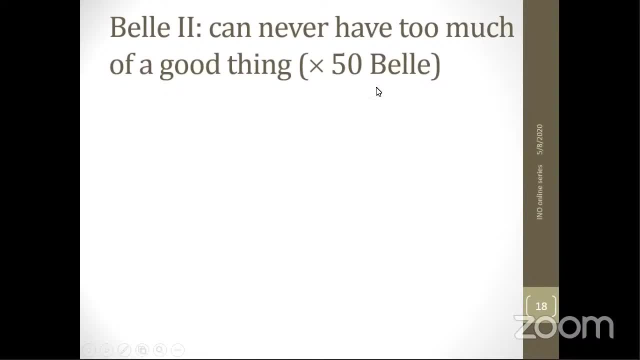 You can never have too much of a good thing. And Bell 2 is the idea of having 50 times more data than Bell, So collecting 50 inverse atta bonds to measure B-physics and charm physics and other observables very precisely. 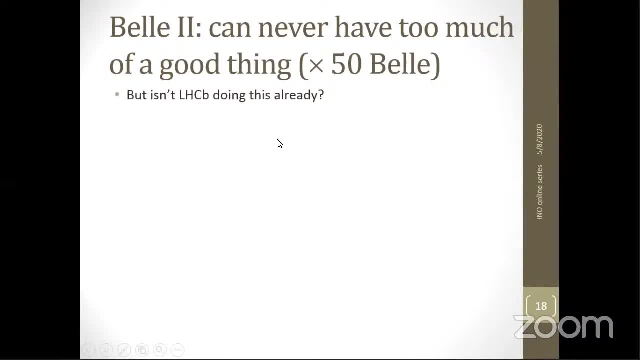 But a question you can ask yourself is: isn't this what LHCb is doing already with their B-physics measurements? So if you look at the iCHEP results, many of the highlights are coming from LHCb this year and in previous years. 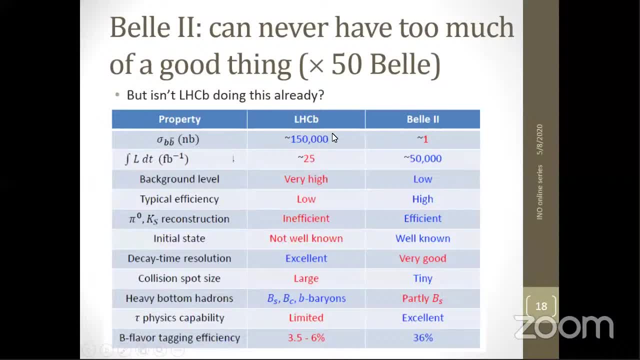 But the big difference between Bell 2 and LHCb is that the E plus, E minus environment allows certain advantages in terms of the reconstruction. So LHCb has the advantage of statistics. So the cross-section for Bb-par pair production at the LHC is enormous. 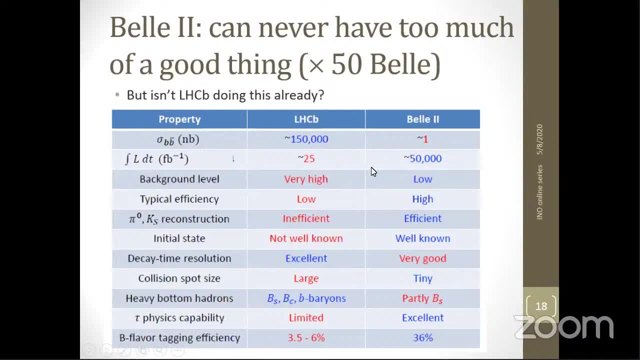 It's five orders of magnitude larger than it is at Bell, But this can be partially compensated by larger luminosities. This is 50 inverse atta bond number. But also because of the threshold production the background level is relatively low. We also don't have to run a real-time trigger. 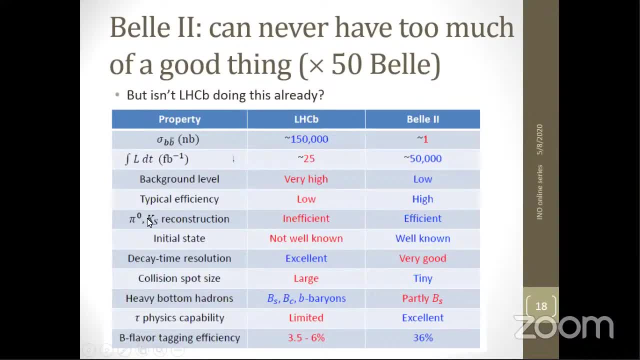 So our efficiency is very high. We can reconstruct neutral particles in our clean environment- pi zero and k-short very, very well, which is more difficult. at the LHC We have this initial state kinematics. We don't have as good decay time resolution because these bees are boosted such that they fly millimeters often before they decay. 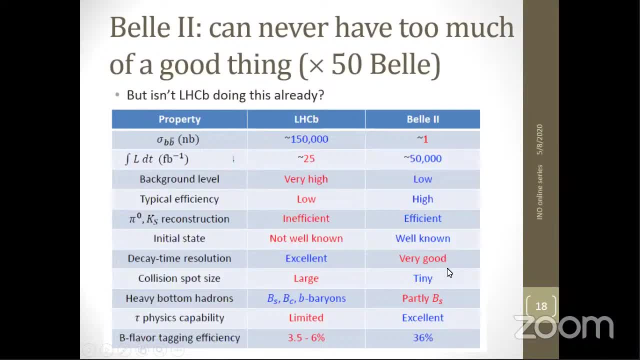 So you can measure their vertices very well. We have a very small beam spot, as I'll show you in a little bit. LHCb has the advantage that they generate all types of B mesons, particularly Bs mesons and B baryons, whereas Bell 2 will produce a few Bs mesons. 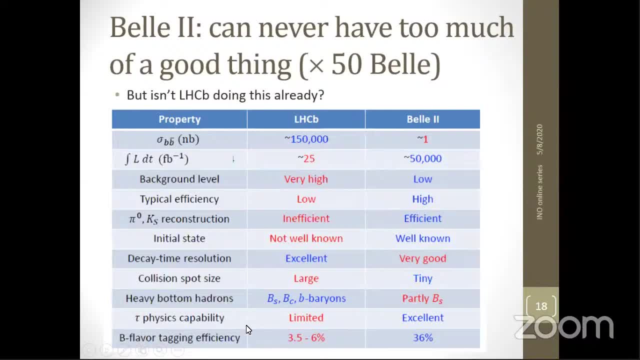 But it's mainly B mesons, B plus and B zero. LHCb cannot do tau physics very well, but Bell 2 is a tau charm factory as well, And there's also this advantage in flavor tagging when you do time-dependent measurements because of the clean environment and this quantum correlation. 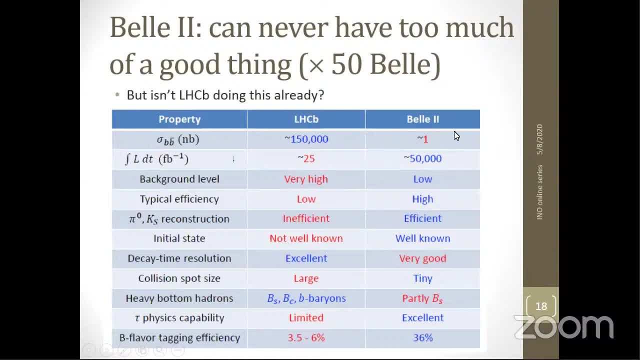 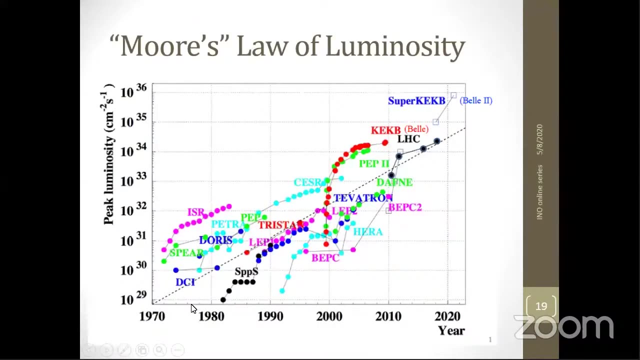 So that efficiency is an order of magnitude larger. So this allows Bell 2 to be competitive, even though it's got a statistical disadvantage to LHCb in terms of the production Of B and B bar pairs. So where Bell 2 leads the way in terms of accelerators, 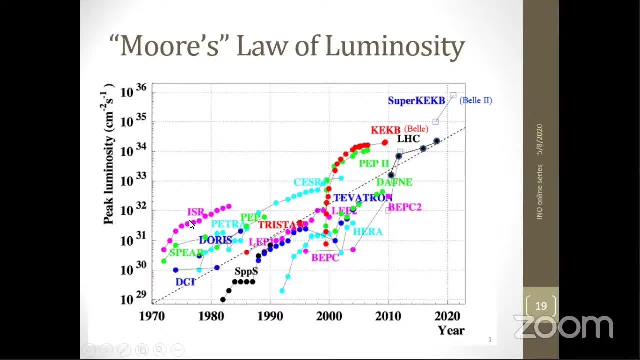 Is in is instantaneous luminosity. peak luminosity here, Where it's trying to achieve something around 10 to the 36 inverse centimetre squared per second, which is very much higher than the LHCb, the luminosity-upgraded LHC, and any previous accelerator. So to understand how Bell 2 can, 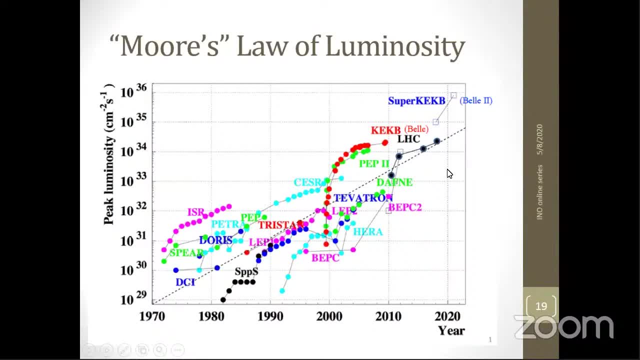 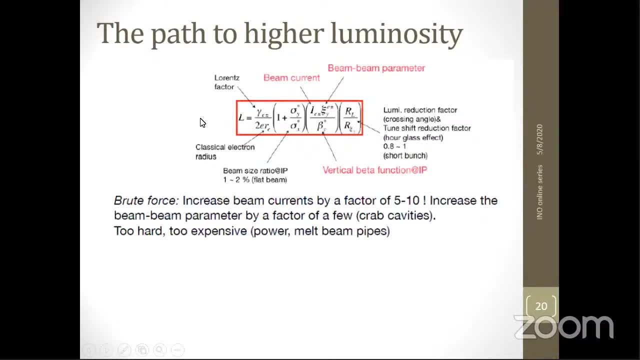 do its physics. we first have to understand the accelerator super Keck B. So this expression, which is rather more complicated than the expression you normally see to describe the luminosity of a collider, introduces the parameters of interest. So there's the usual geometric 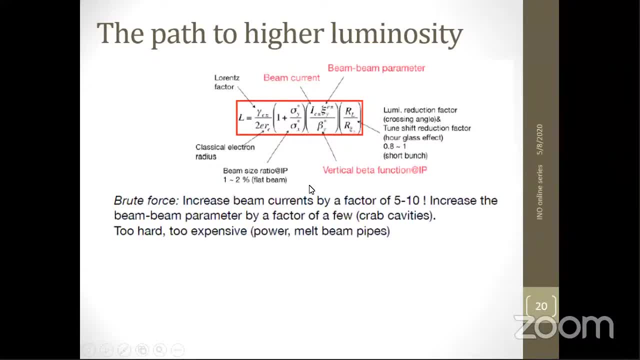 factors, but I want you to focus on these red parameters that I've labeled here So clearly. one way to increase luminosity is just to pour more electrons and positrons into your machine. So you increase the currents And then you can make the beam spot very, very small. So you're 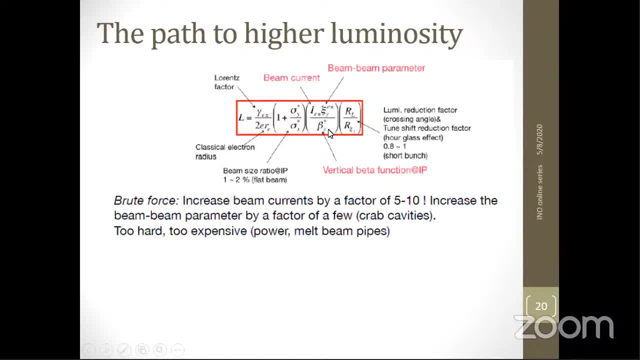 cramming all that current into a smaller space to increase the luminosity. And that's this beta star parameter. It's essentially a measure of how well-focused your beams are, But this is in some ways complicated, So we're going to look at this in a little bit more detail, But this is in some 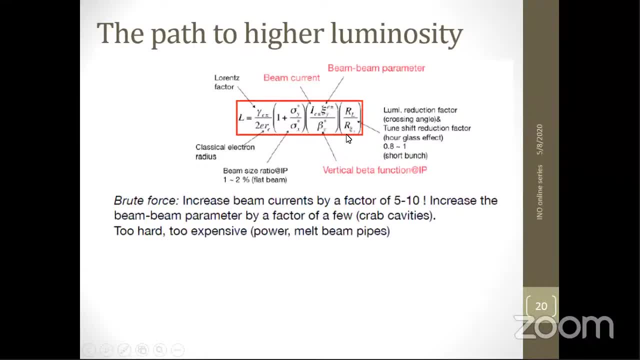 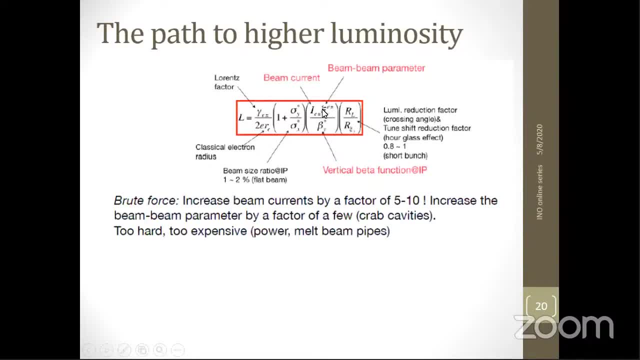 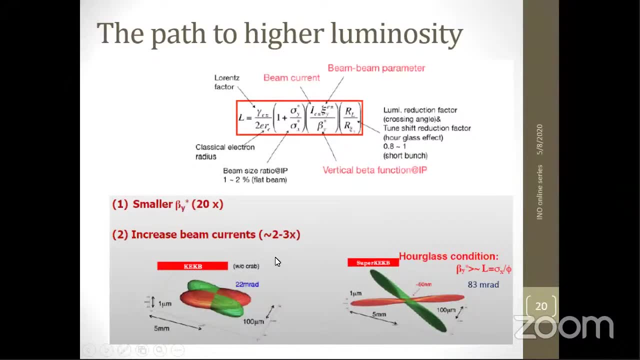 problems, And this parameter you have to try and balance in some way as well. So how Bell 2 tackles this problem is not to just blindly increase the currents as much as possible, because that leads to a lot of synchrotron radiation in an E plus, E minus machine which 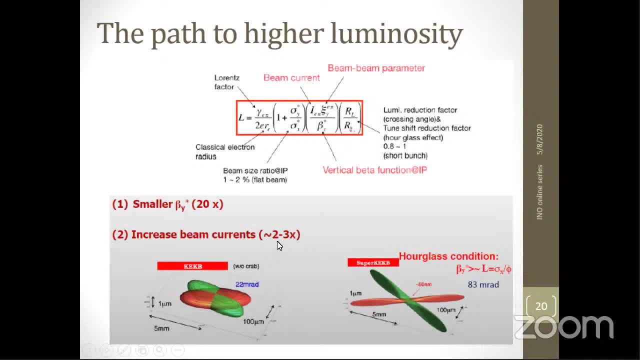 will damage the beam spot, But it's also going to increase the current as much as possible because that leads to a lot of synchrotron radiation in an E plus, E minus machine, which will damage the beam pipe and the detector as well, but to try and squeeze the interaction point down to be as small. 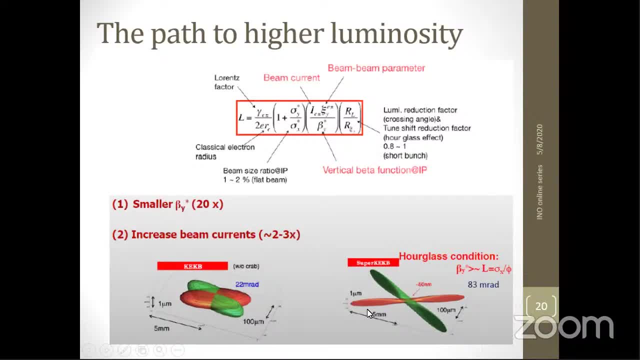 as possible by this beta star parameter. So this led to what's called the nanobeam scheme. So this is Keck B. the accelerator that worked with Bell on the left side- And these are the typical bunch- is crossing one another. So these green and red are the electron and positron bunches. 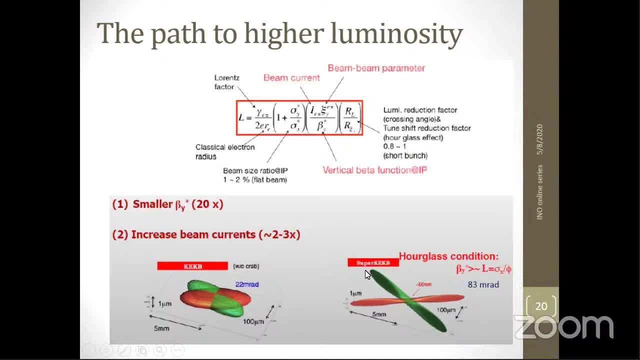 And for Bell 2, the super Keck B have squeezed their bunches in a clever way- so-called hourglass conditions, so that they are pinched at the centers that cross to give a very small beam spot And this leads to this very 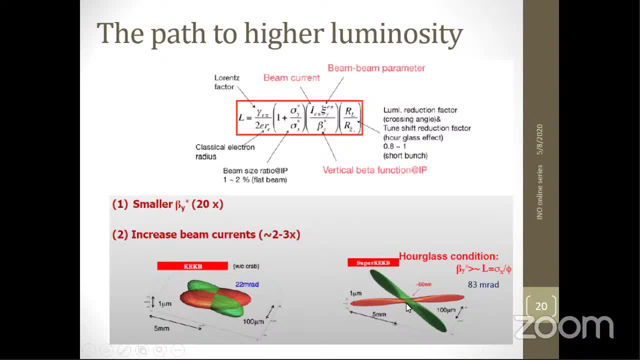 small value of this beta star parameter which leads to the high luminosity. So this has been done and it reduces the size of the interaction region considerably. So, coming back to this beam-beam parameter, it's not just all about focusing on the beam, it's about focusing on the 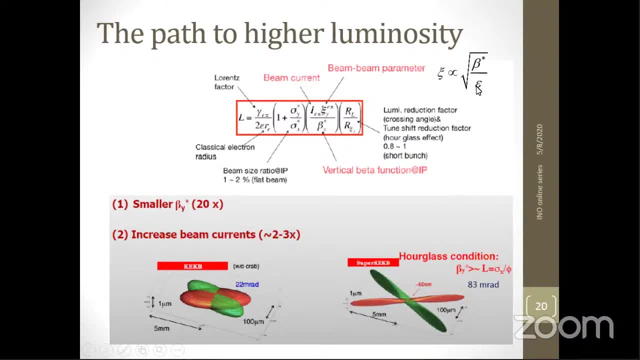 ibaens better. You also have to worry about this epsilon, which is the emittance of the electrons in the in the collider, and you, and if you can reduce the admittance, you will increase this beam-beam parameter and increase your luminosity. 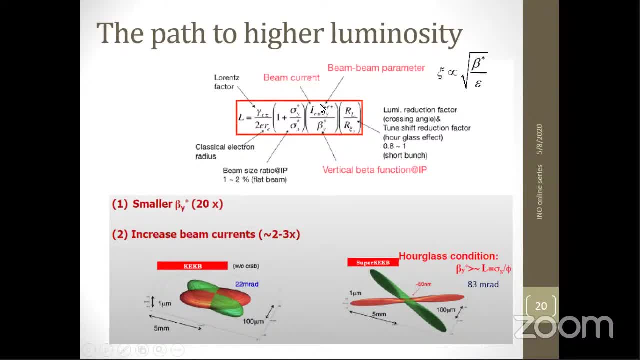 So you also depends on beta star. So there's an overall beta star square root dependence and you also have a dependence on the emittance as well. So it's a matter of squeezing the emittance and and squeezing the beta star parameter as well. 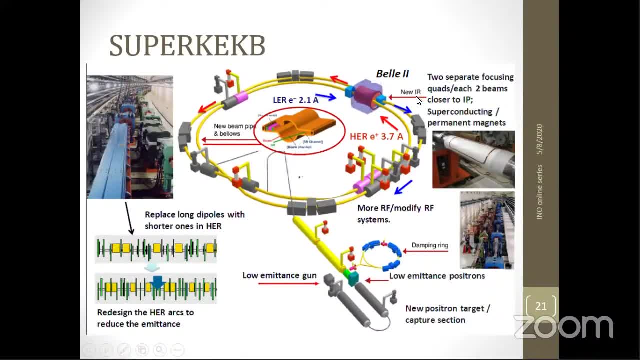 So this led to a major upgrade of SuperKetB, not only the final focus here at the BEL2 experiment, but also in all the components around to deal with the larger currents and also to produce as low emittance beam as possible. So the bending magnets, the dipoles, were replaced. 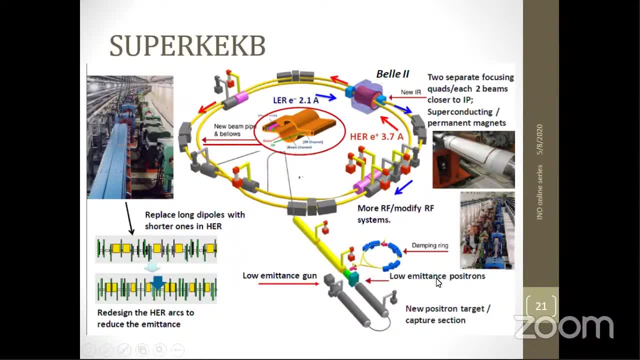 linic was replaced and the RF was replaced too, So there are two separate rings here for the electrons and positrons, given that they have different currents and different energies, And this is this two twin accelerator scheme that was used also by KetB as well. 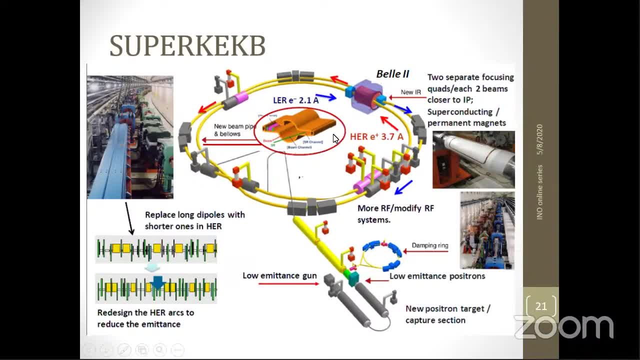 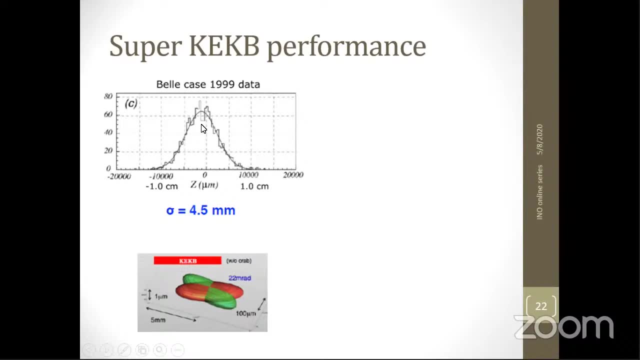 And this is the redesign of the beam pipe in a way that the much higher currents don't melt it, So they use these kind of calipers and cooling to do that. So this performance has already been proven in terms of reducing the size of the interaction region. 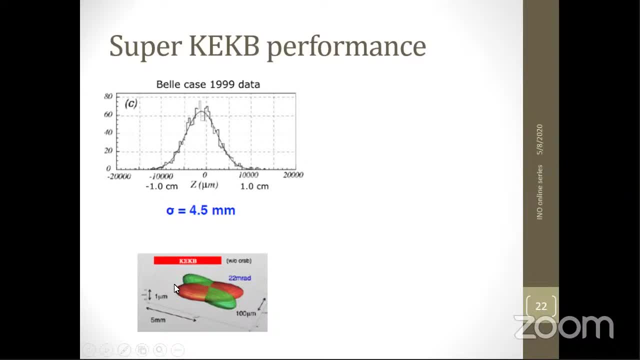 So this is a plot showing the longitudinal spread of the interaction point in our E plus, E minus collisions at BEL. this is from early BEL data And it was roughly half a centimeter across, Whereas the same measurement at BEL2, even before much tuning of the beams gone on- has been shrunk down. 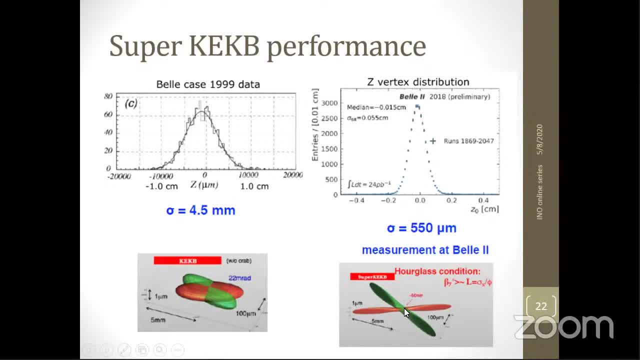 by an order of magnitude. So now this interaction region where the two beams overlap with one another is down to around half a millimeter in length. So this is an early proof that this hourglass scheme was giving what we were expecting in terms of the interaction region. 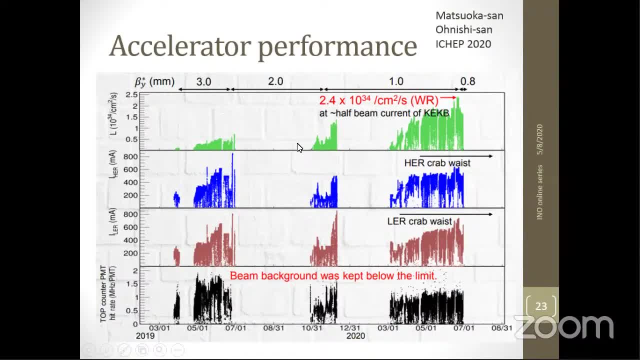 So we've gone on from 2018 and the highlight from the accelerator this year is that a world record was set For the instantaneous luminosity of the super Keck B accelerator of 2.4 times 10 to the 34. So it's still some way off the design luminosity. 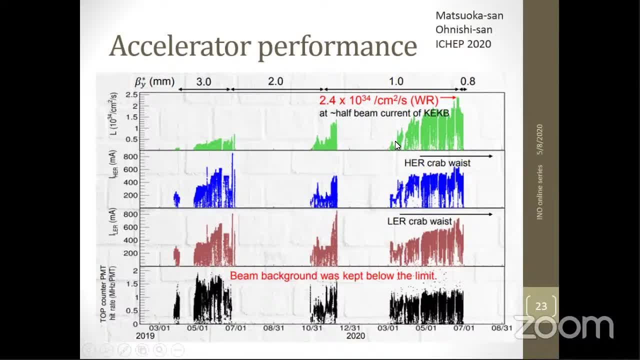 but this is very much falling in line with the plan that we have And you see also the challenge here. this is in the bottom, the black points. The more current you put in and the harder you squeeze the beams, you end up with spurious backgrounds generated. 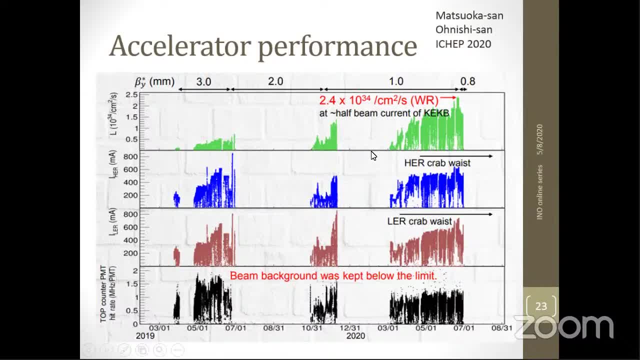 by the synchrotron, radiation and other beam effects. So it's a constant challenge to keep the beam background at a low enough level so that the detective can run smoothly. So this high background level has also been managed to be kept at the same late. 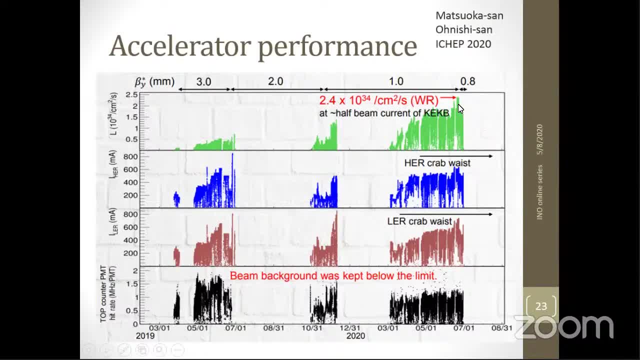 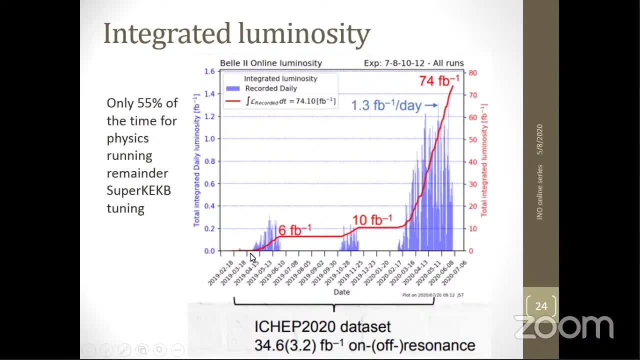 even as we're increasing the luminosity, which is key for us to be able to operate the detector. So, in terms of the integrated luminosity, there was a small amount of running last year. We've got six inverse femtobarns. 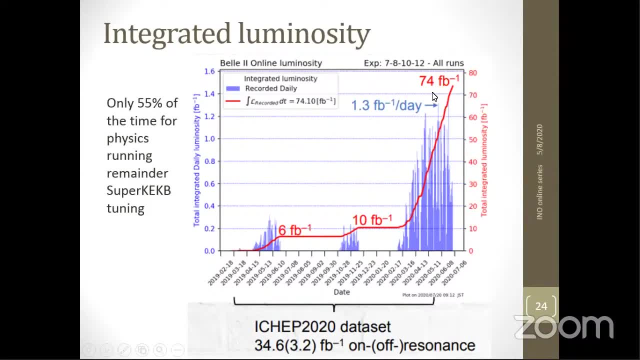 and later in the year there were additional 10, but this summer it's really picked up And we've now got a sample of 74 inverse femtobarns, of which around half has been used for measurements at super, presented at ICHEP. 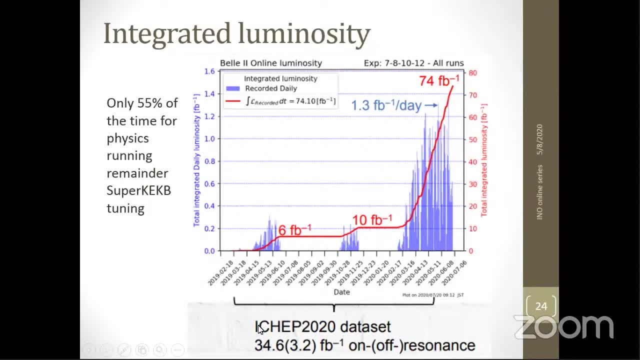 But of course this is very little compared with 50 inverse femtobarns, so we're still on target. but this allows us to prove both the detector is working and that we're moving in the right direction, And also it should be noted that physics collection 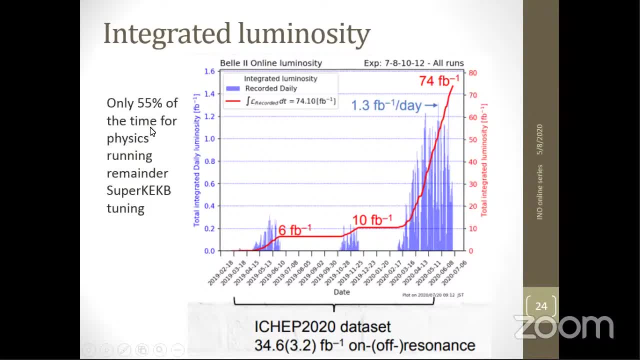 is only roughly half the priority at the moment. Much more time is spent during the day And during the night we get physics data during the day. people are constantly working on trying to improve the parameters of the accelerator to increase this instantaneous luminosity number. 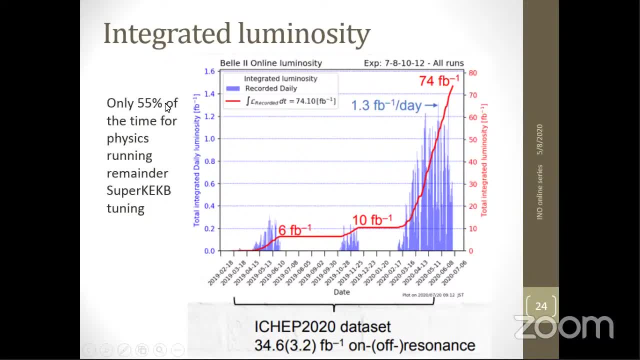 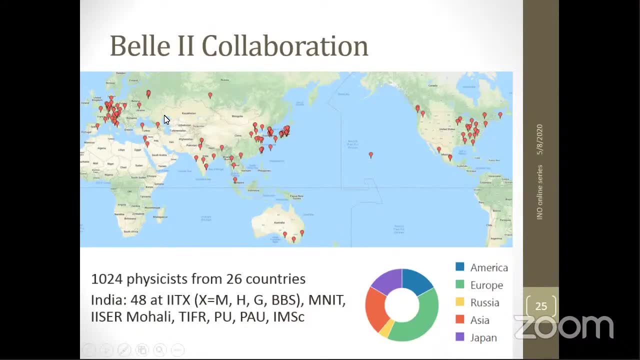 So that's still. the main target at the moment is to improve the accelerator performance. So, talking about the BELL 2 collaboration, briefly now just the sociology of it all. It's a large experiment, over a thousand physicists now from 26 different countries scattered throughout Europe. 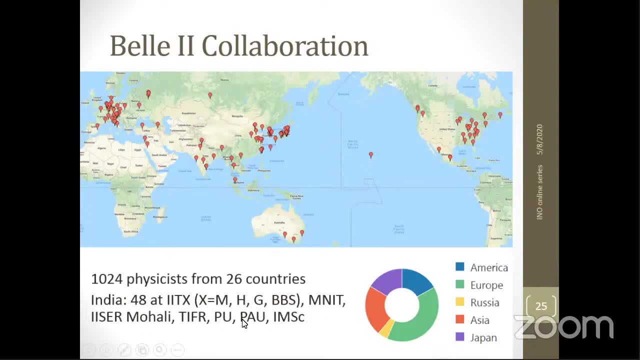 Asia and the Americas, as well as Australasia, Australia, And there's around 5% of the collaboration is from India. There are four IITs involved: There's MNIT, Jaipur, ISA, Mohali, TIFR, Punjab. 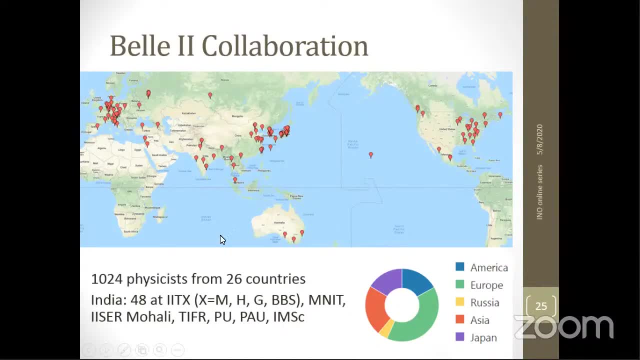 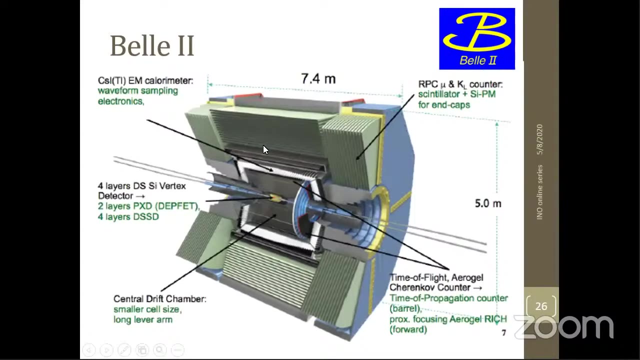 Punjab Agricultural University and IMSC. So we're a large contributor to BELL2, and we've been members of BELL before BELL2 as well. Moving on to the accelerator- sorry, the detector, This is reused parts of BELL, particularly the solenoid. 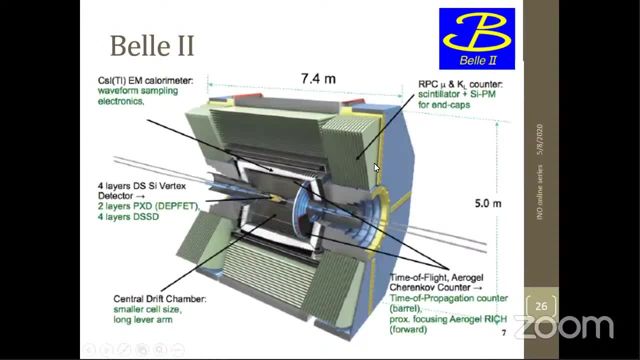 and the flux return, as well as the wire chamber, is very similar design, though it's been slightly changed in size so it was restrung. Sorry, the electromagnetic calorimeter- the crystals- have not been replaced. I thought it was very expensive. 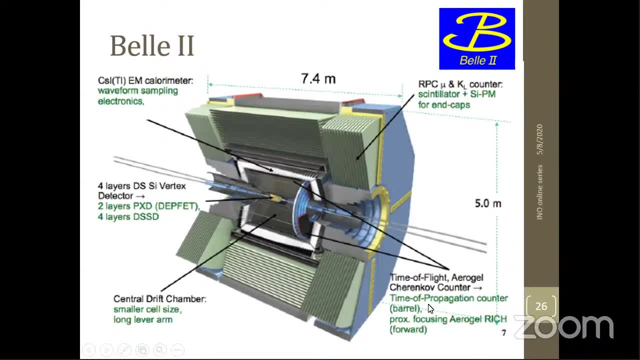 But we have a new silicon detector and we have better particle identification using something called- so this time of propagation counter or top counter, which I'll talk about some more, And also I'll talk a little bit more about the silicon. So this is the BELL2 detector, very similar to any general purpose detector. 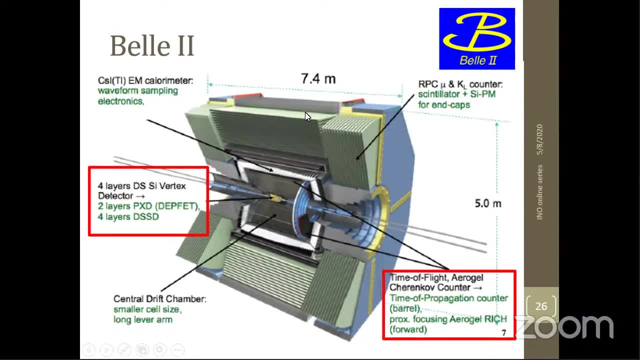 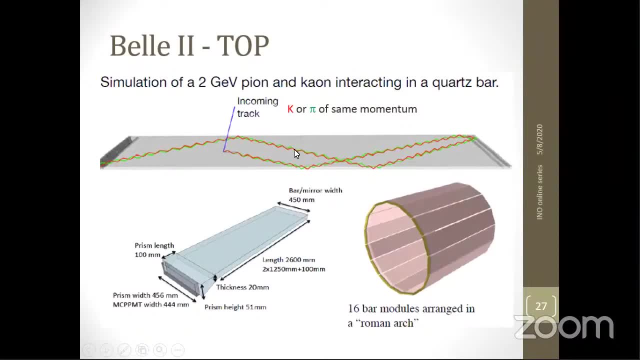 with the inner tracking electromagnetic calorimeter and then a neuron filter along with some Hadron ID. So this time of propagation, or top counter, uses Cherenkov radiation to differentiate between, principally, pions and kaons. It uses a quartz bar, which is this gray slab you see here. 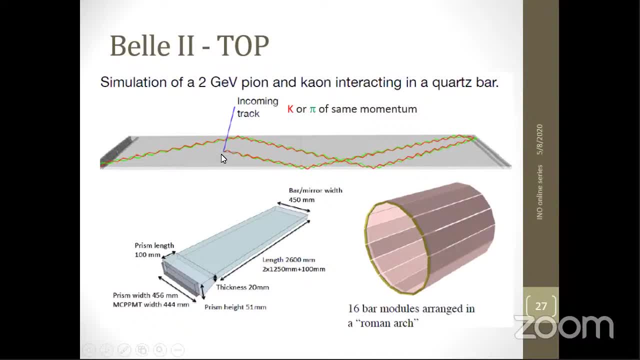 and the track that comes through. it will radiate Cherenkov radiation if it's of high enough momentum, such that its speed is greater than the speed of light in that medium. But the angle at which it comes out will depend on its speed, not its momentum. 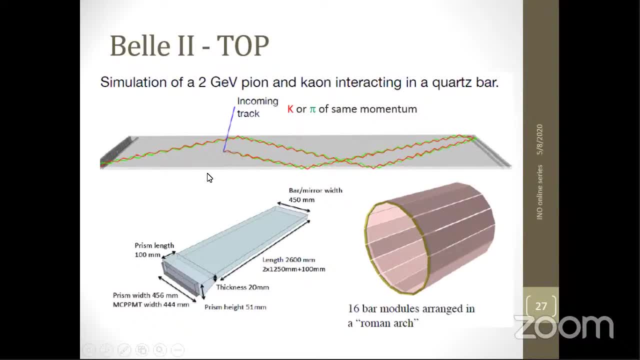 So the same momentum, kaon and pion- will produce different angled Cherenkov radiation. So you then use total internal reflection within the quartz bar to bounce the photon forward and back until it reaches an array of filter multiplier tubes- well, microchannel filter multiplier tubes at one end. 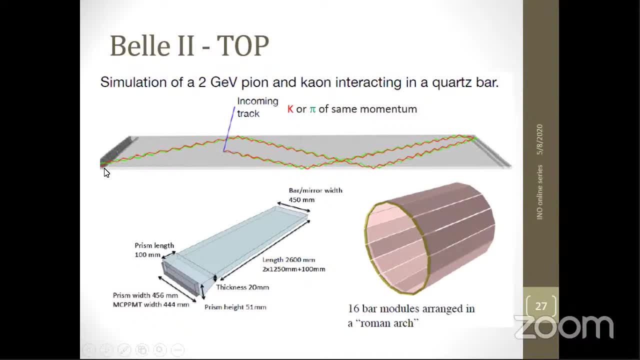 And using timing, as well as the spatial precision at which you see the photons, you can work out where the photon came and the distance it came from, And you have 16 such bars encircling the interaction region, And you can then use this to identify pions and kaons. 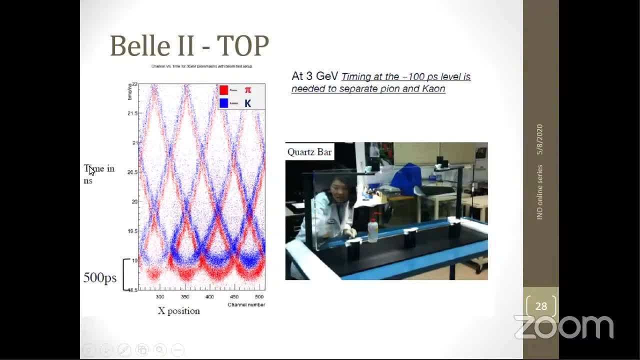 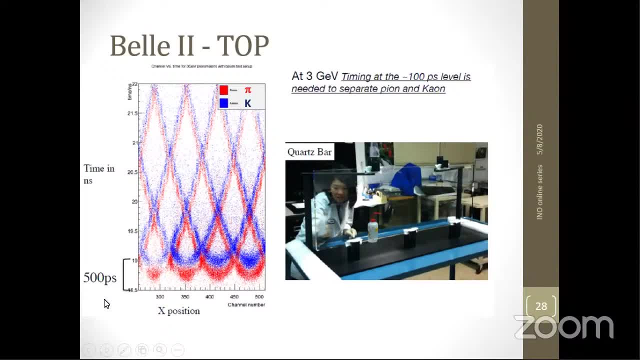 And if you have a pion, you get the red pattern for two coming through a pion. So, as a result, we can look for pions that are in the same place in the same momentum. So as long as you have 100-per-second resolution. 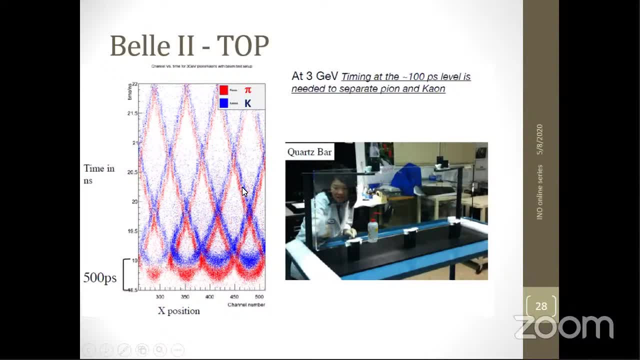 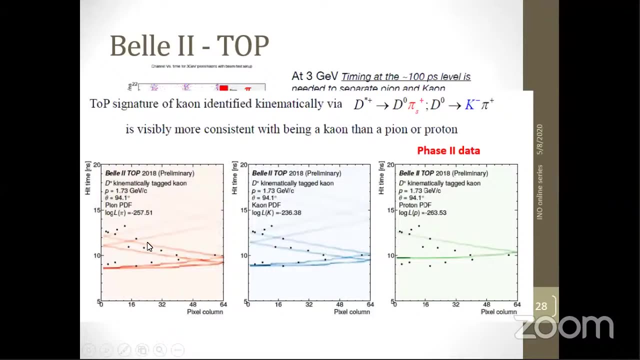 you can be able to separate these different particle types as they go through and be able to identify pions and kaons. So this is not just a, This is now a working device. So this is some early data where you look at this pattern just for a single event. 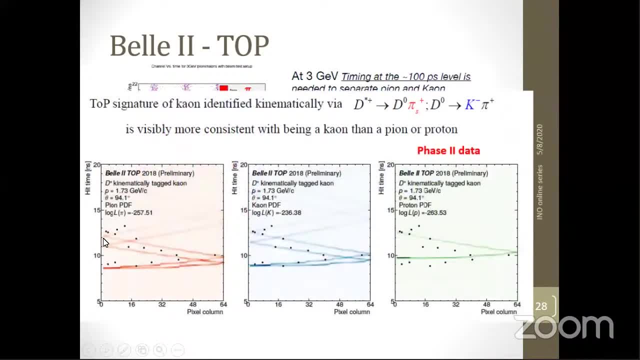 This was taken over many, many Monte Carlo events. This is a single event And you can see the pattern of hits of the photons in terms of the channel and the timing, And you have the hypothesis of whether it's a pion in the left kaon or a proton. 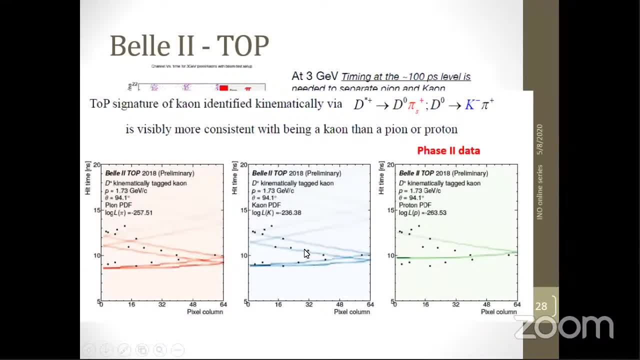 And you see that for the pion, for the kaon, it matches up very nicely with where you would expect the photons to be, which is not the case for the pion and the proton, And hence you're able to identify pions and kaons. 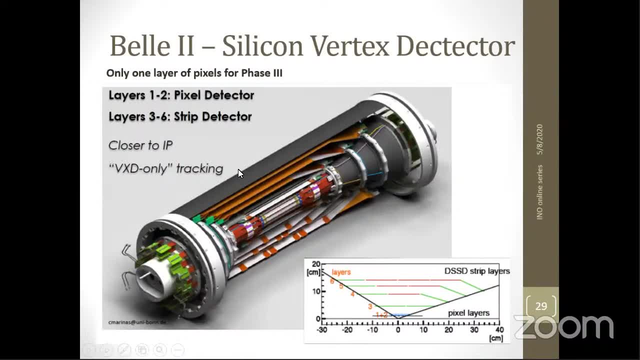 The second instrumentation highlight- before I move to the physics highlights- is the silicon vertex detector, which has two innermost layers of pixels which at present it doesn't have. So it's actually this is the one bit of the detector that's still missing and that will be installed somewhat later. 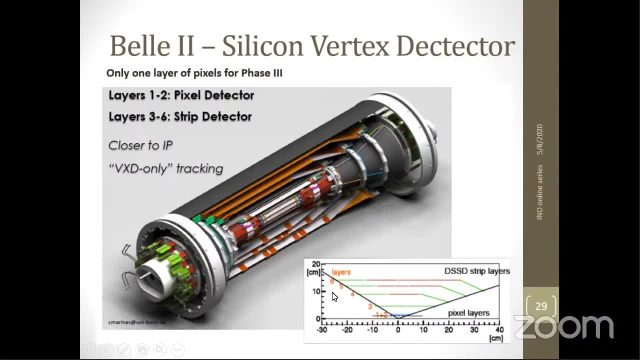 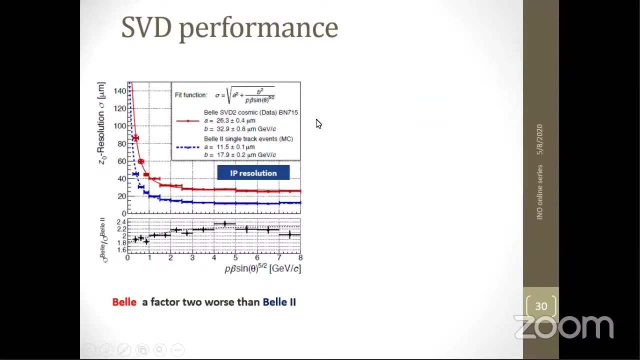 And then there are four layers of double-sided silicon strip detectors, Of which one- layer four- was constructed by Indian groups led by TIFR, And this detector has much better impact parameter or decay vertex resolution than the Bell silicon vertex detector, And that compensates for a slightly smaller boost that we have now between the two beams, which is required. 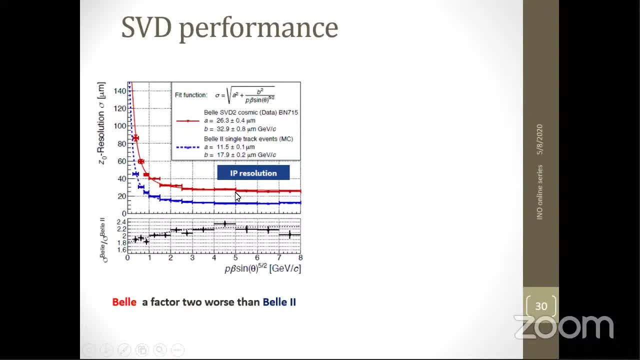 So this is the resolution of the impact parameter related to the vertex reconstruction. Red is Bell, blue is Bell two. And you see there's a significant difference as a function of the momentum of the particles. Further you can do standalone tracking of very low momentum particles, which is much more efficient than Bell. 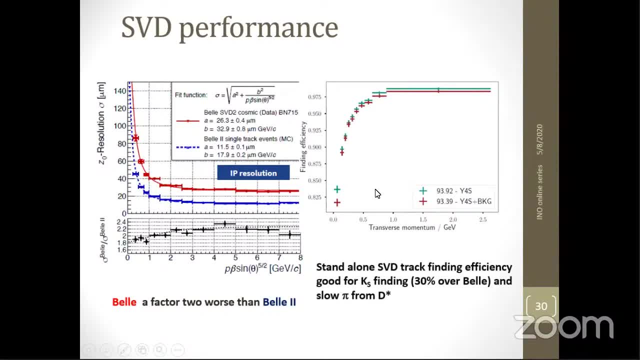 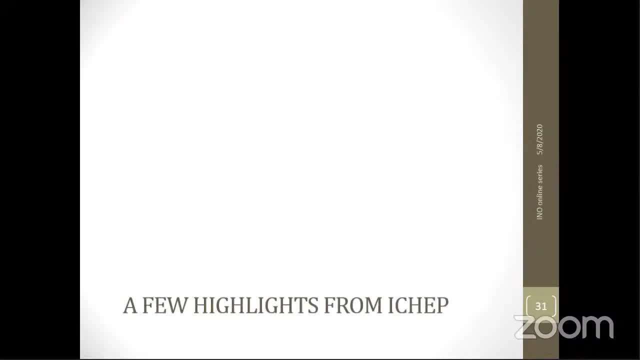 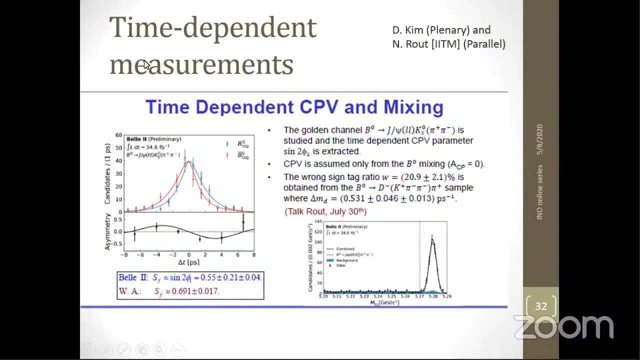 This is showing for low momentum pions coming from charm decades. So I will conclude the talk with a few highlights from iChip and then one physics prospect. So I've talked about time-dependent measurements of sine two beta or sine two five one, And the highlight from Bell two is that we've had our first measurement of that this year. 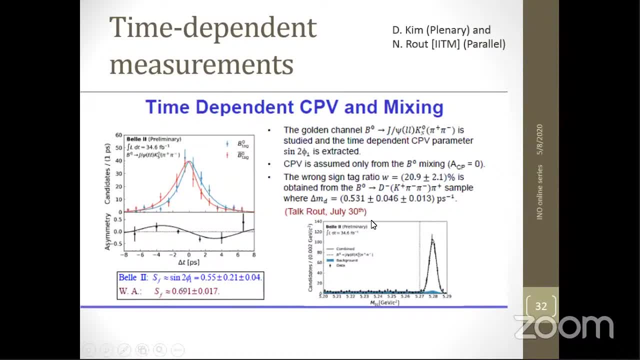 So this was shown last week by my student from IIT Madras, Though she's working on something else. she showed the result. So this is again just the benchmark. So you can see that. You can see that shows this delta t difference and the blue are b zeros and the red is b zero bar. and if you plot, 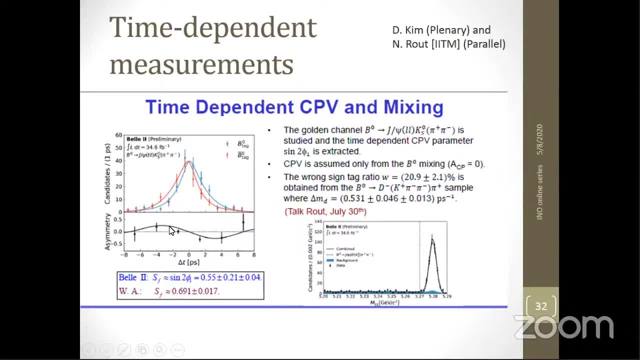 the number of decay that you see as a function of this time difference. you see there's a clear asymmetry and if you fit this asymmetry you get a value of sine two beta which is compatible, within the statistical uncertainty, with the world average, but it's a lot less precise. it's a order of 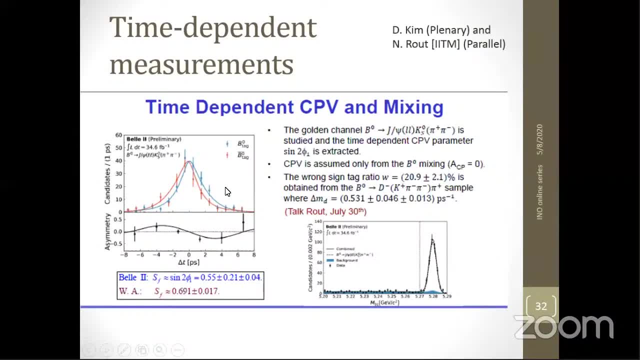 magnitude less precise but of course this will improve as our statistics increase. also, it highlights a very clean environment in which we worked. here is the essentially the B mass peak that we have. this is centered at the mass of the B and you see there's a very low level of 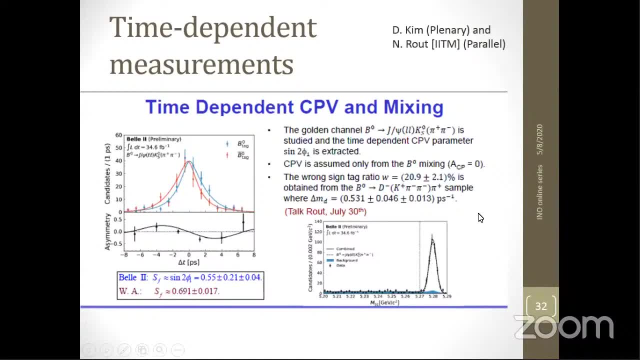 background underneath the signal for the J spy K short that's reconstructed. we aren't quite yet at our optimal tagging efficiency, just in terms of how this measurement was done, and that will again improve as we make further measurements, use more information to do the tagging. that's one of the highlights of the B mass peak that we have. this is centered at the mass of the B and you see there's a very clean environment in which we worked. here is the essentially the B mass peak that we have. this is centered at the mass of the B and you see there's a very clean environment in which we worked. 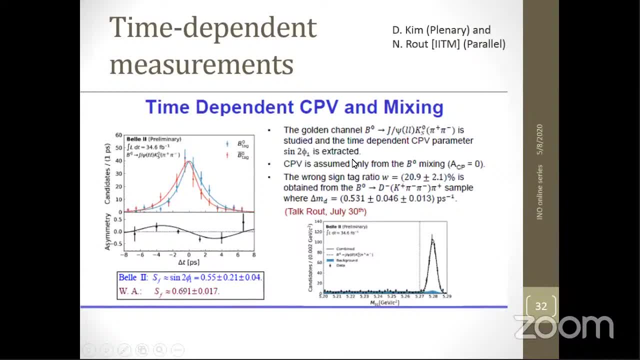 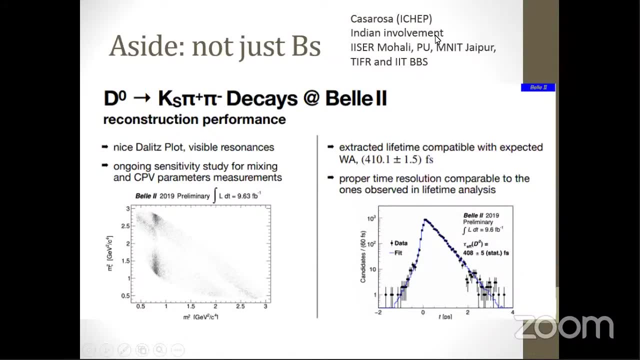 highlights from I CHEP. so this is very much Bell 2 working, as we would hope. another highlight is related to charm physics and again there's strong Indian involvement from these institutes in charm measurements of Bell 2. many of the plots that were shown at iCHEP came from these groups. 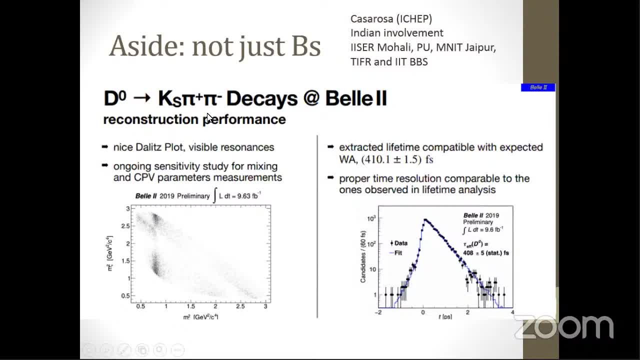 this is for a decay of d0 to k- short pi plus, pi minus- which currently from LHCb measurements, provides the best measurements of mixing of d0 meson and these parameters are sensitive to physics beyond the standard model because again it's a mixing, so it's a loop that's involved. so this is a three-body decay, so you have a Dalitz plot. 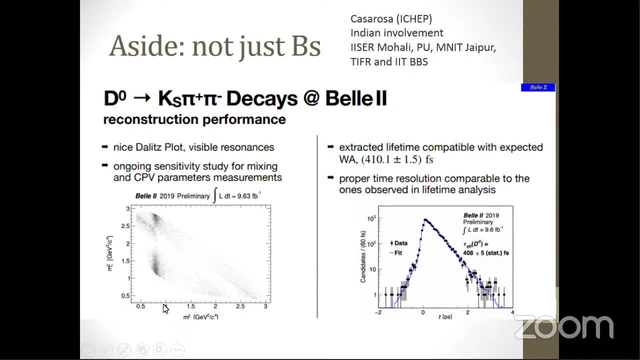 where you look at the invariant mass of the k short with one pi on the pi plus on the horizontal axis. sorry, it's pi minus on the horizontal axis and the pi plus on the vertical axis and if there were no resonances involved you would have a uniform distribution. but when you have resonances, 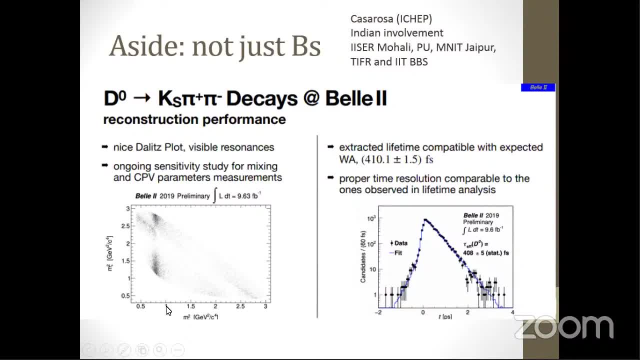 like here, you would have a uniform distribution. but when you have resonances like here, you would have a uniform distribution. but when you have resonances like here, you see a k star, you get a band and the structure of the band actually tells you the spin of the particle. 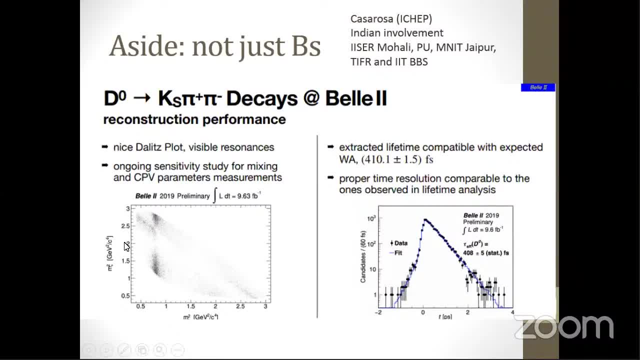 you see on the diagonal a Rho meson as well. so this is real data- with only 10 inverse venture bonds. so you're getting many, many decays. so what is interesting is to measure mixing. you must do things in a time dependent way and here shows the lifetime distribution coming. 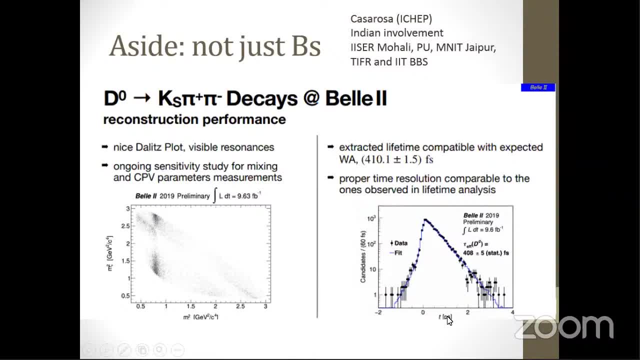 from these d to k short pi pi decays, and this is measuring a femtosecond, 450 second lifetime of the d zero and you you see that the signal has this extended lifetime like linear distribution on this log scale for the exponential decay rate that you'd. 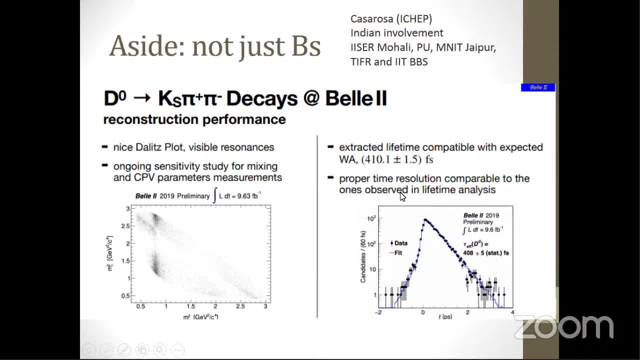 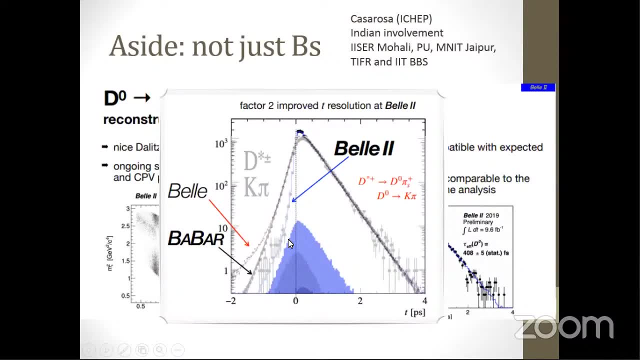 expect for a long-lived particle. so this is again showing the the the good performance of the detector, and also we can see the vertex detectors performing much better than bell. so this is the different d data, but you have the bell data. compared with what you had at bell and also at. 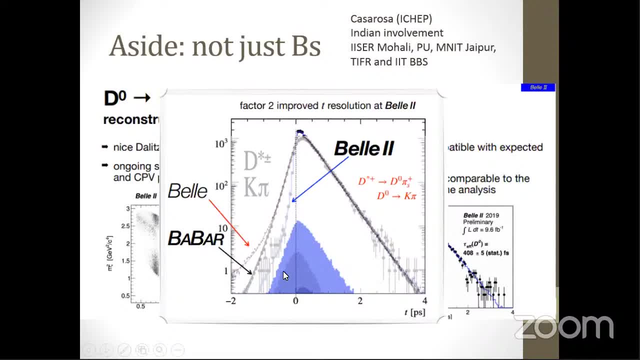 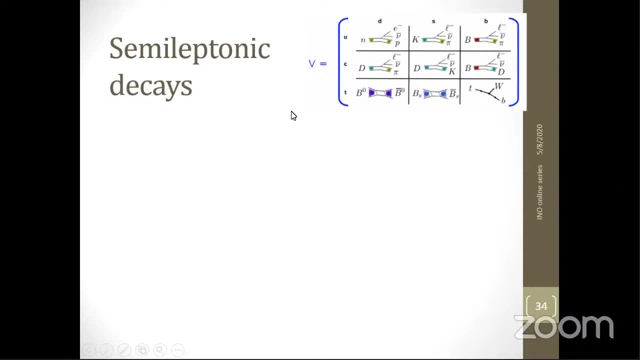 babar, and you get a much smaller tail on the negative side, which is just to do with the resolution with which you measure the lifetime. so that factor of two difference is really being observed in the data. now, moving to the other main highlight of bell 2 at this year's ichep: 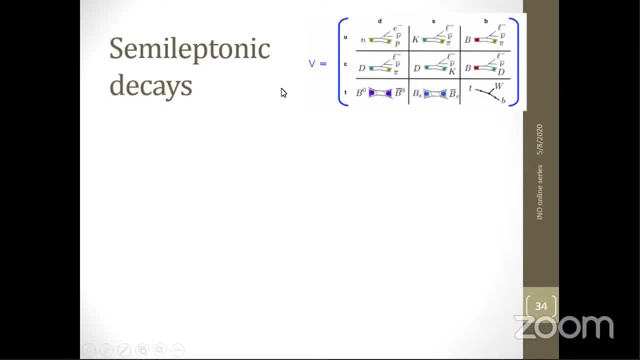 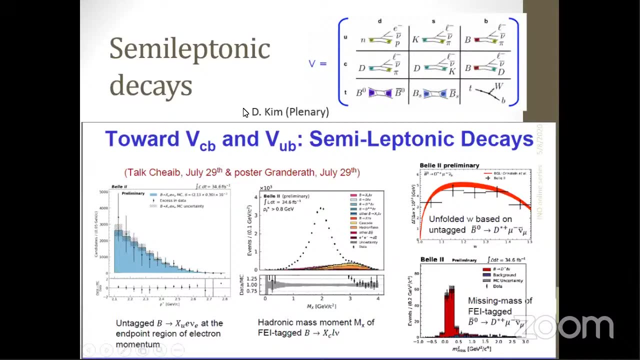 conference was measuring semi-leptonic decays and i'll explain more about what that is and why that's very interesting in my highlight, in my prospect. but here we measure the magnitude of ckm elements by either looking at the vub decay- that's related to vub- with a 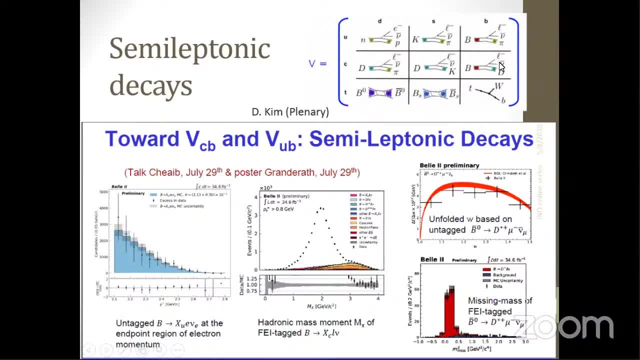 b going to pi on two leptons or a? b going to a charm into leptons to measure vcb and you can measure the part by looking at the very highest momentum electrons that are produced, because there's more phase space available when you're going to a lighter pion, so you get higher momentum. 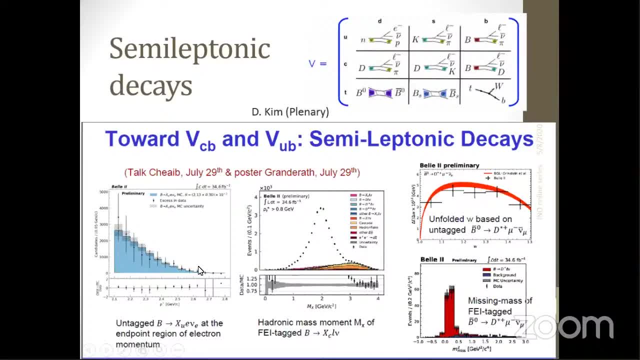 electrons, which allows you to measure vub. this is the first measurement of that from bell 2 and you're also being able to look not just at the electroweak part, the vcb measurement, you can also study the qcd of the b2d. 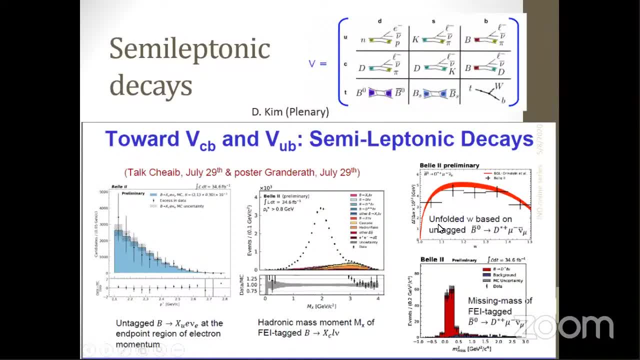 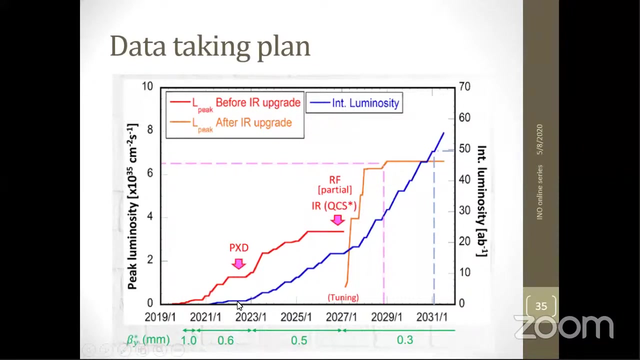 and this is the desired energy distribution using a centripetal. So Bell 2 is working well, but our luminosity is still very small compared with Bell And our next goals are shown on this slide, which shows the plan for Bell. a SuperCat could be running in the years ahead, So this has changed a bit recently. 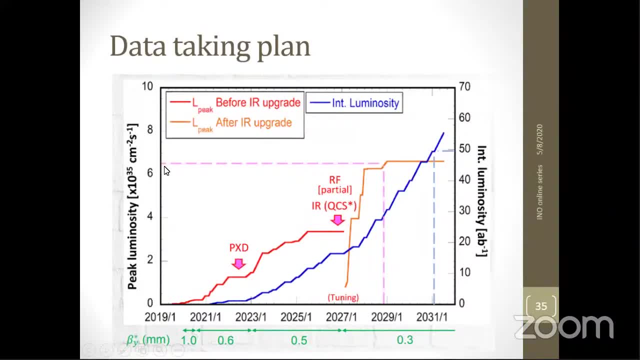 So we've actually downgraded where we expect our peak luminosity to be, to be around 6.5 times 10 to the 35. And this is the blue line. Sorry, the red line is showing this slowly increase over time. 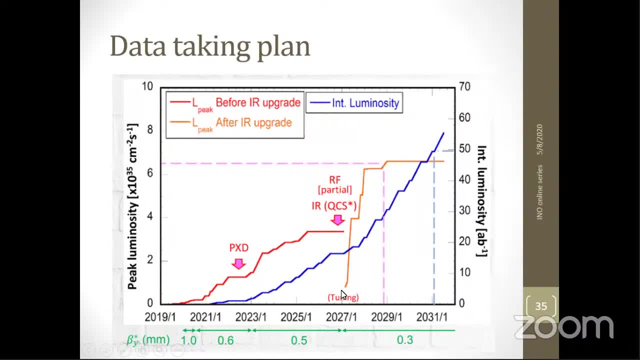 Then we're going to upgrade our interaction region and then we'll get to the very highest values in around the second half of this decade. And over time we'll just slowly accumulate for the next 10 years a data set corresponding to 50 inverse Atterbarns. 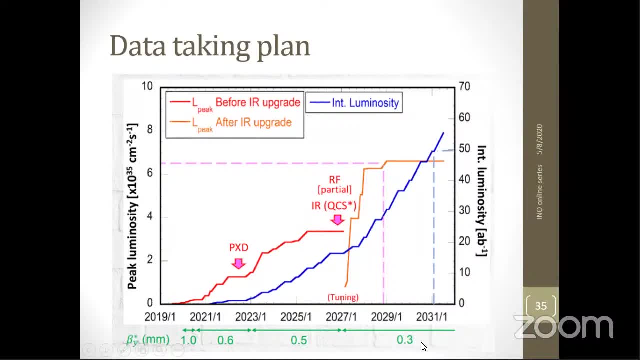 as we slowly squeeze down this beta star parameter and get the very highest instantaneous luminosities. So one point to look out for along the way is here in the blue line, which is the integrated luminosity. When we get around five inverse Atterbarns we will start to make some very competitive measurements in around 2024. 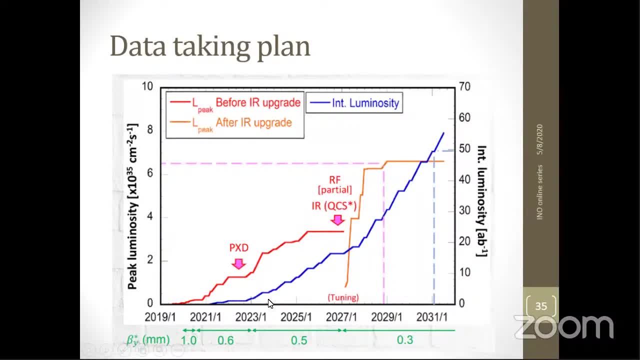 where we may be able to see new physics contributions. So it's a long game, as it is with any accelerator or any detector project, But we are now on the road to getting some results. Thank you, And we hope to see some very interesting results in the next few years with Bell 2.. 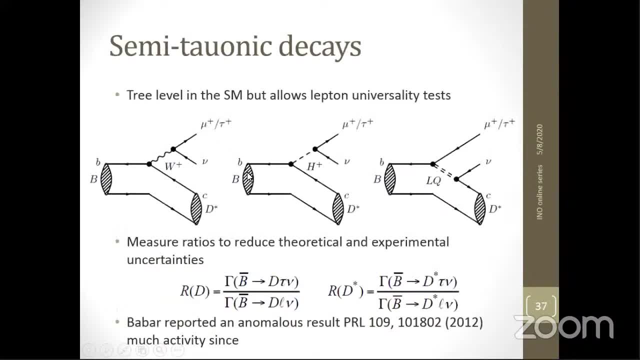 So, as in my example, which is related to semileptonic decays, I'm going to talk about a very hot topic in particle physics, which is the so-called B anomalies related to lepton universality violation. So, naively, once you've taken into account, 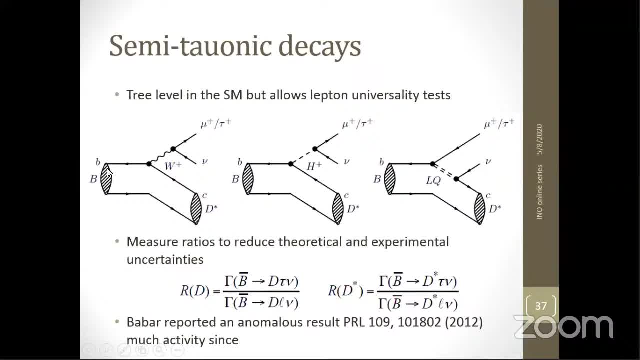 the same mass of the tau and the mu, you would expect the rate of B to D tau nu and B to mu nu to be exactly the same because of the universality of the weak coupling to lepton. However, it's possible with new physics, such as a charged Higgs or a lepto quark, to change this pattern. 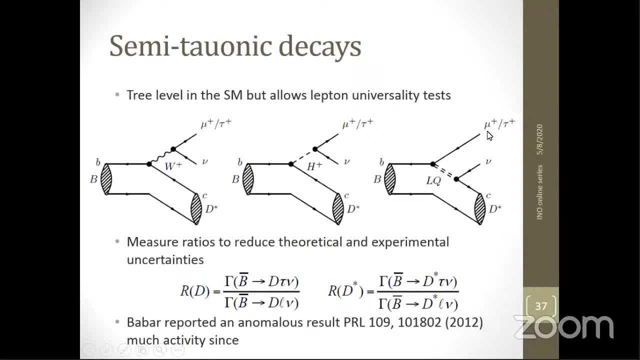 And that would predominantly or more likely change things for the third generation, the tau than the mu. So this is an interesting place to look for new physics and see if there's any violation, This lepton universality. So what you measure is the ratio of the B to D tau nu, with B to D L nu, where L is E or mu. 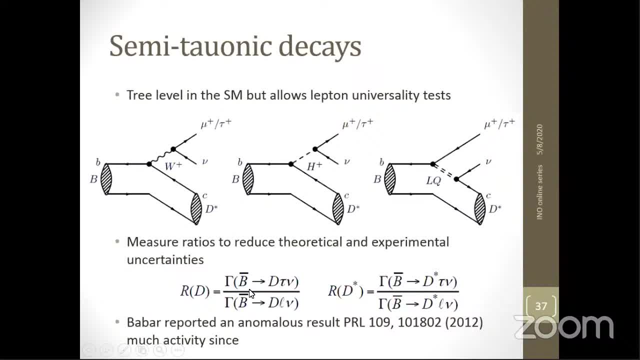 And this can be very precisely predicted in the standard model, assuming lepton universality. And you can do this for both D tau nu and D star tau nu, And this has been a hot topic for a long time now. The first result was in 2012.. But why this is interesting. 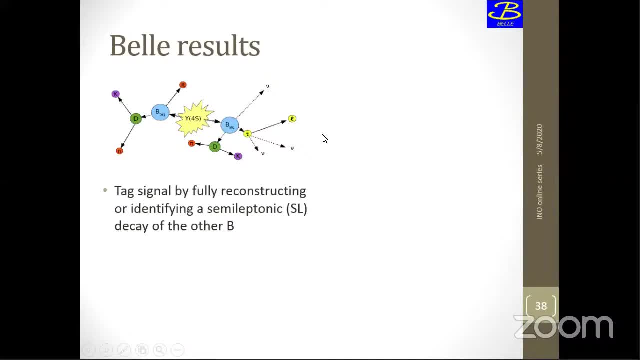 Because there's some deviation seen from the standard model prediction, But it showcases the advantages of the BELT2 experiment. So here where we have our epsilon 4s decay, we have a tag side and a signal side. With the signal side you have your tau then decaying to a single prong lepton. 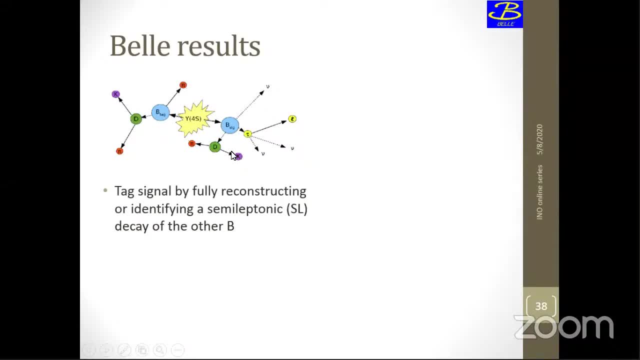 So tau to mu neutrino neutrino, for example, and you have a D And then on the other side you fully reconstruct the hadronic B decay. So that allows you to see that there's significant missing energy here, all coming from neutrinos. 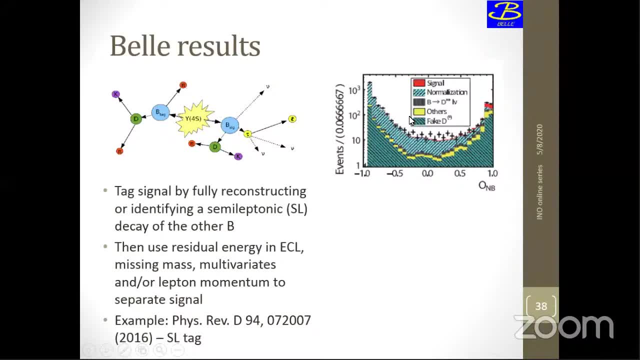 And you can use both multivariate techniques and then combining that with how much energy you see in the calorimeter, Events that are truly all neutrinos to giving the missing energy will have very little calorimetric activity And you see a peak of the signal down here towards low values of energy in the calorimeter. 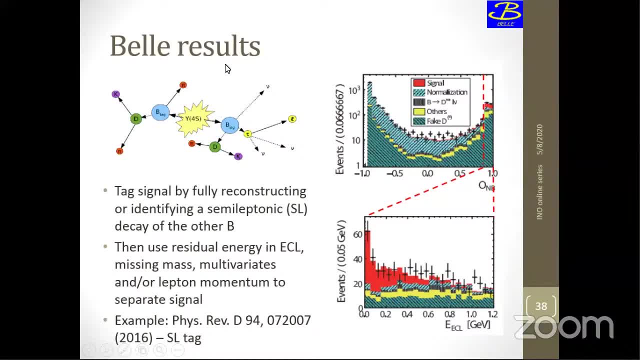 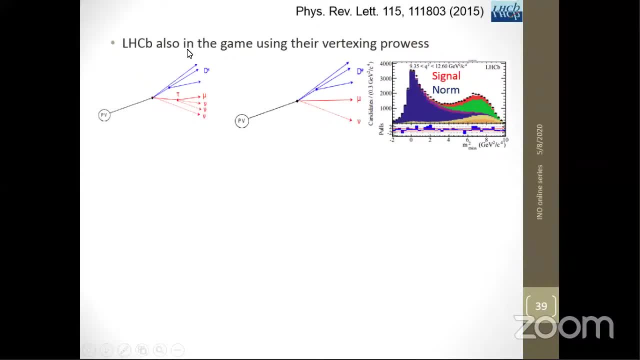 And this is how we saw these decays. This is a BEL, But of course we're limited by the statistics that are available, So I'll skip over. But LHCb can also do this, But they have huge backgrounds in doing this, much higher backgrounds than the BEL measurement they have. 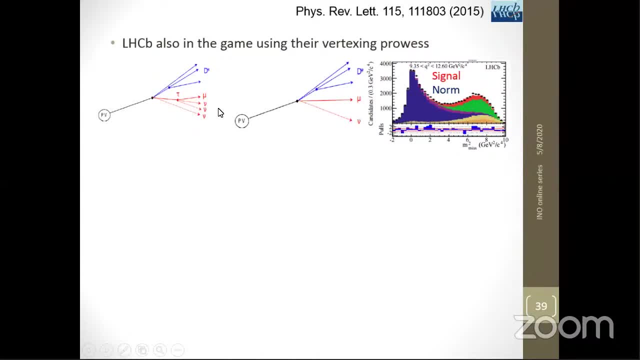 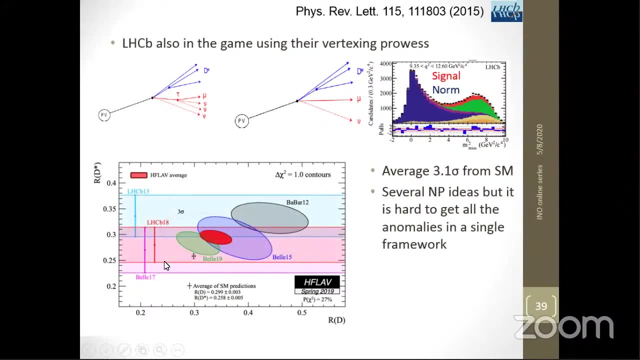 This is a signal in red here over a huge background, So it's very difficult for them to do, But they have tremendous vertexing so they are able to do this. But moving to the results now with BEL and ABAR and LHCb. 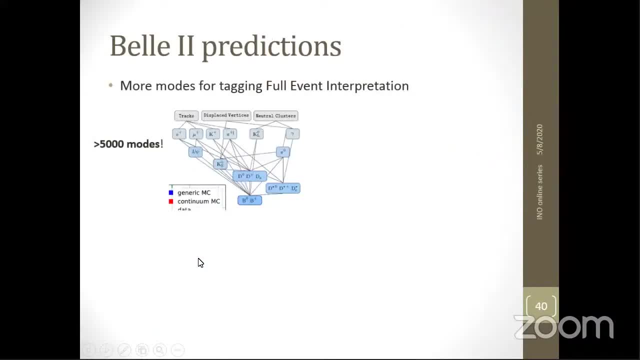 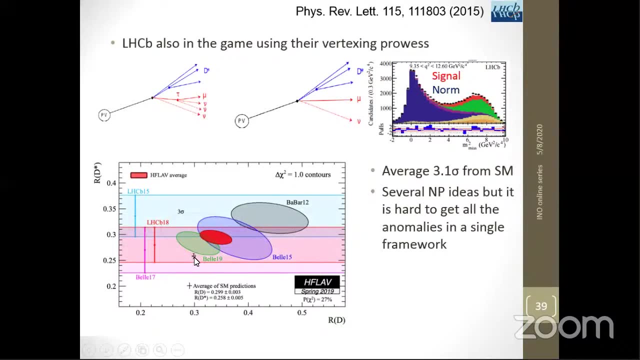 If you look down here, this is the standard model prediction for this ratio: RD and RD star. RD star on the vertical and RD on the horizontal axis, And red is the current world average And there is just over three standard deviation difference between these. 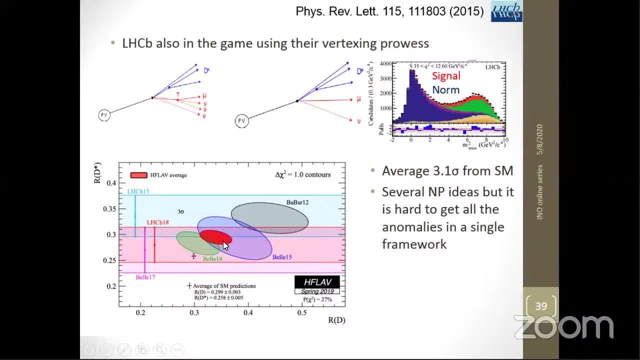 So the standard model is incompatible with the measurements at three standard deviations, And only more precise measurements of this RD and RD star parameter will be able to resolve this and see if there is some exotic physics explanation for this. This is one of the few places where the standard model is not working fully as we expect. 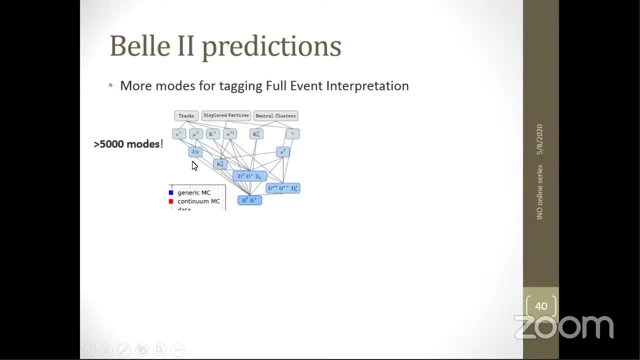 So BEL2 will do very well at these kind of measurements And they use this full-invent interpretation Where they reconstruct over 5,000 different B decays to get a very pure sample of hadronic B decays on one side, For which you can look for these rare decays with lots of missing energy on the other side of the event. 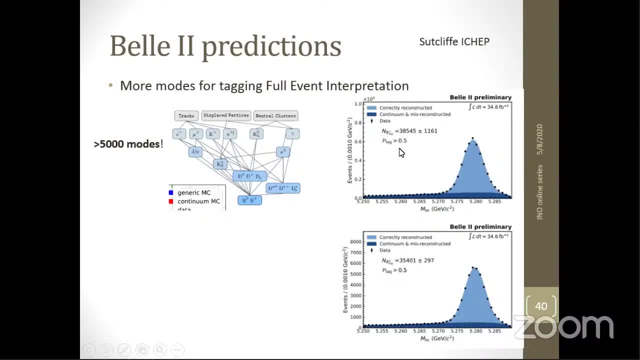 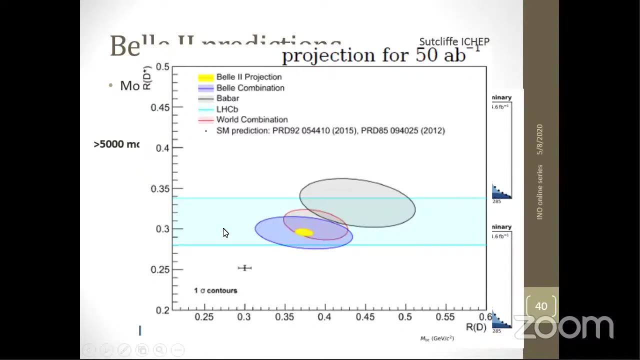 So these are plots from iCHEP showing that we've already got 40,000 of these tags for B plus and 35,000 for B zero, And one expects that this is with 50 inverse atta bonds. You get this very small region allowed from the measurements measured very precisely. 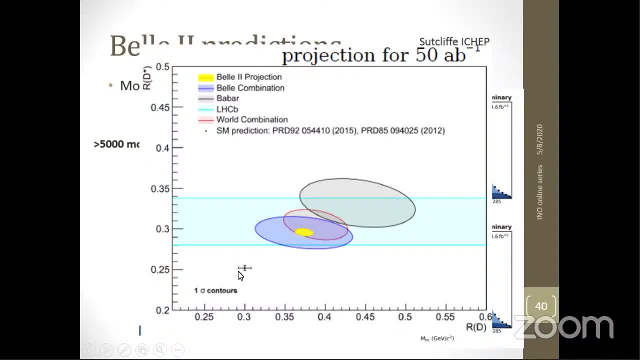 But even with five inverse atta bonds, we'll be able to tell whether there is a significant difference between the standard model and what we're observing, And this would be a clear signature of new physics if we see this. So there are many other measurements. 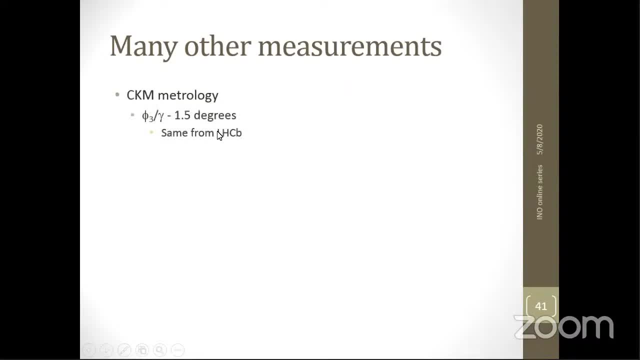 This is my penultimate slide. now We can determine the other angle of the unitarity triangle Particularly gamma Very precisely to around one and a half degrees. This is competition with LHCB. They are also making precise measurements. You can measure the length of the side. 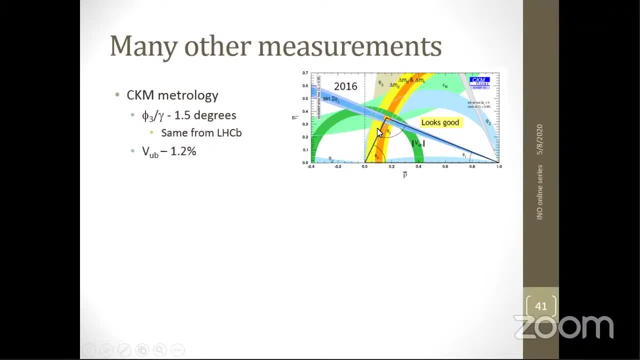 That's proportional to VUB And that will be done to around 1.2%. That relies on improvements in QCD as well. This is what we expect it to look like. Sorry, this date I should change. This is now nearer to 2030.. 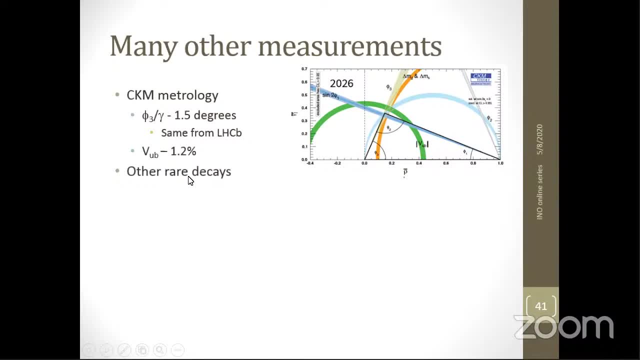 This is now nearer to 2030.. There are other rare decays one can measure. These are all given here. In particular, there's other lepton universality anomalies seen in these loop-only diagrams, these beta XS, LL, And we'll be able to measure those to a few percent to see if these deviations really are. 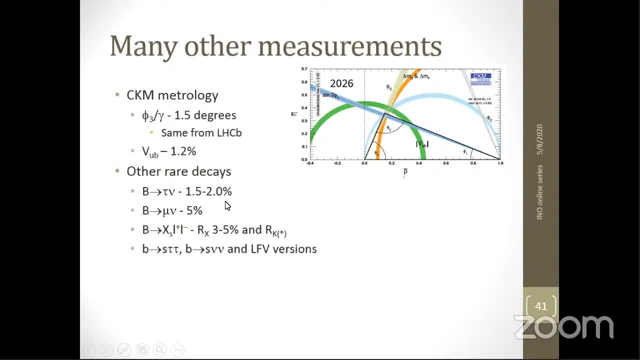 They're currently observed at the 20% level. whether they really are the result of new physics or not, We can also do more with neutrinos. here We can measure CP violation, again in loop-only processes, the so-called Galonic penguin. 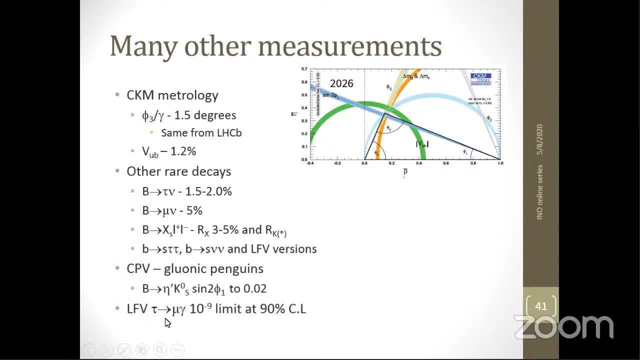 We can do very rare tau decays. I don't have any time to talk about this, but this is a very interesting area. You have this number violating decay, tau to mu gamma. We'll set the most precise limits on that And this is an example of tau decays in our early data showing excellent data. Monte Carlo agreement. 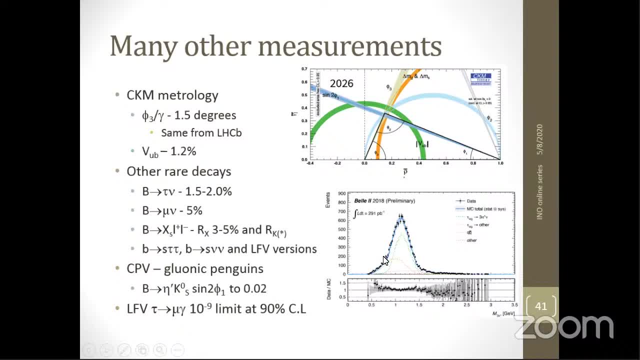 This is the pseudo mass of the tau decay. So we're already producing many taus and studying those. And there's also this QCD, a charm physics, QCD physics and dark sector, which I haven't talked about: certain regions. We can look for dark matter. 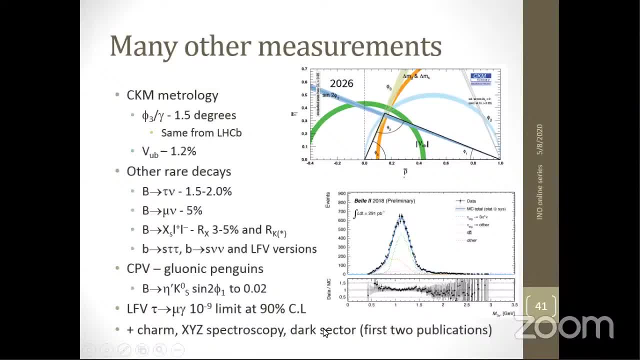 We can look for action like particles. We can look for dark eggs and dark photon And there have been already two publications- Sorry, not publication- One publication and one submitted for publication. But that's talk for another day for the dark sector. 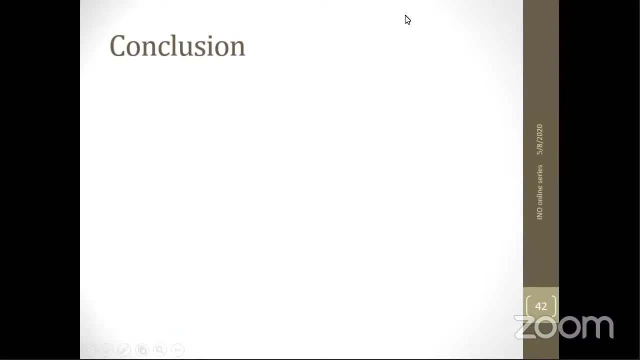 So I'll conclude now. I've taken an hour of your time. So intensity frontier is a very active area And Bell 2, the first Bell 2, and Super Keck B, the first high energy physics collider experiments since the LHC, are really leading the way in terms of the intensity frontier. 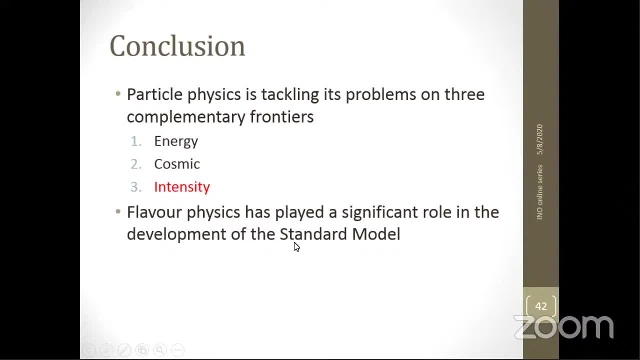 And flavor physics has played an important role in developing the standard model, The fourth quark, third generation heavy top, And there's no reason to think that they might point the way for us to look at physics beyond the standard model by making these precision measurements in the flavor sector. 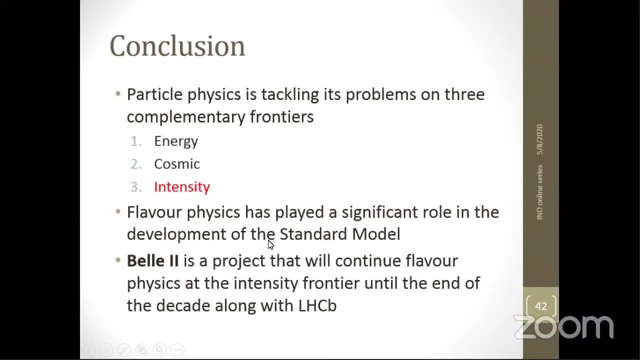 So, along with LHCB, we hope to be continuing the tradition of learning more about the standard model and particle physics in general from from these precision measurements. So thank you, I'm done. Thank you very much, Zim, for your really excellent talk with nice pedagogy that you kind of started off. 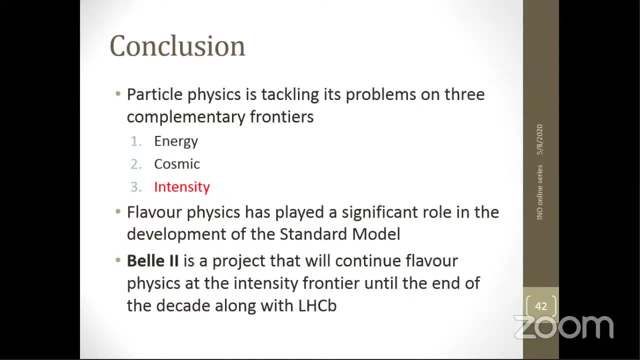 And then, of course, both at some point and also as the talk went on, you made an excellent comparison of capabilities and results, or the you know USPs, I can say, of the LHCB and Bell 2.. And very nicely, you have actually brought out the developments or the upgrades in the accelerators and briefly on the various detector upgrades for the Bell 2 compared to the Bell experiment. 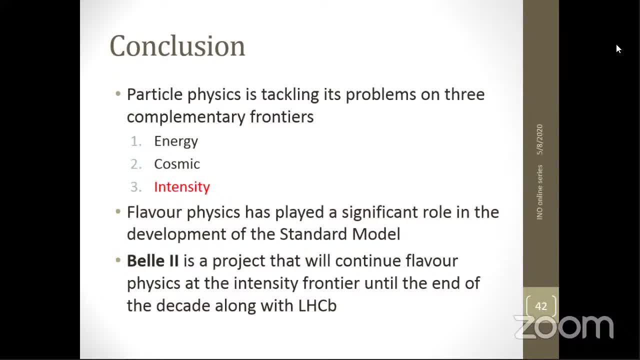 And what is, of course, very much heartening to many of us on the call is very significant: The Indian contributions that were made, Both on the detector developments, as well as the physics that you have shown, including those results which are really fresh from ICHEP. 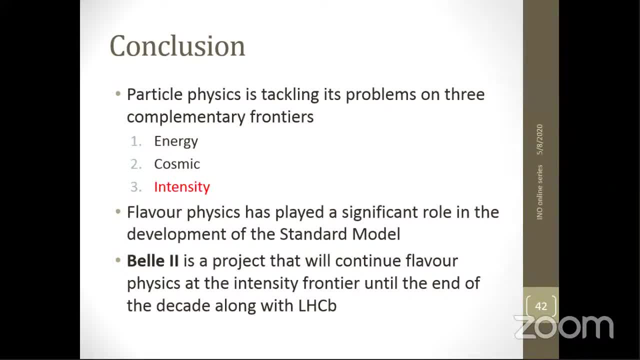 Yeah, particularly the SVD, I think, is feathering, I think the Indian collaborations cap, I must say. And so congratulations to you and your colleagues, And also I mean you brought out quite a few, Thank you. 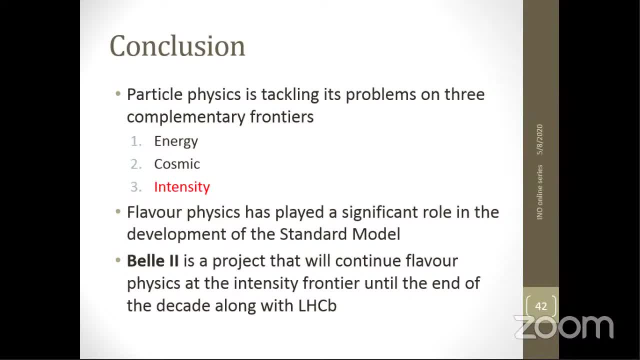 Quite a few future prospects and the physics that is waiting to be done at Bell 2.. And as, hopefully, your luminosity you're able to kind of increase with time, with additional components both on the accelerator and the detector. So you know, in all, I mean it was very nicely pitched for the participants, I guess. 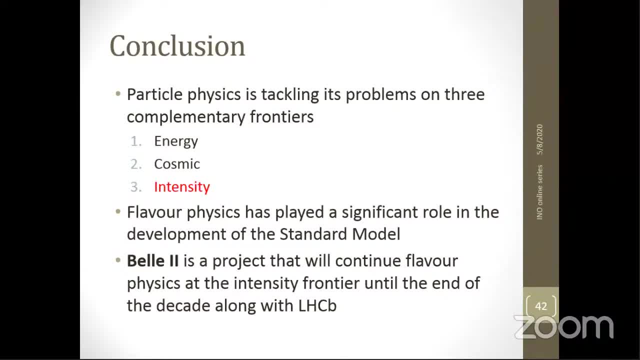 And I'm expecting that there will be visible discussions. So let me not take too much time except to thank you on that. But we'll get back now. We already have some questions, So let me start from here. Silesh Pincha has a question for you. 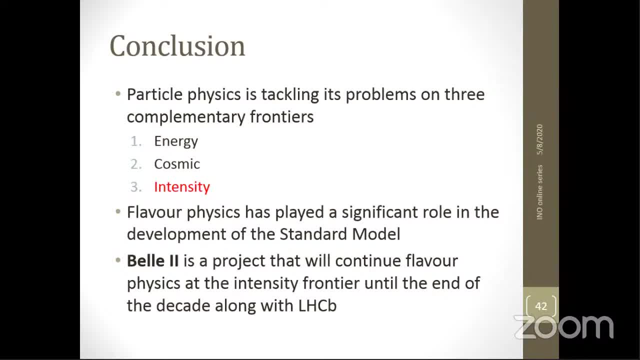 Hello, Yeah, Hi, Yeah. So my question is: just like there is a possibility that, due to the sterile neutrinos, the current three cross three matrix in neutrinos, the current three cross three matrix in neutrino sector is nonunitary? 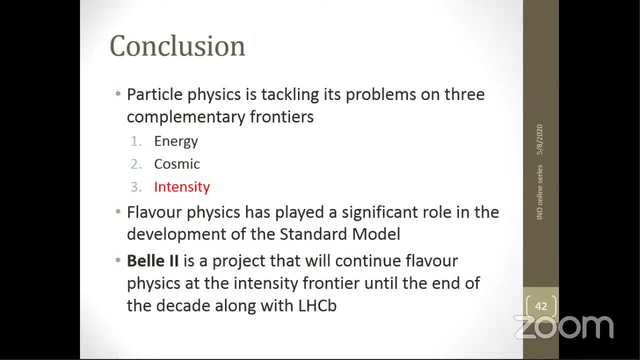 So is there the similar possibility in the quark sector that the current CKM matrix may be nonunitary with the possible fourth generation quarks? So that has been put forward as an idea over the years that there might be a fourth generation. However, 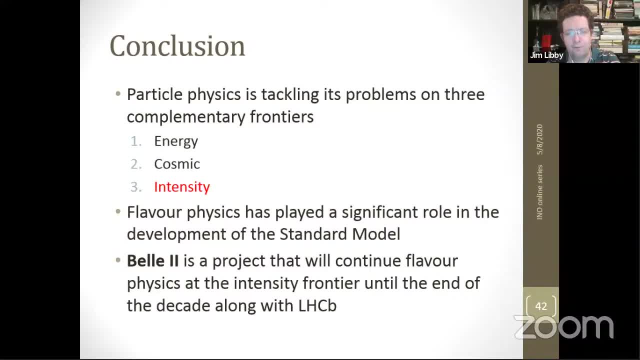 current measurements are such that the fourth generation is not particularly favored in terms of a model of new physics, say, to describe what's going on. These particles wouldn't be sterile in the same way that you're thinking of. Yeah, that is true. 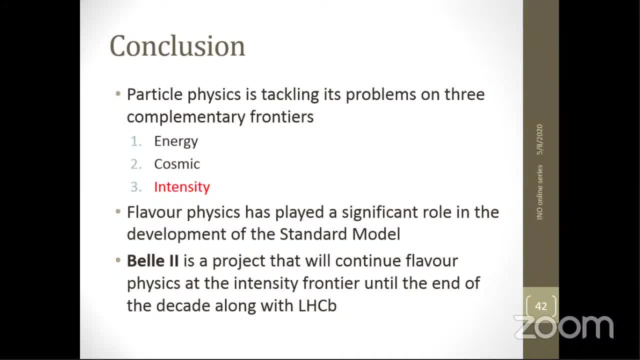 Like they will most probably be charged, So they will definitely interact electromagnetically. Yeah, So how they can hide is by being very heavy. Yeah, Right, So it's possible. there are additional particles that follow some generational scheme, but at very high masses which even we wouldn't be sensitive to. 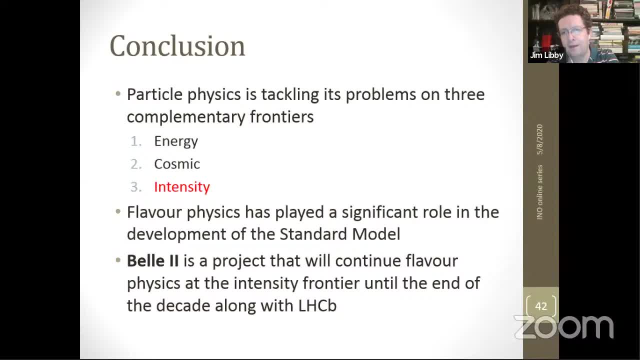 But in principle you're right that it's there. It's a possible extension, But it seems unlikely. For example, there aren't any fourth generation models That describe the B anomalies, for example. There that's very much lepto, quarks or similar things to do that. 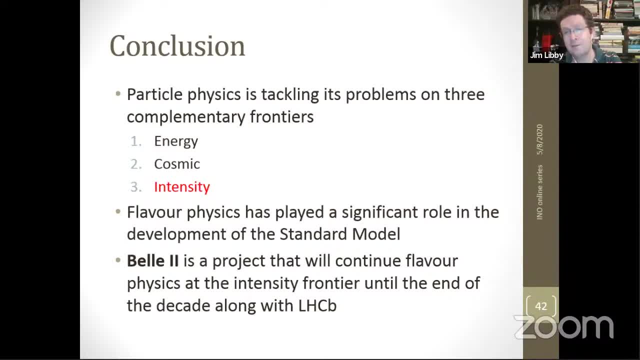 So, or additional gauge symmetries, So Z primes, and those kind of extensions of the standard model rather than the fourth generation. But in principle there's of course there's nothing to stop it, But you would have to put it at very high mass to stop it. 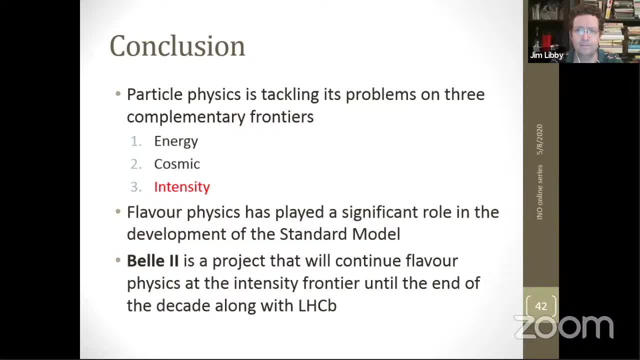 So that's one of the really disturbing measurements that we've already made. Thank you, Okay, There's one question in the YouTube by Abhinav Chaudhary: Why do quarks have flavors, with each flavor having different characteristics, and why they switch into one to another? 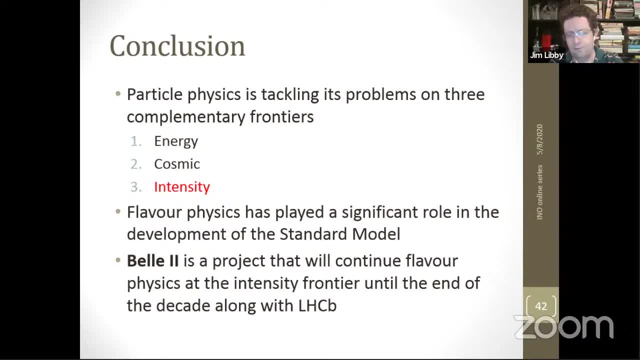 Um, So Yeah, The why is a good reason, A good question. I don't think anyone knows exactly why flavor allows this. that you can move between the generations- Okay, That's just. it's feasible through the CKM picture, But it could be like the lepton sector where that's not possible. 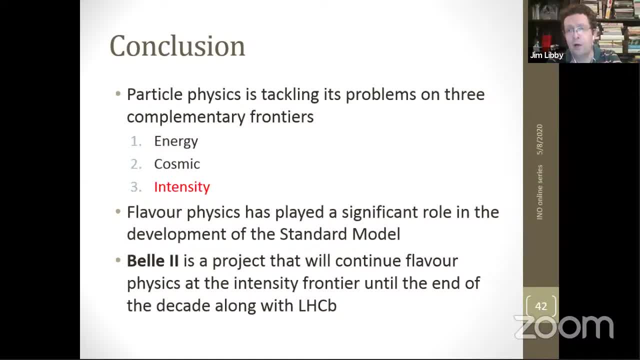 Right That, naively, It would look like the leptons, where you can't change between generations. Yeah, So This, This idea of flavor, Right, It's just a way of labeling the different types of quark. So Isospin is the original flavor. 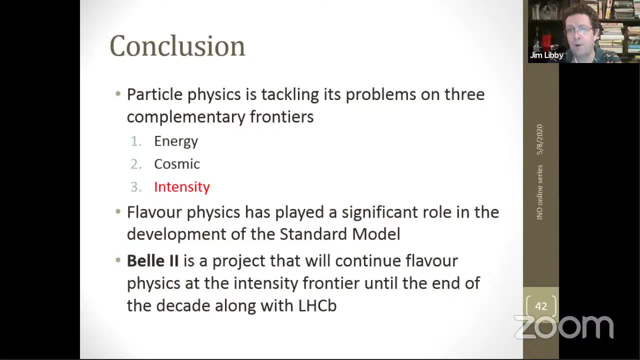 Where you Plus A half Is giving you an up quark Upness Minus A half Downness. Okay, So It's saying that these are Quarks, But they are of distinct types. So 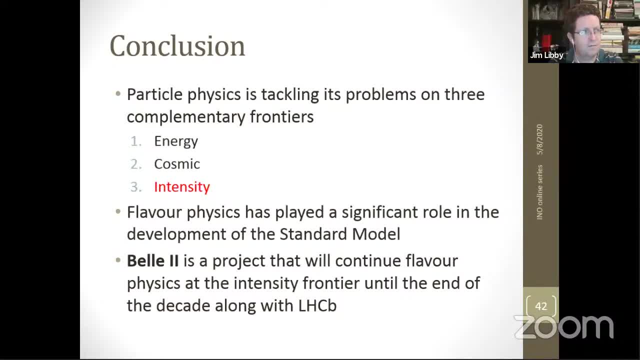 Um, It's, It's Just a way of Of Of Of saying that there is more than one variety. Okay, So we have six varieties or 18.. If you choose the different colors, And it's just a way of counting, 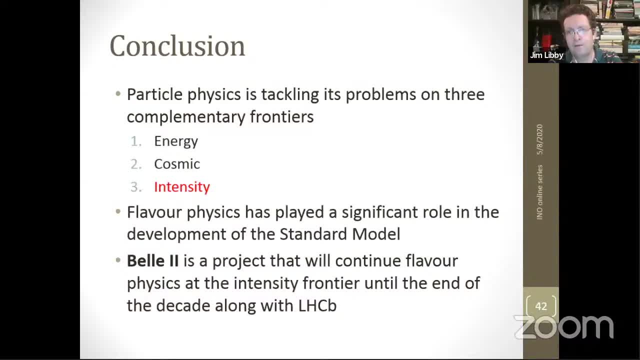 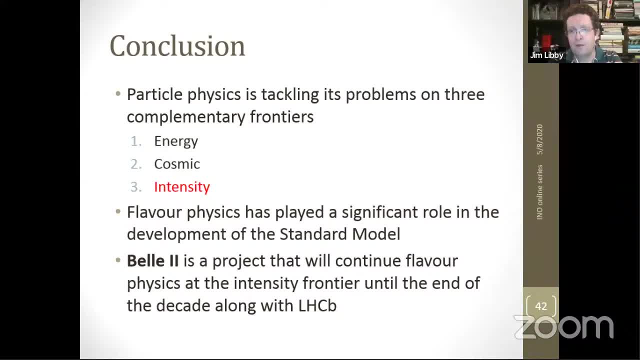 But the second part, Yeah, Um, That, that, That, That, That That ability to change is what makes The weak Interaction so interesting, that it's the only place in the standard Model where we can Change Between generations. 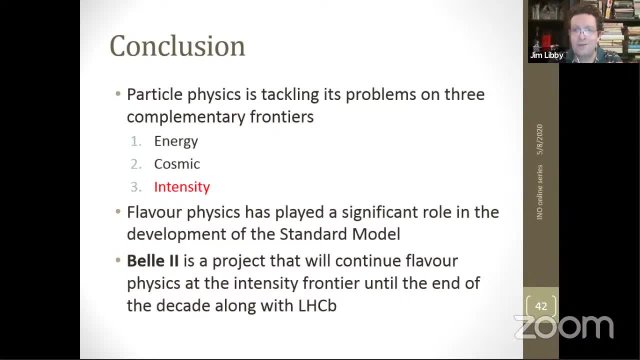 Otherwise, Heavy particles Would have been stable without New Physics. stable particles, or even beauty-stable particles of some kind, if there hadn't been this ability to then move between generations and decay to a kinematically more favorable state. Another one: what are the particles detected by electron-positron inhalation? 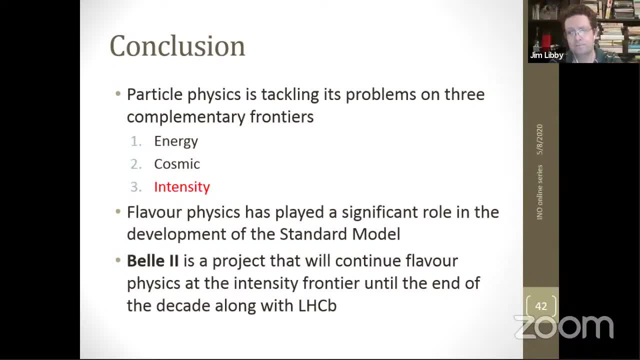 at Bell 2 experiments till date. Well, okay, So we? well, there are two aspects of this, right. There's one is that generally, we just reconstruct a handful of particles, the ones that we can, the stable ones, whether they be photons or K long. 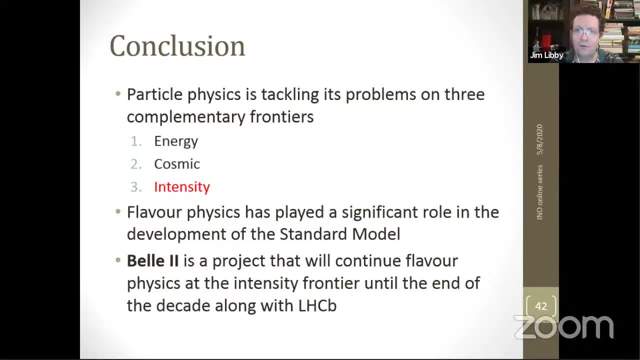 in terms of neutral particles or the electrons, So muon, pion, kaon, proton. Then from that we have reconstructed pretty much. well, you know, you look in the PDG and there are all sorts of possibilities for your mesons. 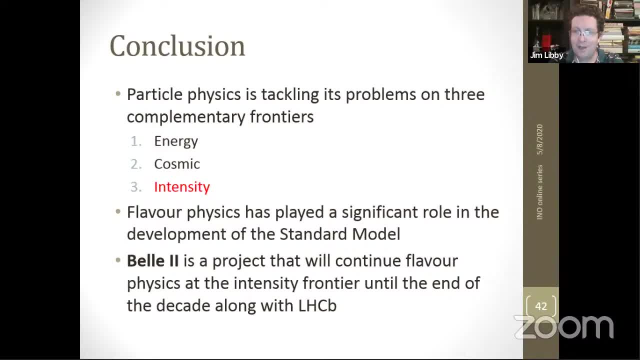 that are made up of charm, strange and up-down quarks. So it depends. It depends what we've seen: many, many things: DS, mesons, D0, mesons lambda C came at the ICHEP conference. We've also been looking for more exotic things, like the X3872,. 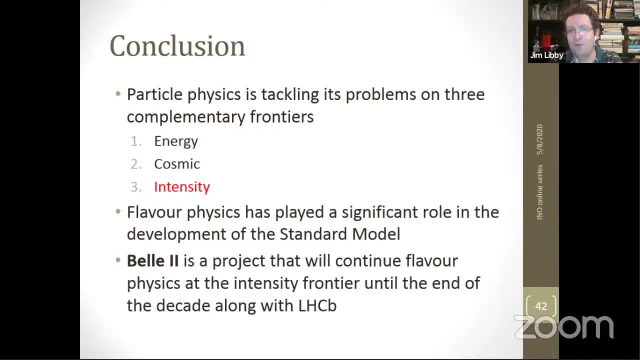 this charmonium light state. So we're seeing all the things we expect to see that have masses in the few GEV range. So we're looking at all those zoo of particles, Particles that are there. we haven't seen anything exotic. 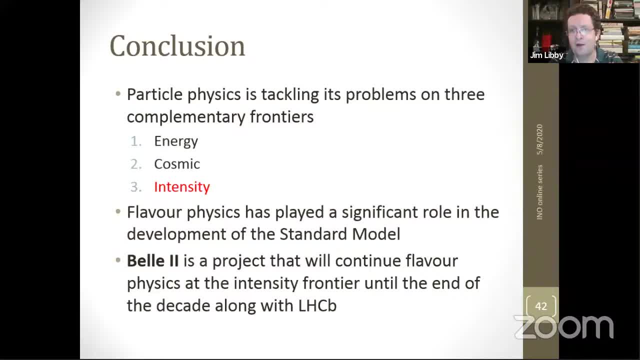 We haven't seen an alps-like particle and we haven't seen dark matter candidates, but those things that are there in the standard model we have seen. We haven't yet seen any signatures for exotic hadrons, but we've certainly seen J psi. 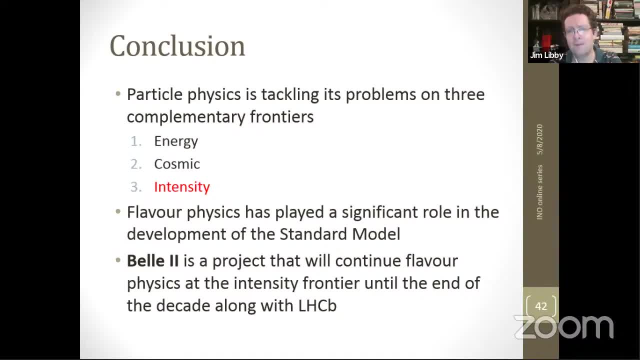 psi 2s, all the things that we expect to see. Okay, so, Jim, we have another a few questions or comments, So let us go to Bala Subramaniam. Hello, good evening. I'm Areeb. 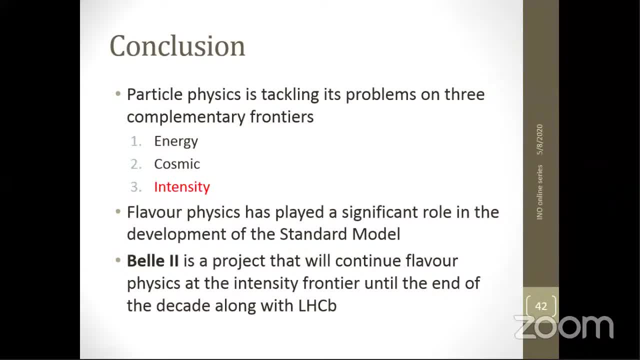 Yes, yes, Please go ahead. Sir, could you please tell us something about lattice QCD measurements on CK matrix elements? Well, I'm not an expert. Okay, I'm not an expert on that. However, maybe I'll just show a picture I showed near the end, which is helpful. 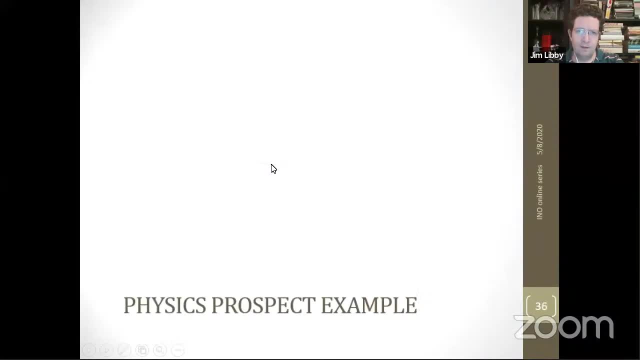 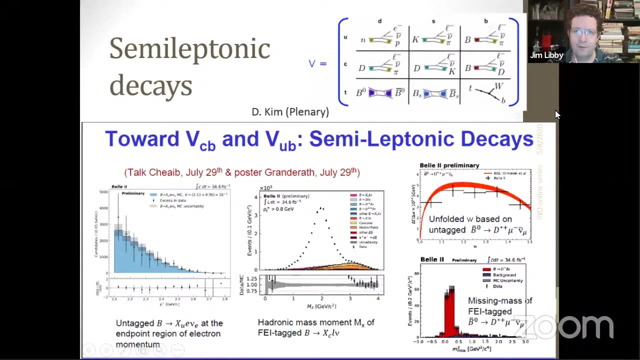 Here. So you see, we've written the CK matrix in terms of the different diagrams that are sensitive to the magnitudes. Okay, So you can see. you can see the color of the CKM. I'm not sure if you can see it. 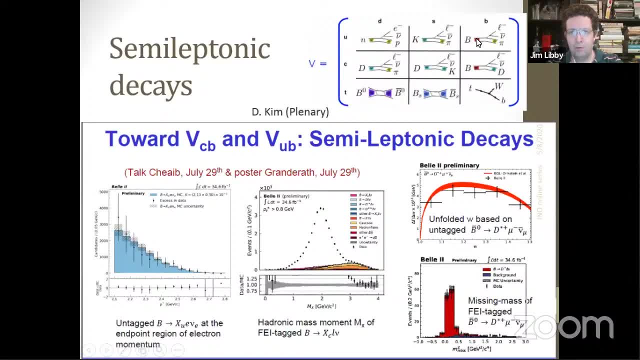 You can see it here. So these are the four different parts of the CKM elements. Now, where you see sort of fuzzy bits, whether they be yellow or blue or red, they're either showing you light quarks, charm quarks in blue or red. B quarks. 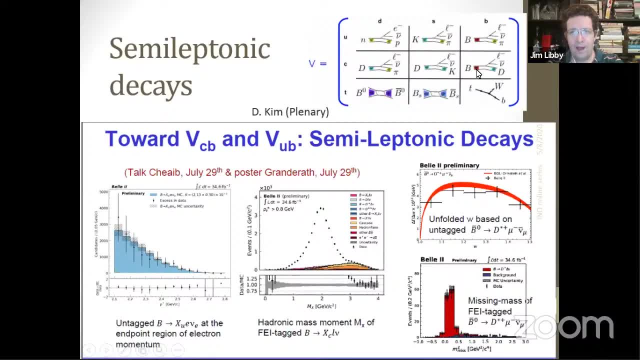 There is a lot of QCD going on, binding together the B meson or the charm meson interpret well these semi-leptonic measurements. you either have to do calculations in like cone sum rules or in some way in QCD, or you use lattice calculations to 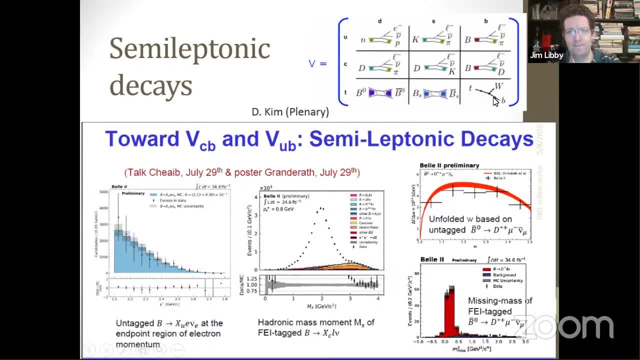 to determine the form factors that you have. so these form factors are often calculated by the lattice and then we compare them to the measurements and take out those, the contribution from the QCD, to get at the electroweak, the short range effect. Now these measurements are: 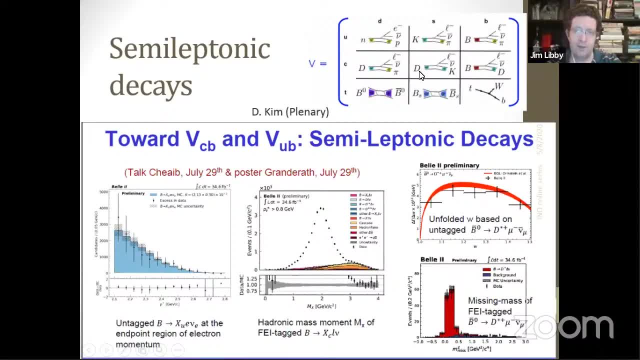 also done with charm decays, principally at the BEST3 experiment, and the charm measurements here are very useful to calibrate the techniques of lattice QCD so that you can then apply them to the QCD, to the B system to get more precise measurements of VUB, for example. so this particular decay B to 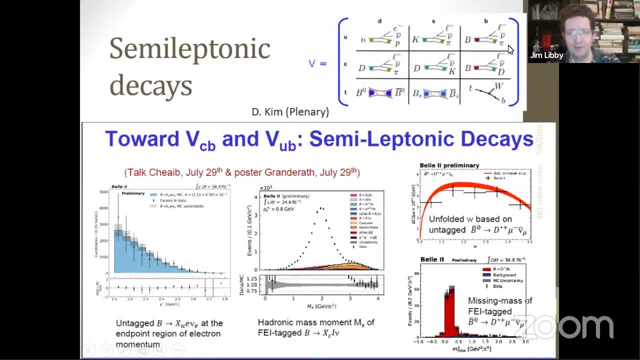 pi, LNU to get the lattice predictions for the B to pi form factors are essential to determine VUB, which is one of the big goals of um, of BEL2, but it also requires improvements in lattice QCD. so I whatever petaflop calculations or whatever people say need to be done as well to do these. 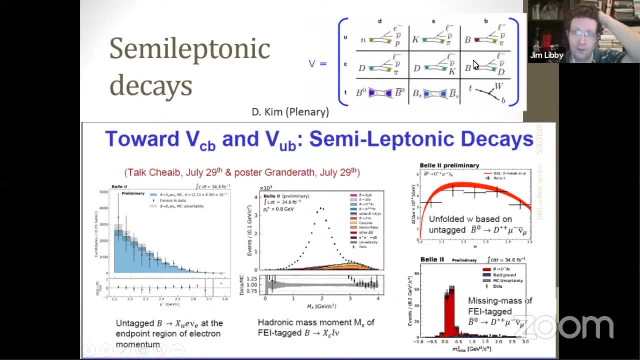 these, these calculations as as good as possible and and to do as realistic as possible, calculations with less and less quenched, calculations with more and more massive quarks, and things like this. so I, I, you, you really should talk to a lattice QCD specialist about this. it's it, it's a very um. 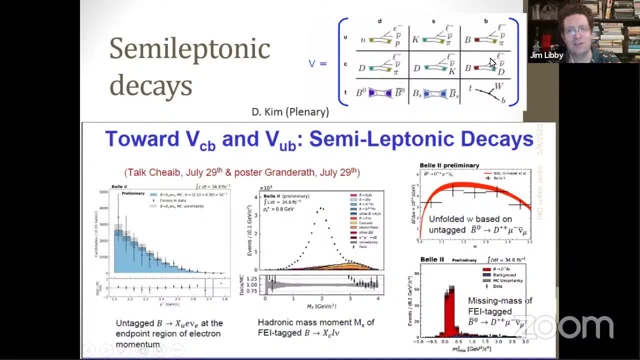 uh, yeah, you shouldn't, you shouldn't ask me too many details of the calculations, but they're exceedingly important for these types of measurements. Okay, yes, sir. thank you, sir. Uh, let me take a question or maybe comment from Gagan. Ah, can you hear me? 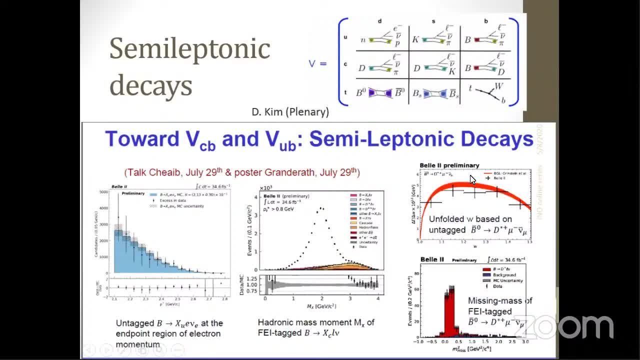 Yeah, okay, you can take over. No, no, no, I absolutely not. so anyway, I enjoyed the talk because there was this, um I I don't know from YouTube this comment: um, so you really said the half of the PDT, more than half, is basically the measurement from the flavor sector. uh, so indeed, we haven't seen anything new as uh. 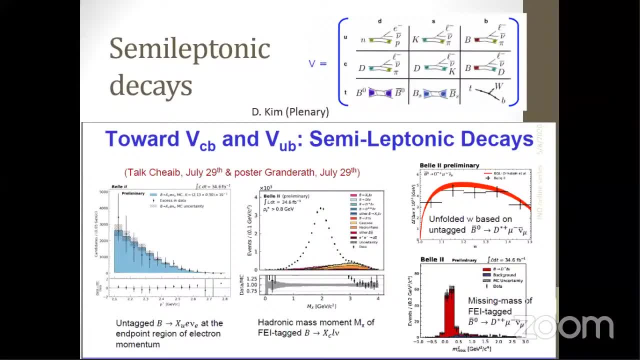 similar, like LSC. but there are some exotic measures uh, which have been seen by Bell and Barber, like this X3872 uh or the discharged uh tetrachlor candidate. I mean, they are not new physics. I don't know if the questionnaire is still there. 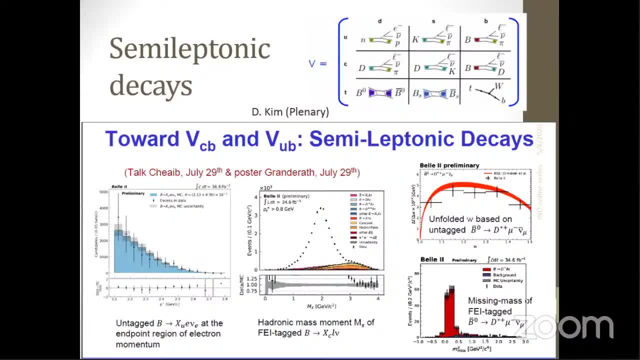 Yeah, But but the QCD, QCD, QCD people are still having trouble to really, uh, you know, fit in that with this what we call the standard quack margin. okay, yeah, so, but we haven't reconstructed them yet at bell two, right, I don't think. oh, was that in bear? okay, okay, that was in bell two was the question. 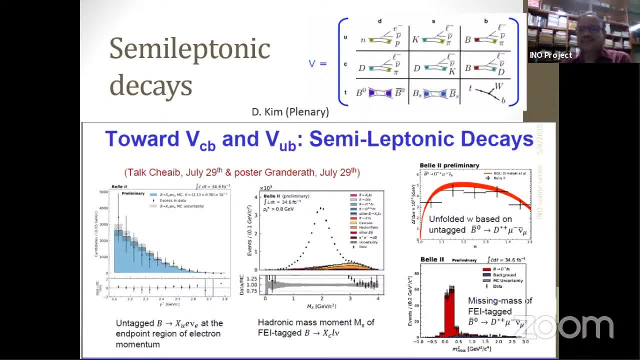 sure, in bell. yeah, he was asking for bell two. oh, okay, okay, sorry, yeah, yeah, no, no, no, but uh, nevertheless it's uh. thanks, Gagan, for actually uh pitching in and also adding up uh to what Jim has already said. I hope uh the uh. the participant got his answer. thanks for that. 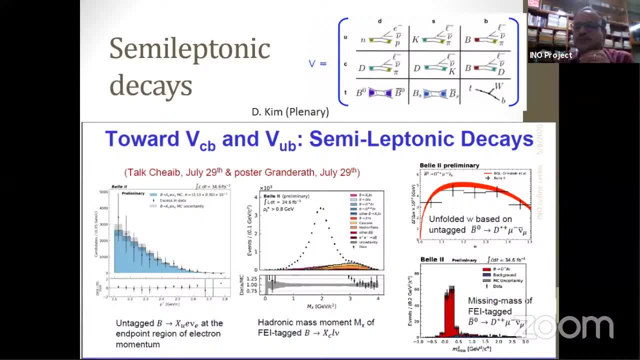 and uh, we'll also take up another question from Ashwant Prabhu. uh, good evening sir, uh, hello, yeah, how are you? I'm great, I'm great, how are you, sir? fine, yeah, so I just had a question. so, uh, bell and babar, these are mainly related to studying. 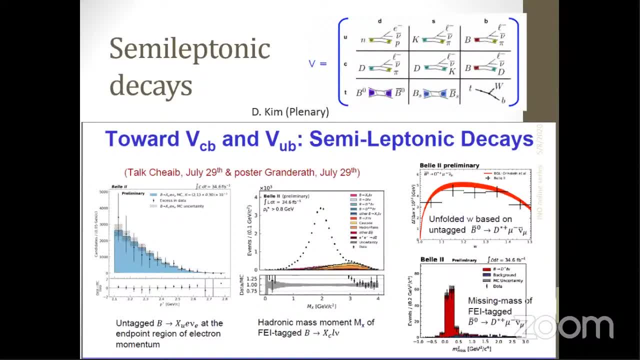 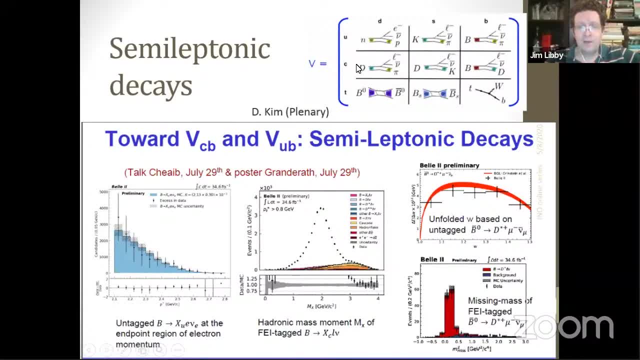 um, best three contributes in two ways really to CKM physics. one is by measuring VCD and VCS very precisely, and then the other is by measuring VCD and VCS very precisely in semi-leptonic d-decays and in fully leptonic d-decays. 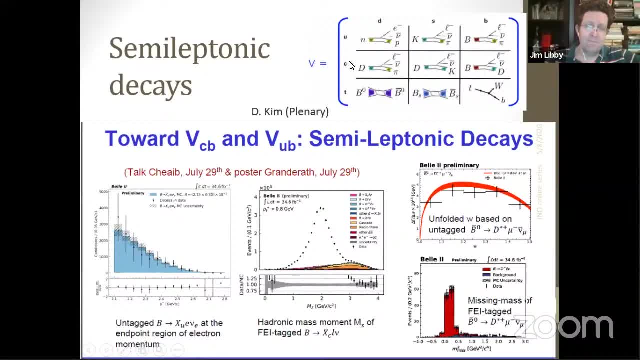 and the other way is less direct, but it measures what are called strong phases of d0 and d0 bar, which are essential inputs to determining Gamma in bdks. so these are the two principal contributions of best three to CKM physics: um and, and particularly in terms of the absolute size of um. 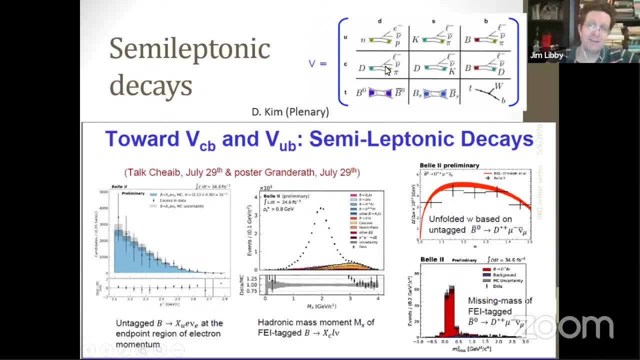 VCD and VCS. that's the best place with which you can measure these in CKM physics. and and because it's a charm threshold, it has the same um advantages as as bell two: that you only have a d, two d mesons. you have nothing else. 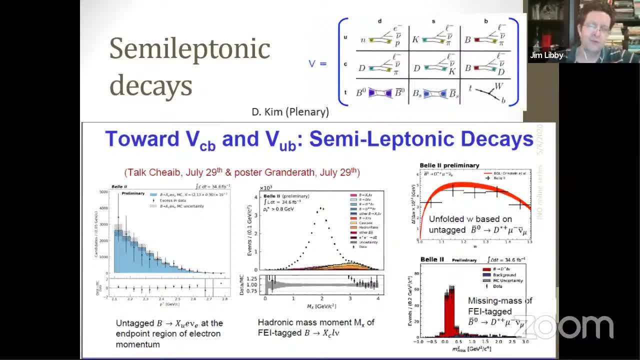 so you can fully reconstruct the whole event and you can make absolute branching fraction measurements and you can measure almost background-free measurements of partial decay rates. You can then test the QCD predictions for the form factors very, very well, And there's also a lot of other physics that's done in terms of measuring branching fractions. 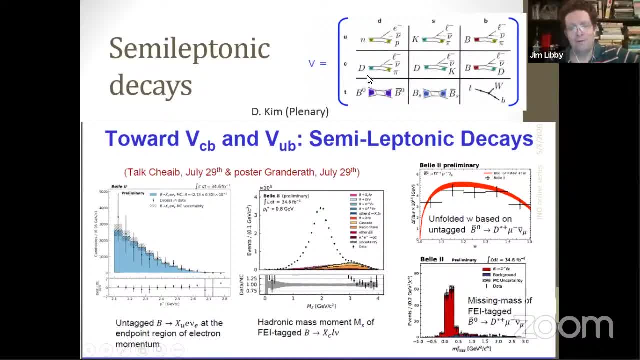 which again are important for flavour physics. So as an example, they also produce lambda C, lambda C bar pairs and you measure the lambda C branching fractions And those are used to normalise VUB measurements at LHCb, for example in lambda B. 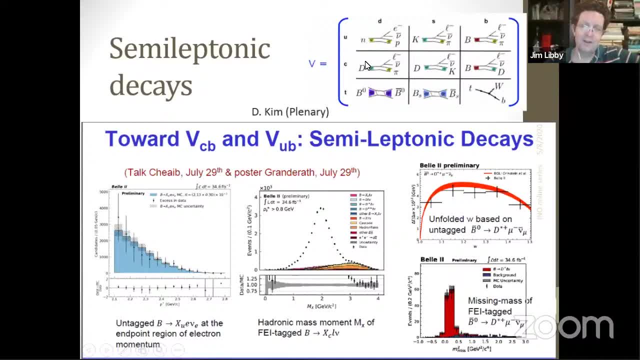 semi-leptonic decay as lambda B to proton. So there are all sorts of engineering measurements that are there as well, And then there's this direct contribution in terms of VCS and VTD. Thank you, Okay. So in terms of neutrinos, I think they will be very similar, isn't it?